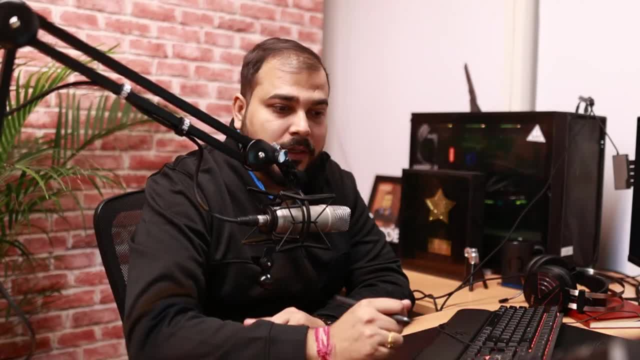 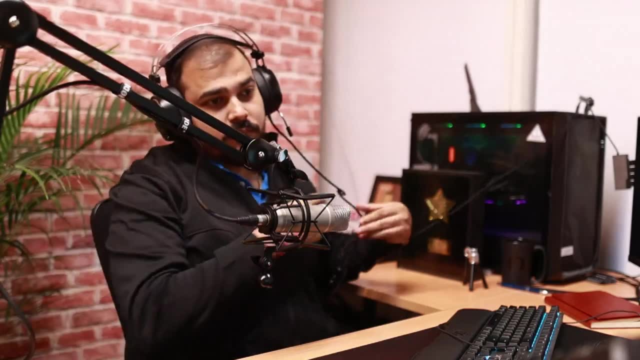 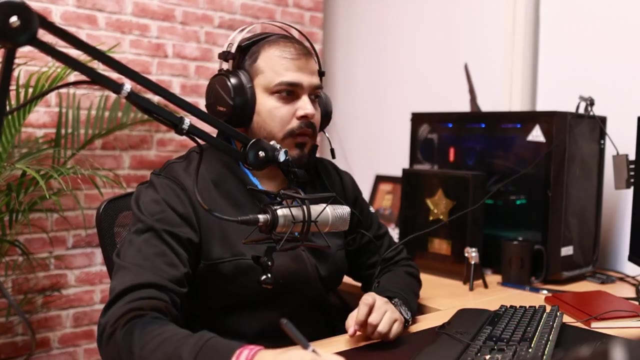 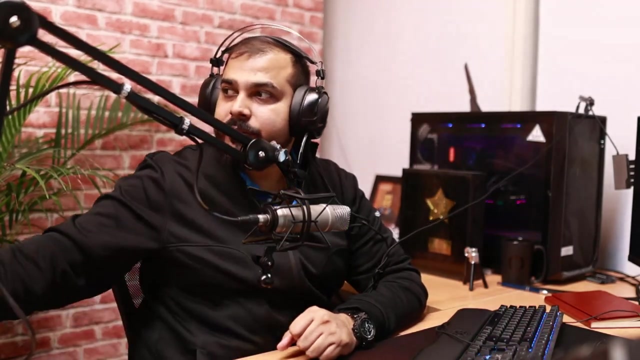 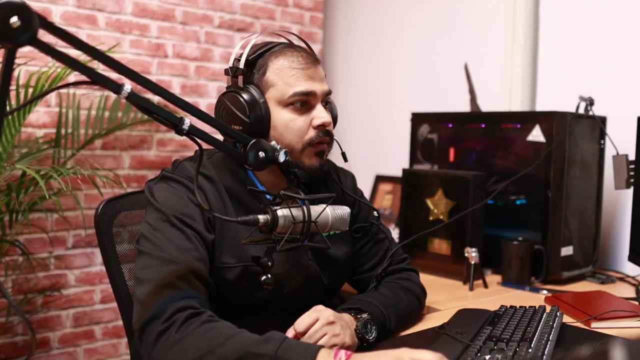 Okay, perfect, Perfect. So how are you all? I hope you are doing fine. I hope the NLP series is going on fine. Okay, so what? all things we have discussed in the previous session? Yeah, so what? all things we have actually discussed in the previous session. 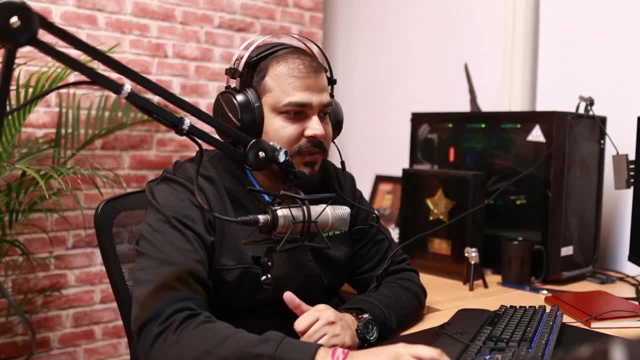 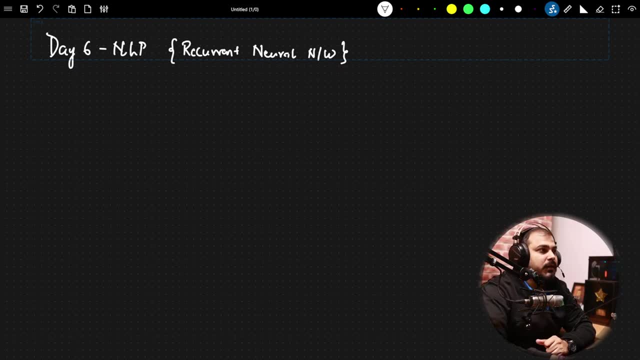 Can somebody tell us so that we can start doing things? So let me go ahead and quickly share my screen, and then we will just start. In today's session we are actually going to discuss about RNN, that is, Recurrent Neural Network. 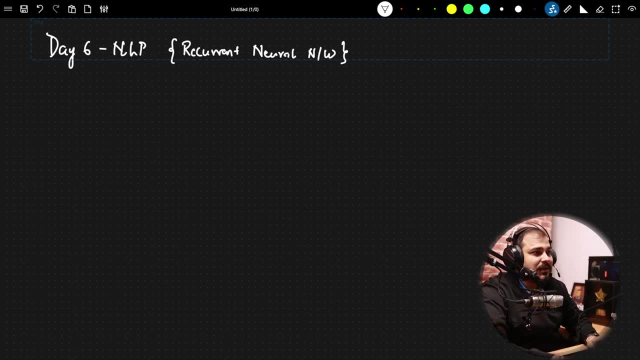 This will be quite amazing because we are going to learn some amazing things. now We are going from machine learning to, you know, deep learning, and here you will be able to do some amazing things right. So this will be quite amazing when we are learning things, and we'll make sure that whatever things we learn, we understand it and we do it practically. 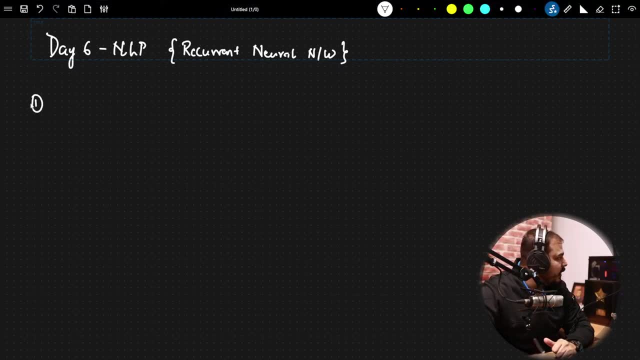 Okay. So in our previous sessions- let me go ahead and write- We have also learned about Bag of Words. We have learned about TF-IDF. Then we learned about something called as Word2Vec. Okay, Then we also learned about Average Word2Vec. 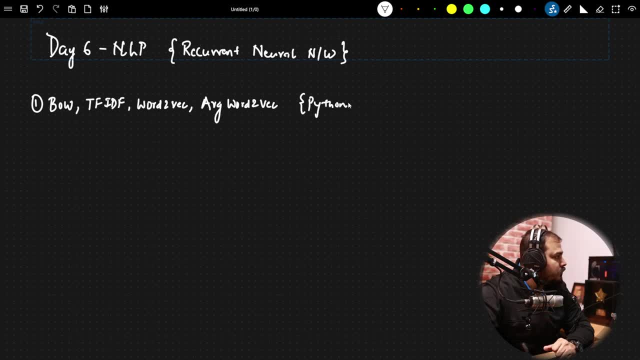 Right, All this we did with Python Practical implementation. we have completed this Practical implementation. Two architecture of Word2Vec we have seen. One is CBOW and one is NGG. Right, Sorry, N-scriptgram. Scriptgram basically is this: 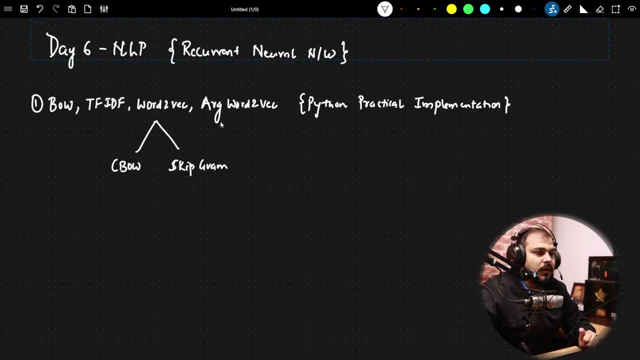 We have learned about these two architecture And now today, we are basically going to learn about one amazing thing, which is basically called as Recurrent Neural Network. Now we are moving towards deep learning. If you remember, from the first session, the graph that I have actually created, right bottom to top, 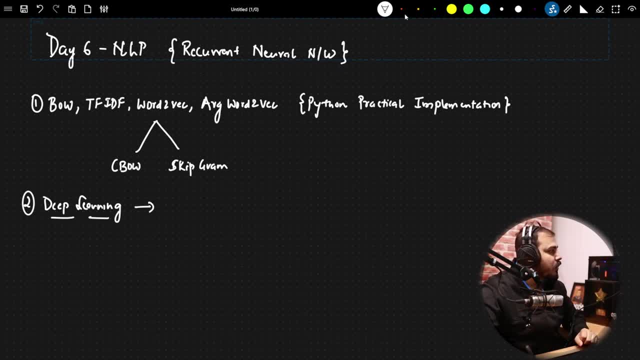 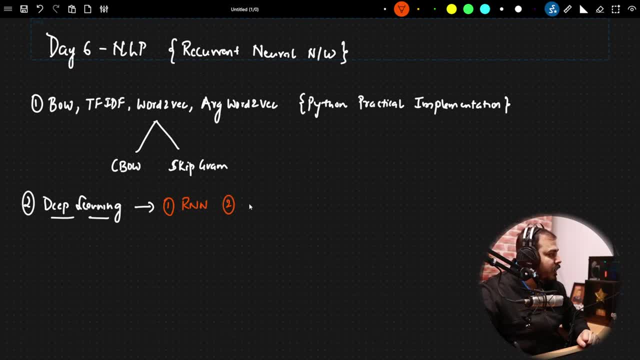 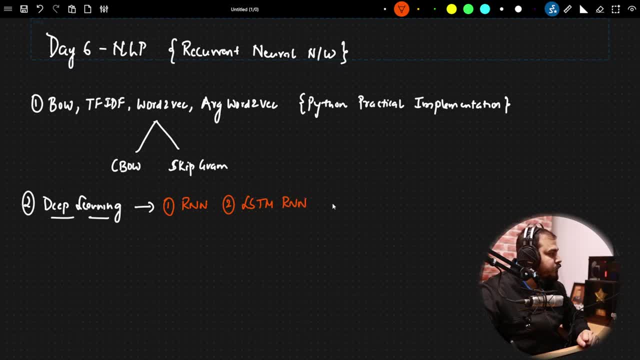 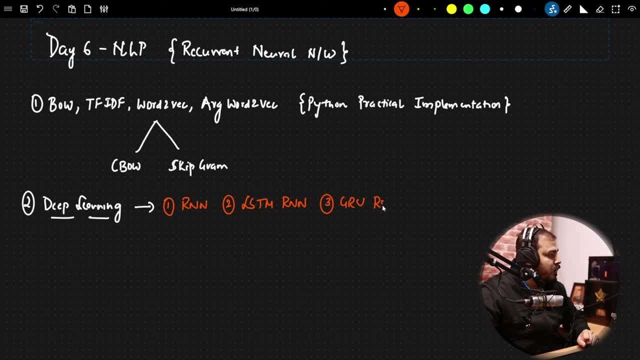 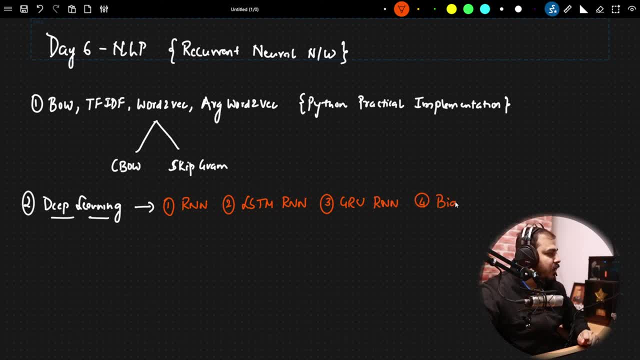 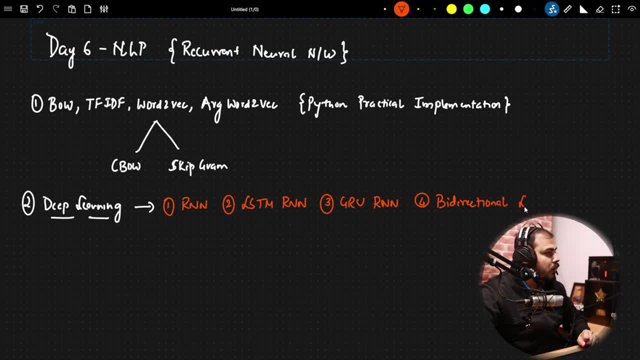 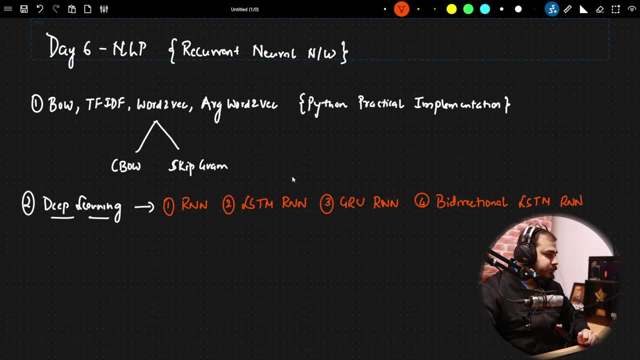 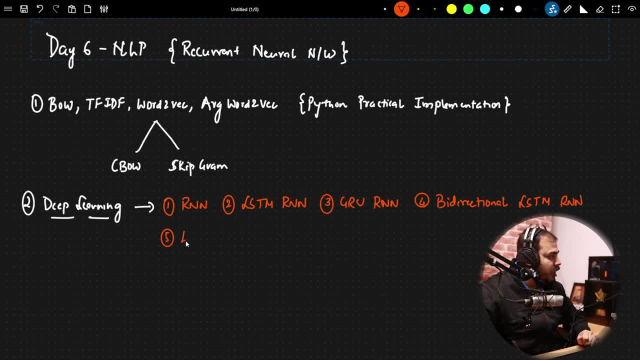 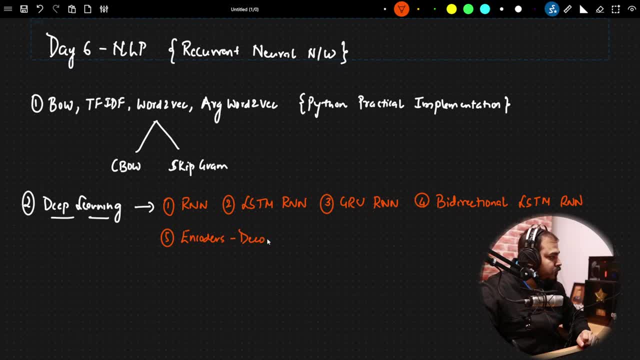 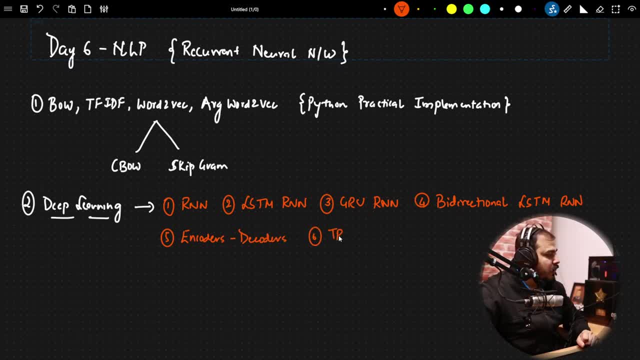 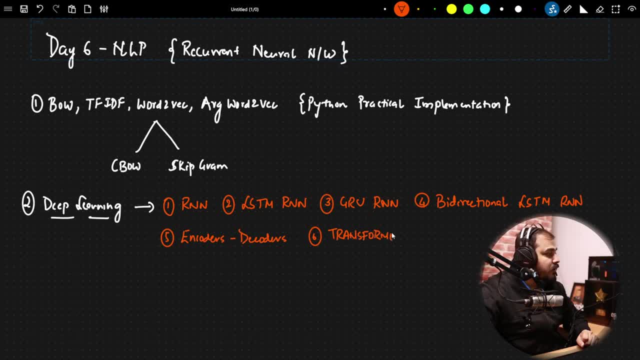 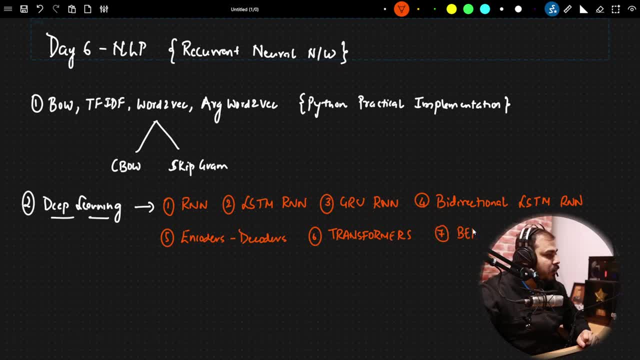 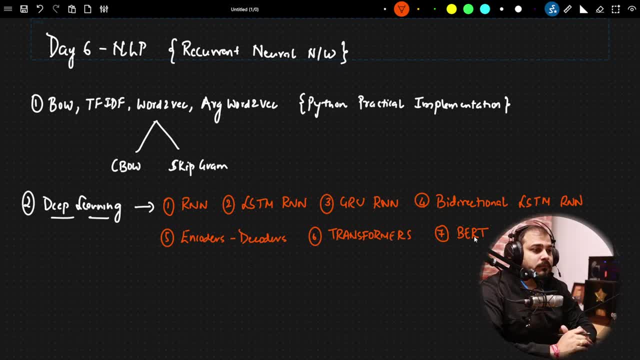 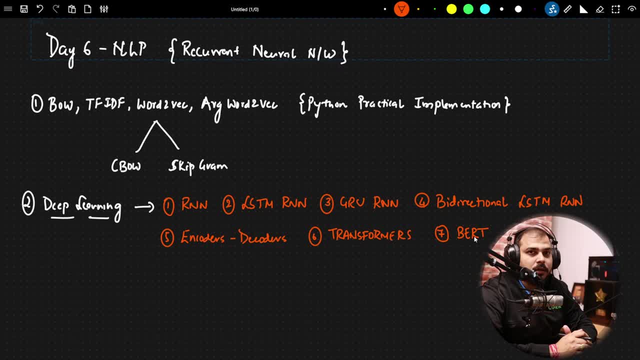 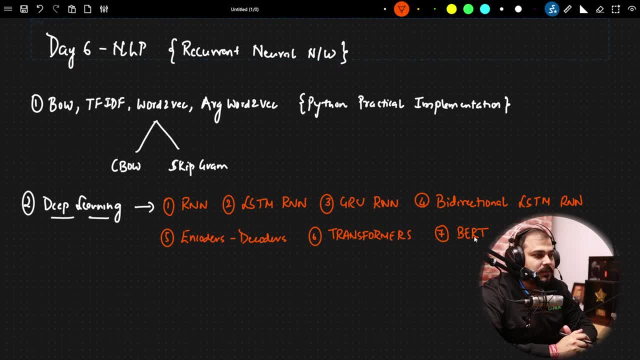 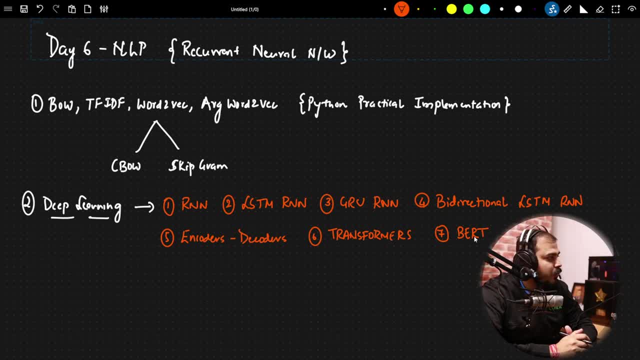 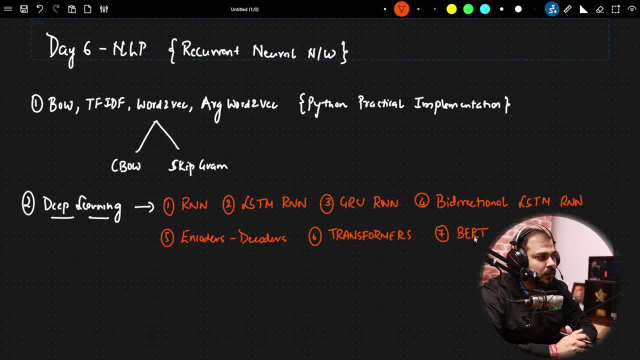 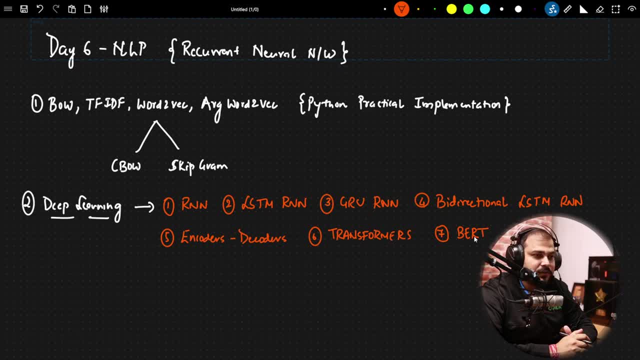 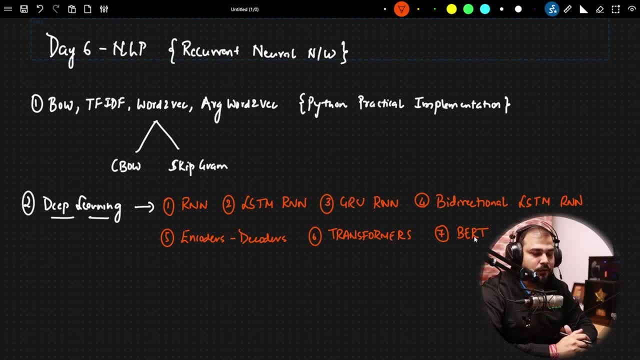 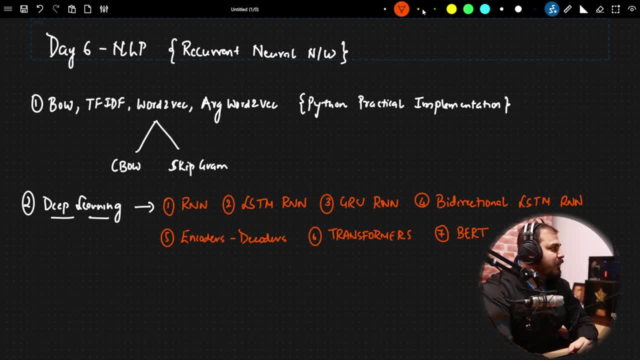 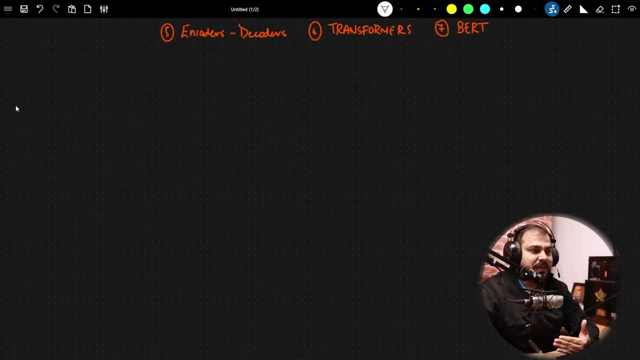 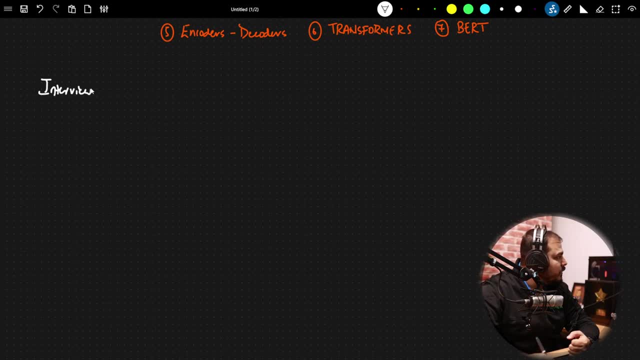 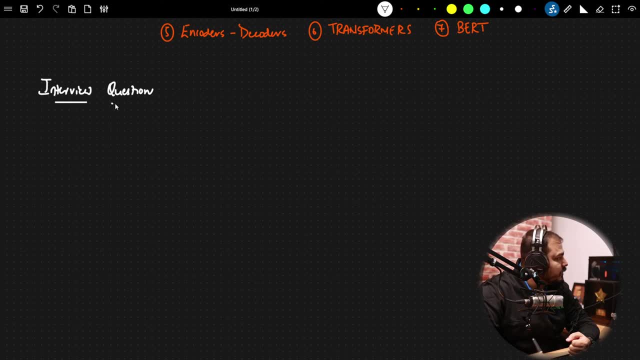 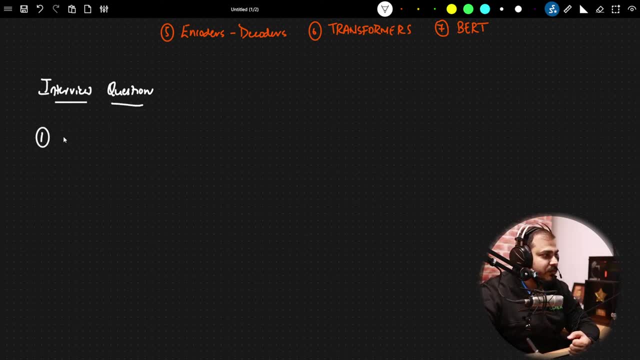 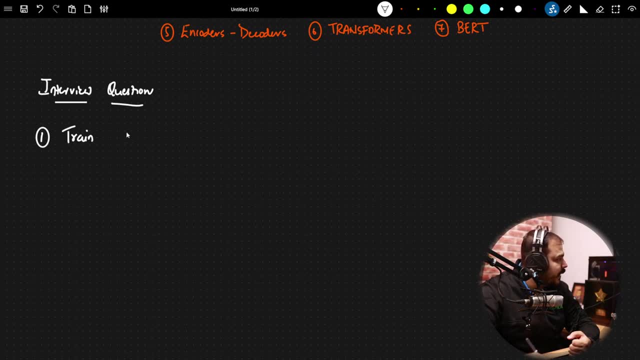 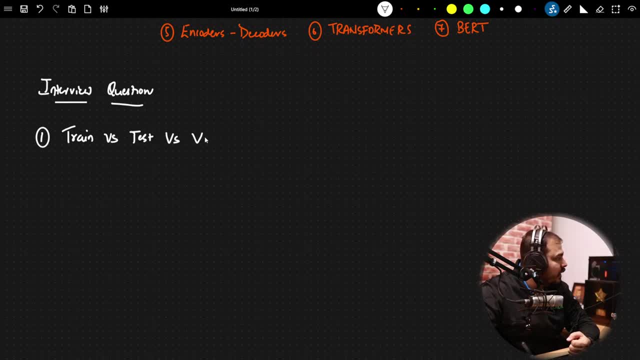 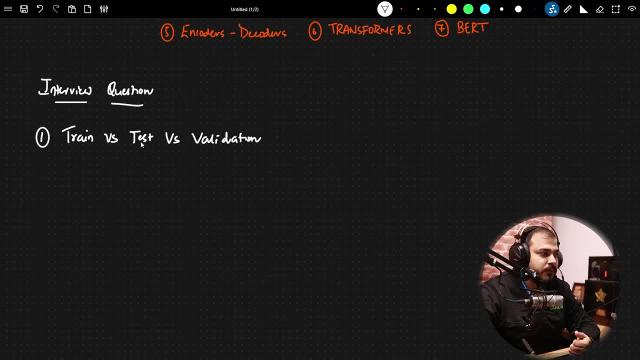 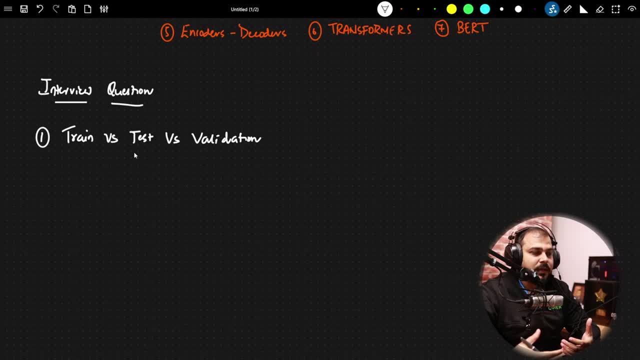 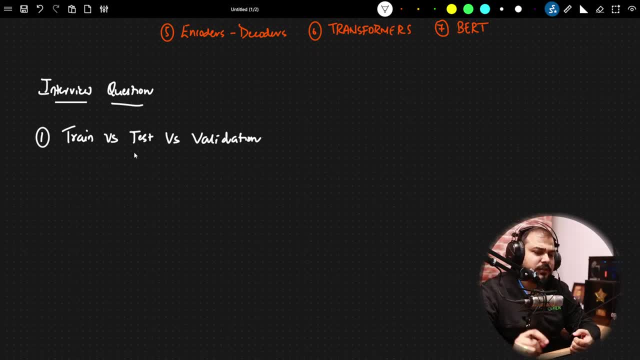 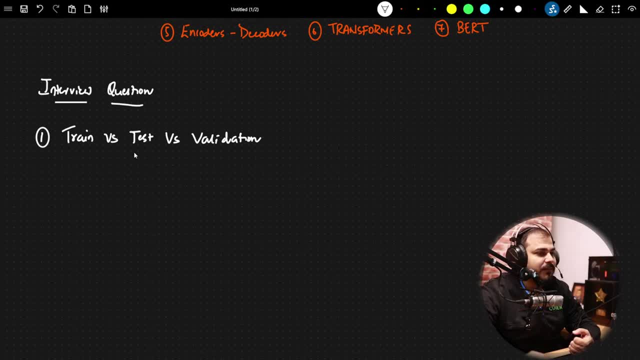 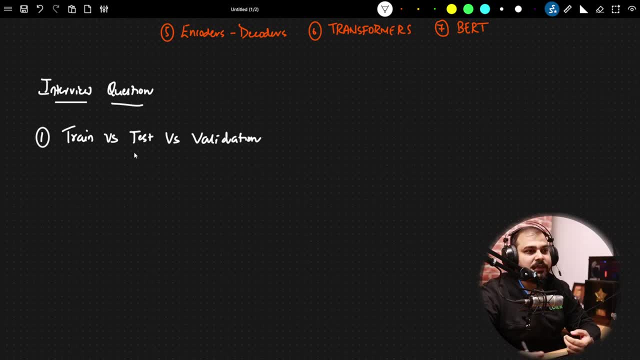 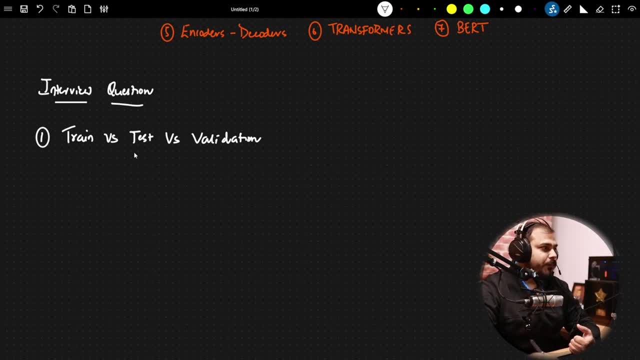 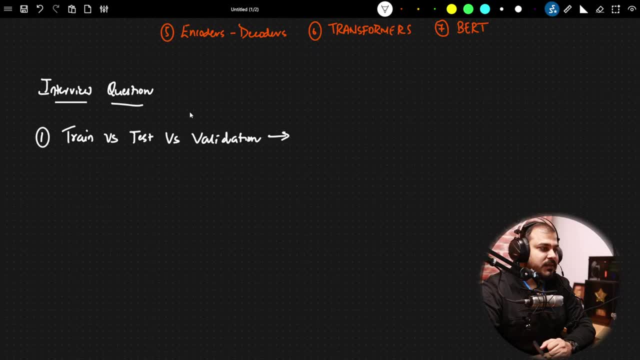 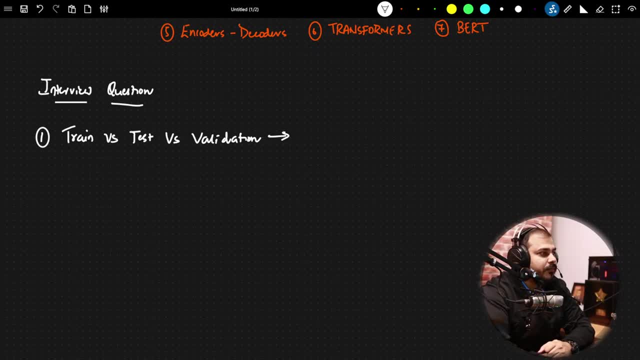 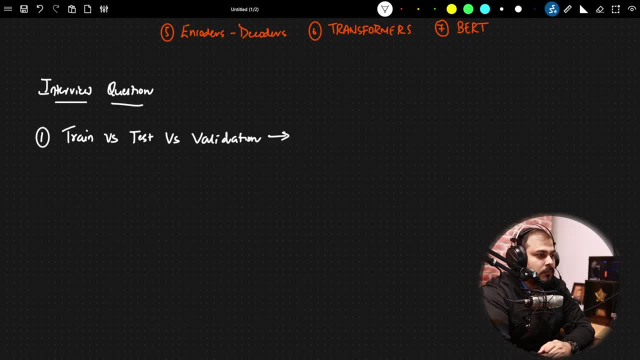 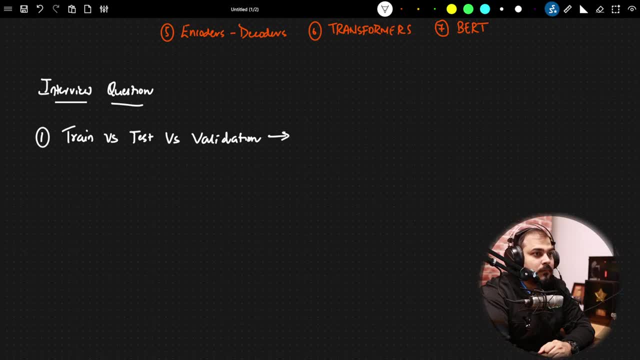 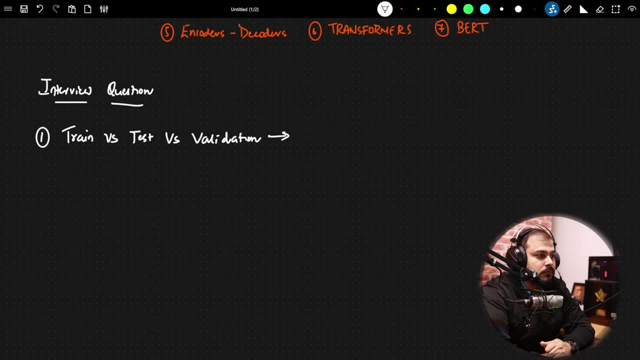 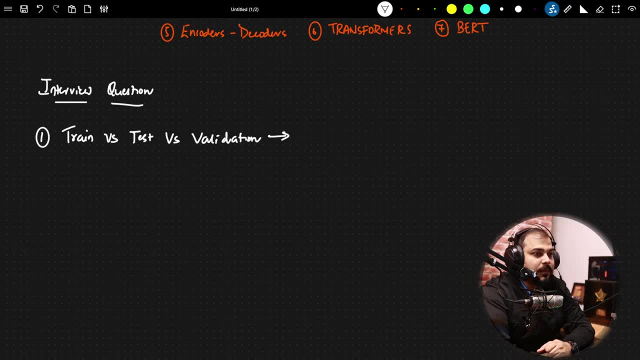 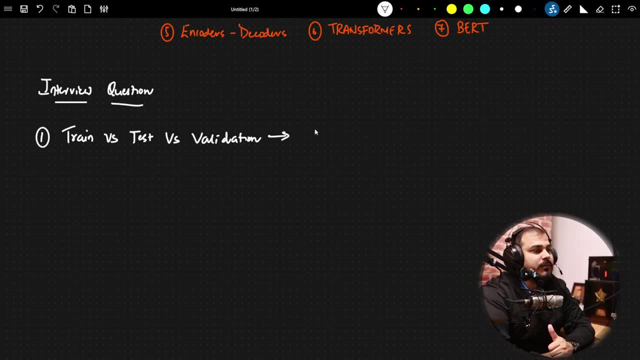 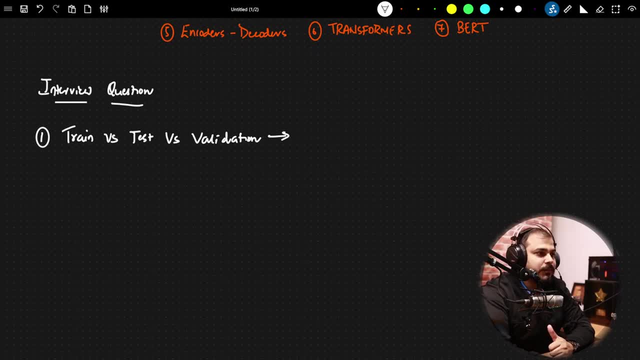 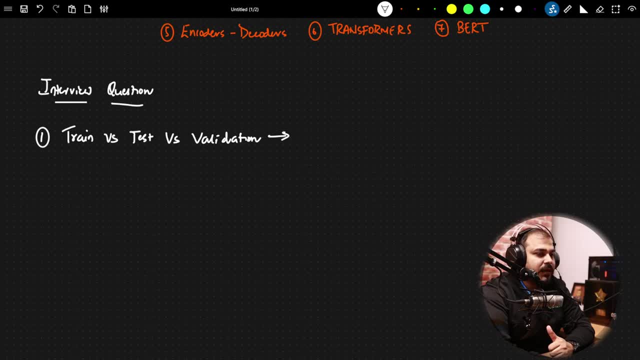 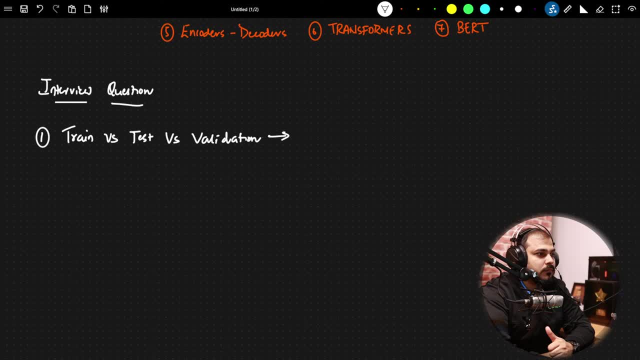 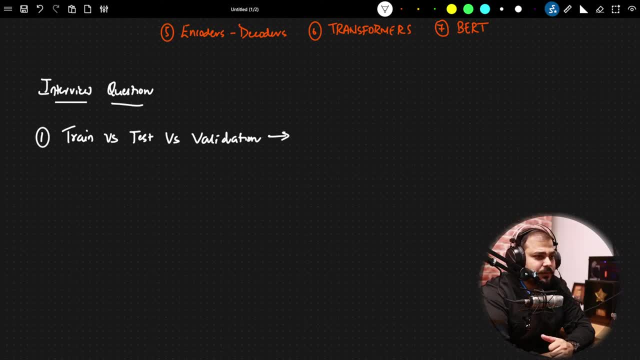 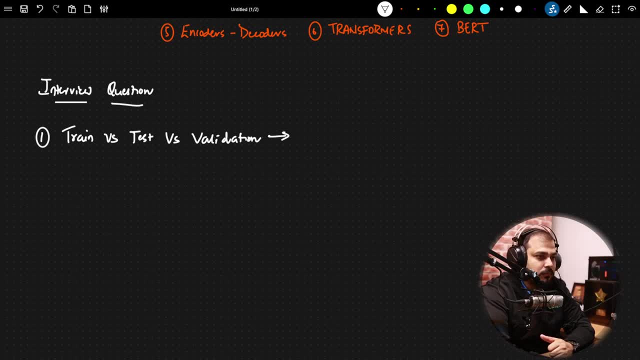 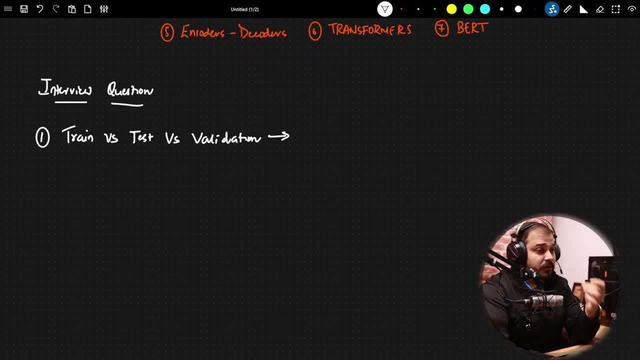 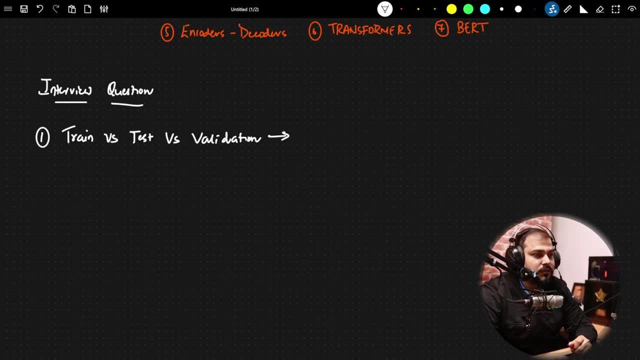 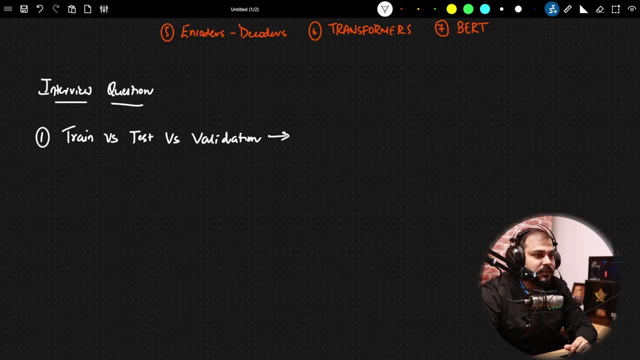 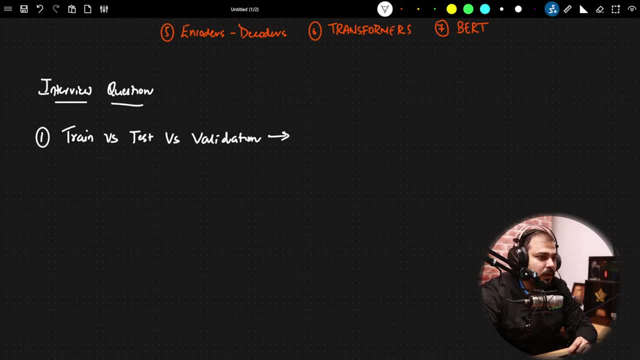 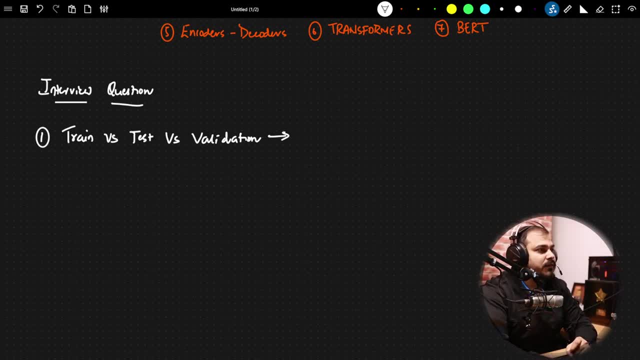 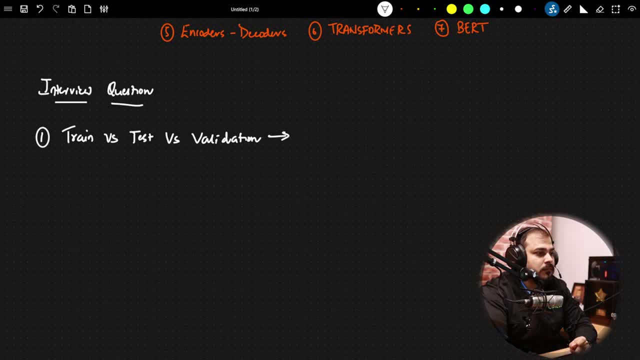 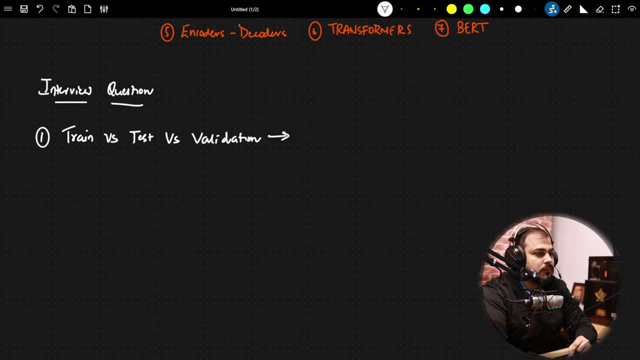 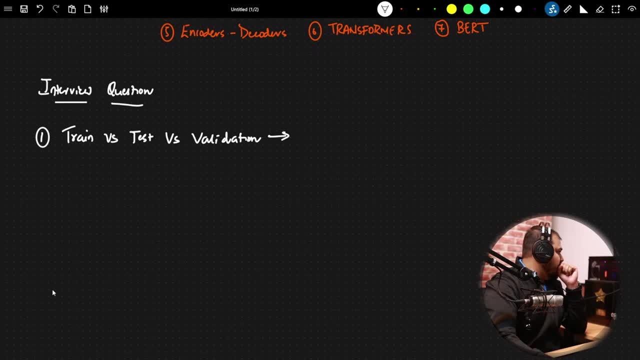 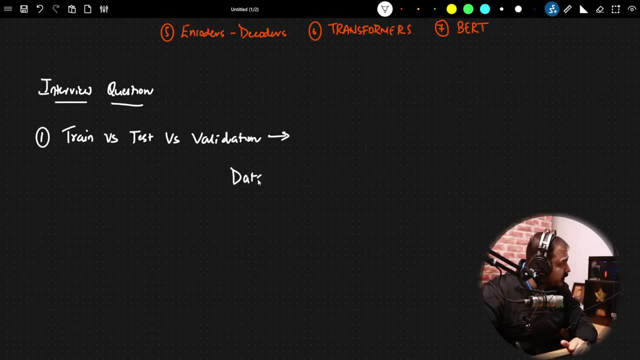 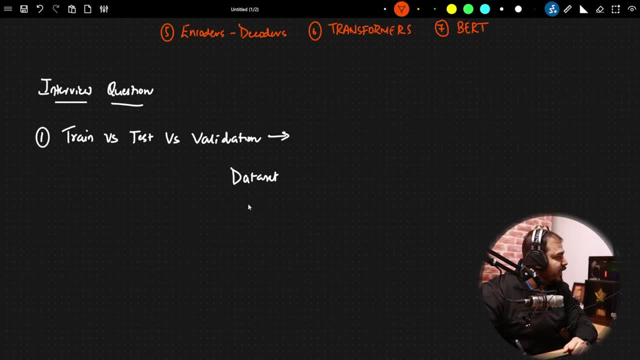 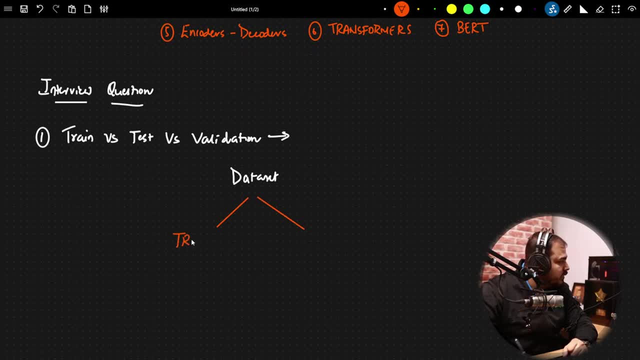 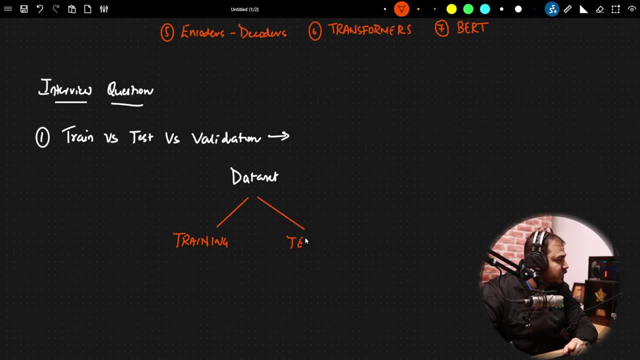 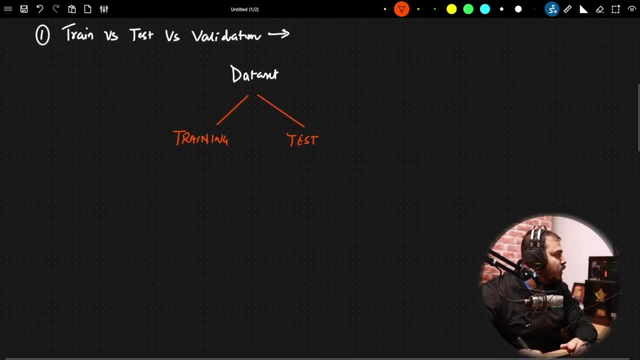 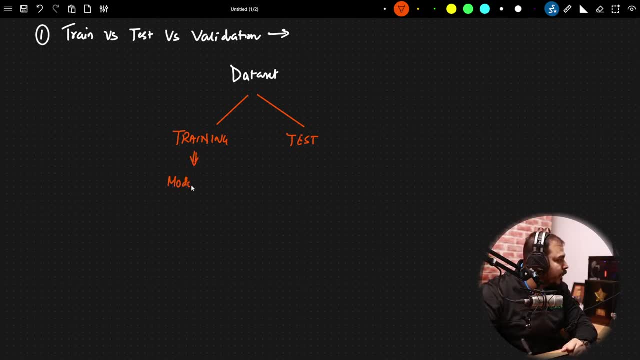 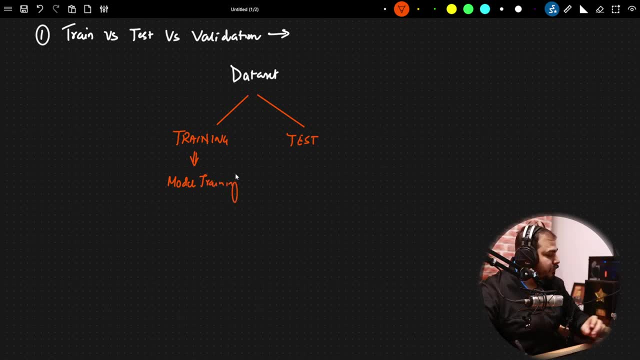 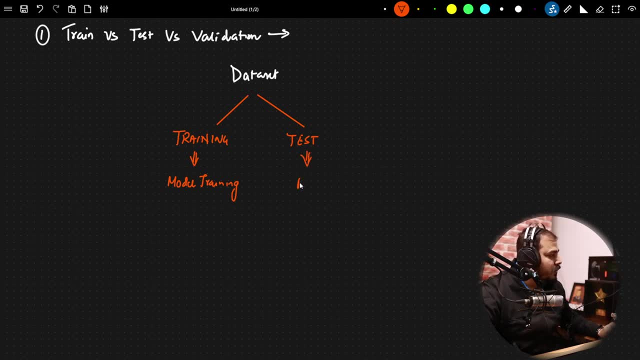 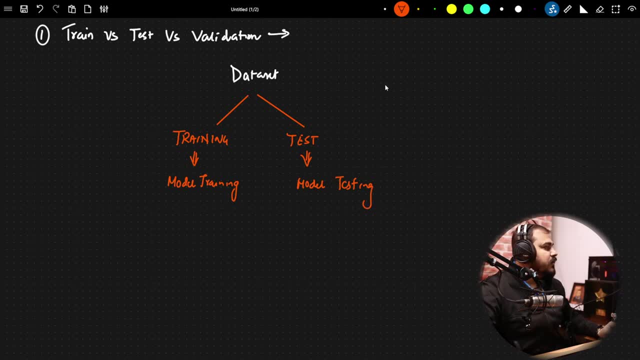 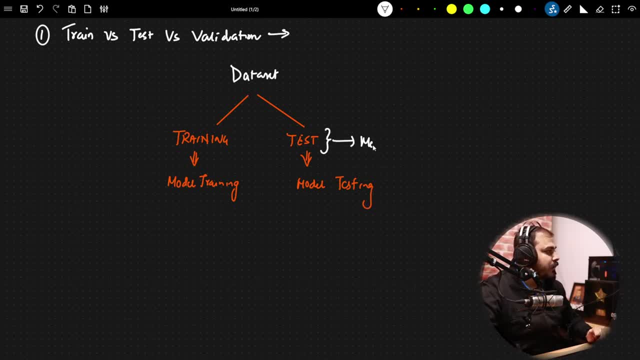 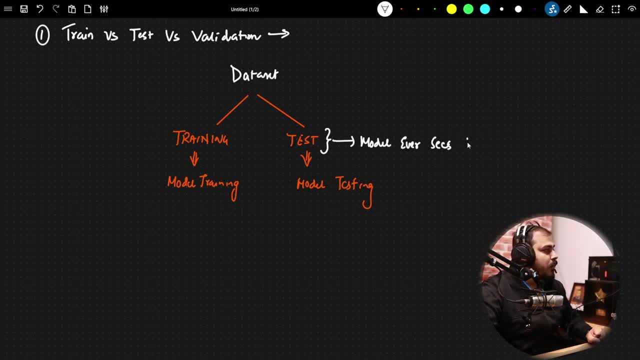 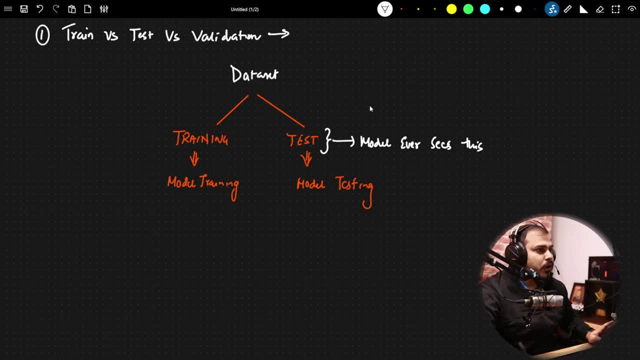 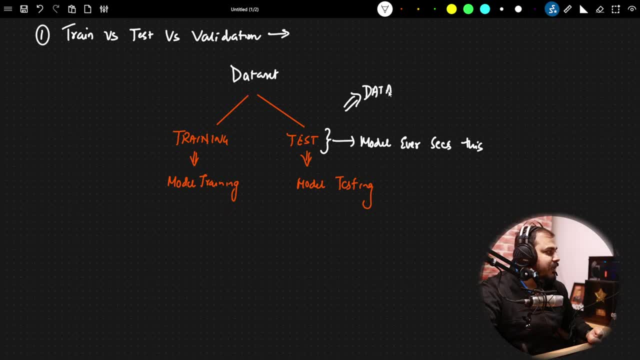 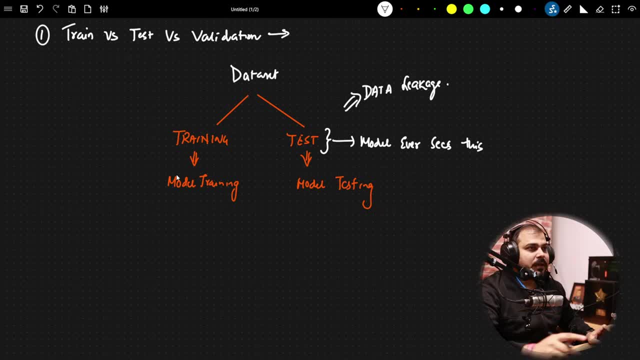 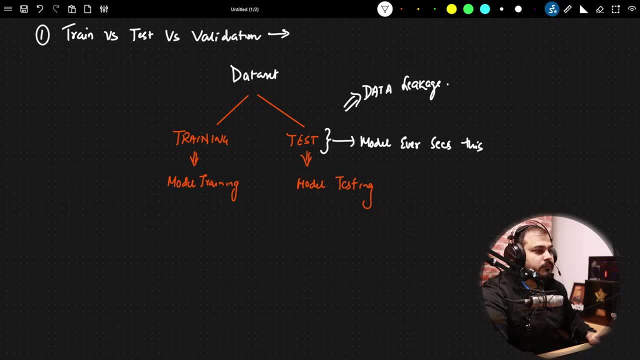 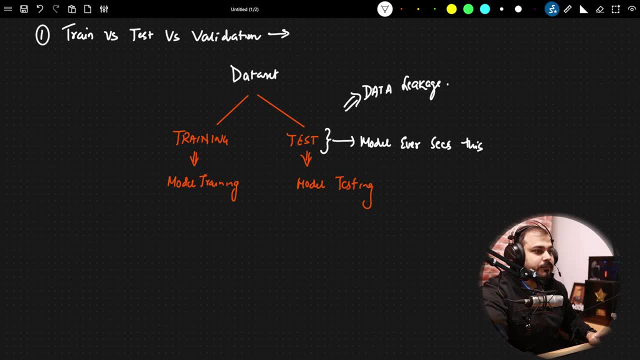 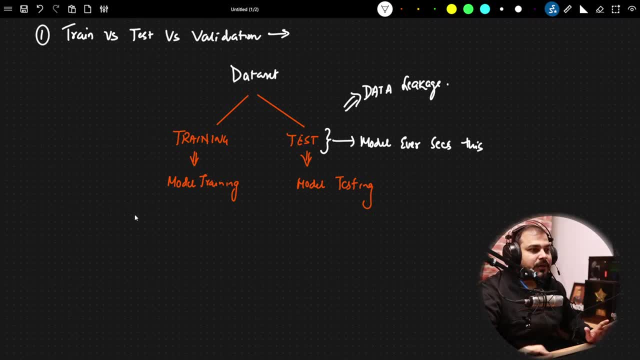 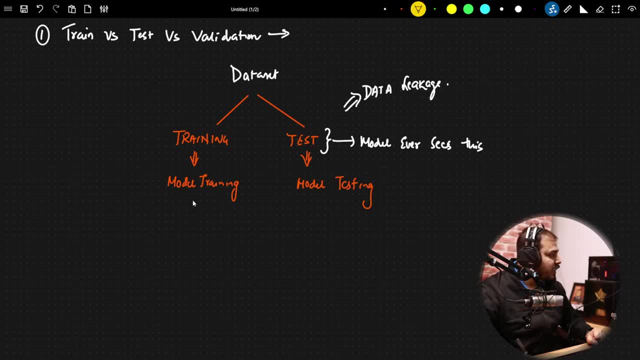 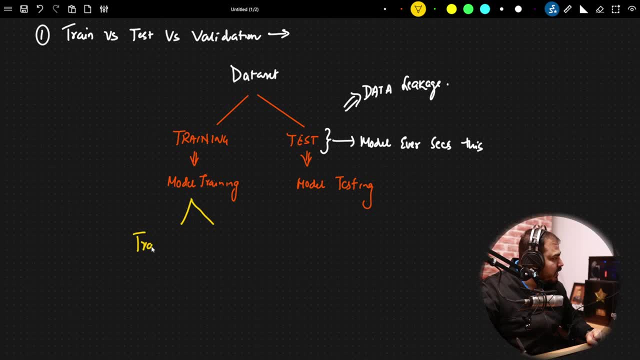 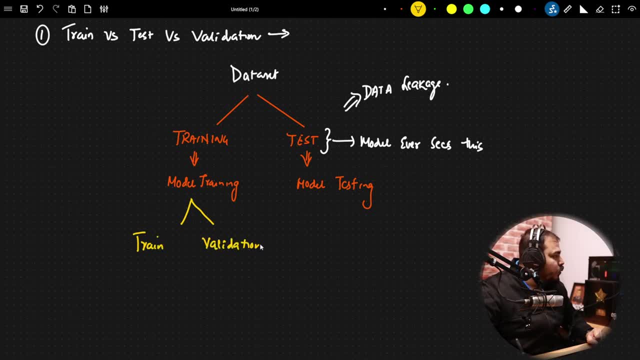 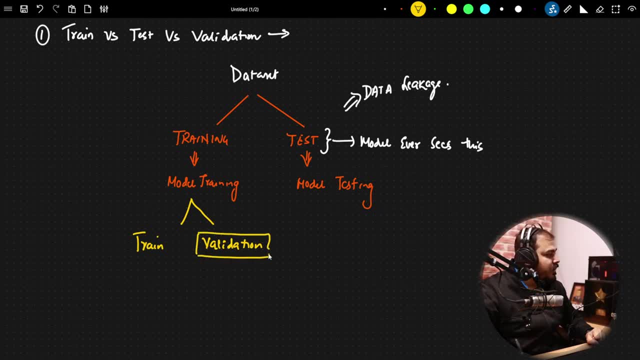 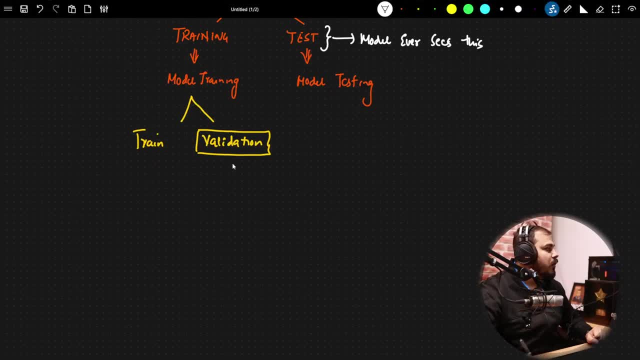 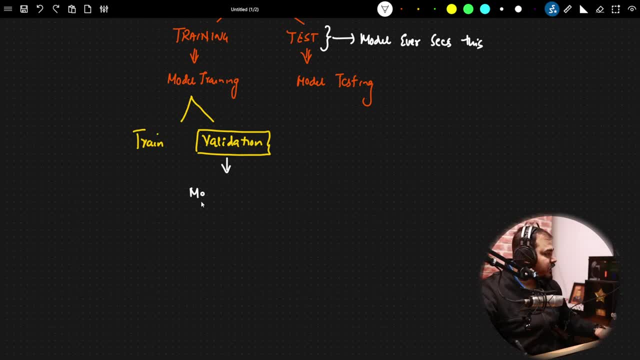 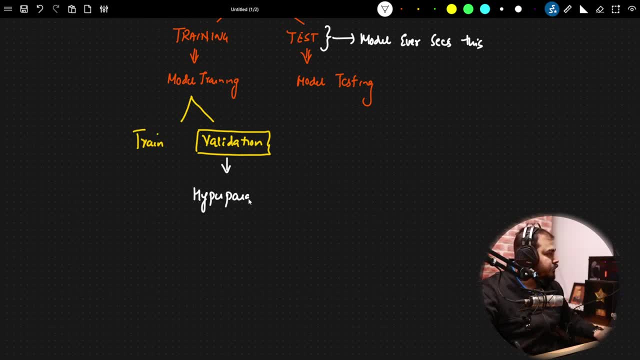 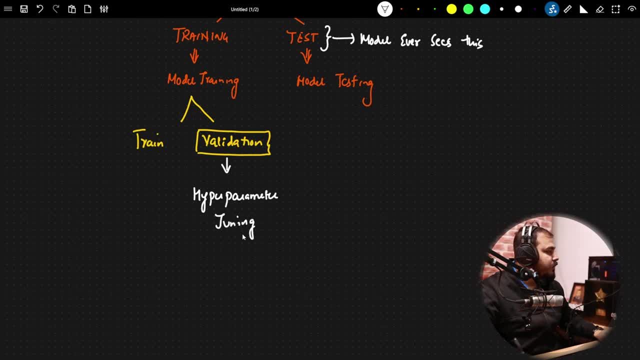 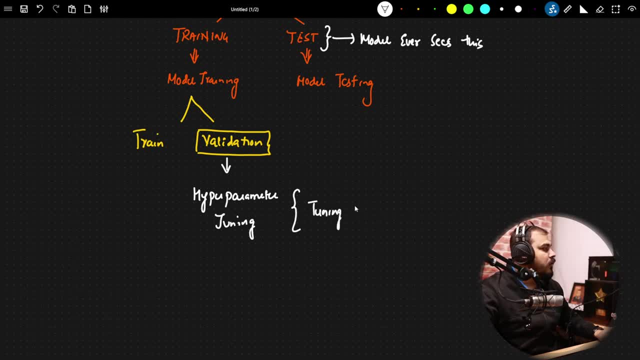 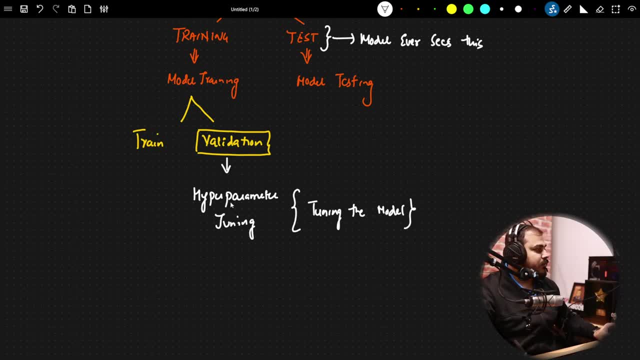 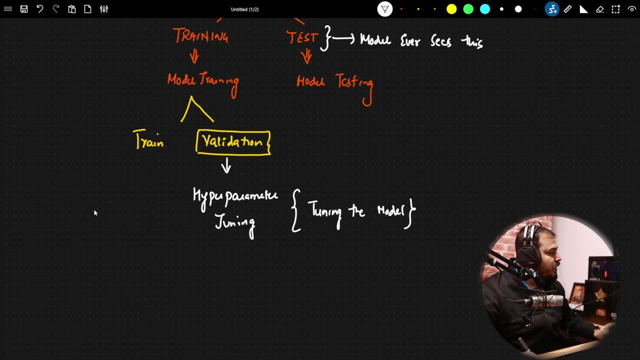 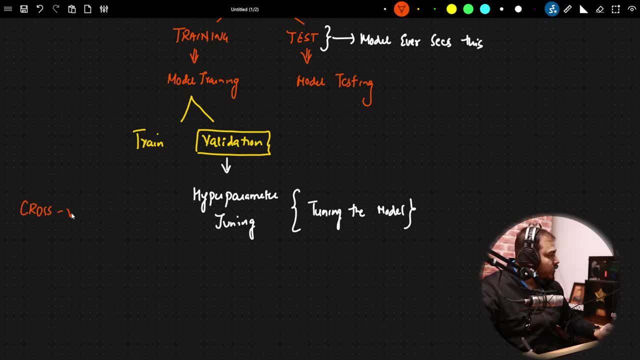 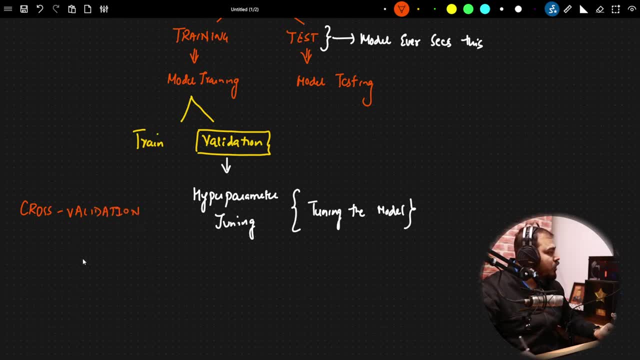 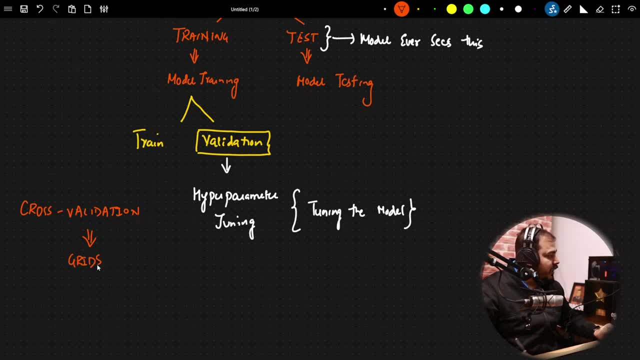 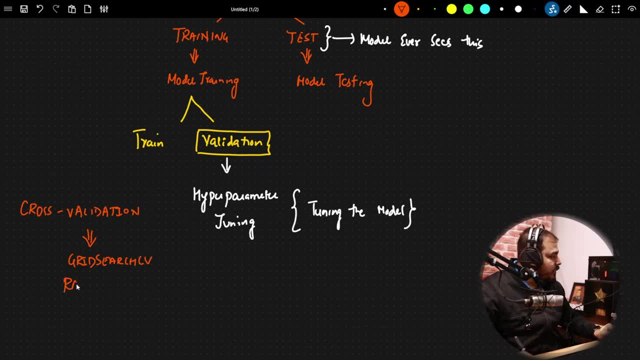 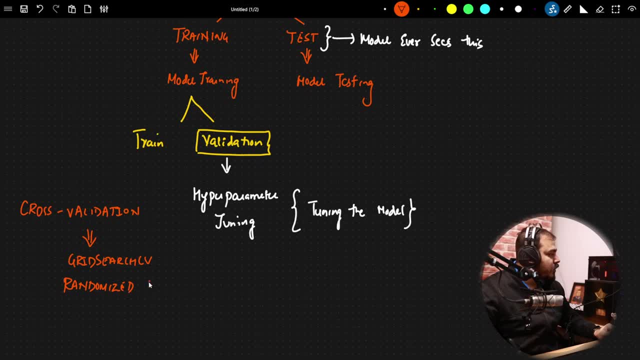 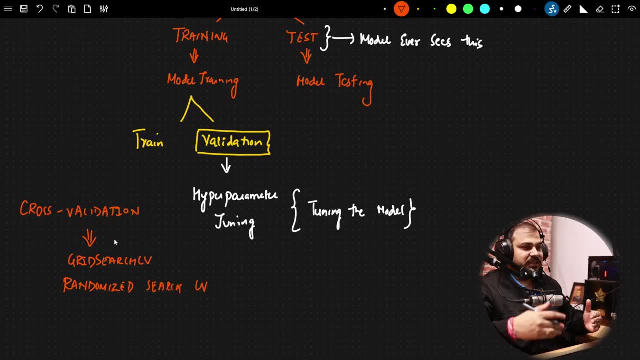 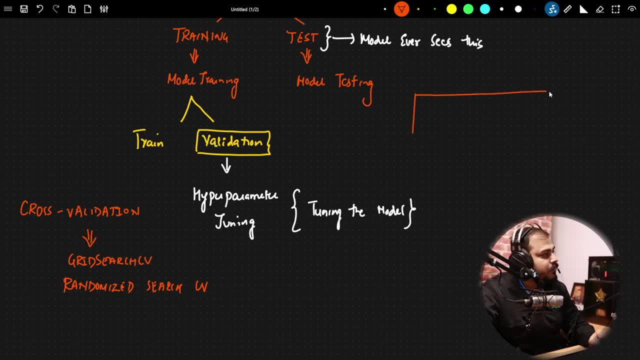 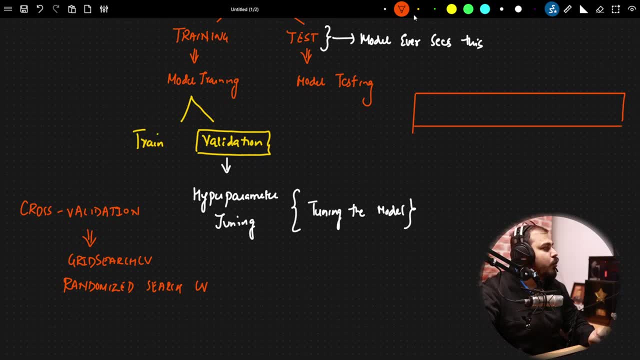 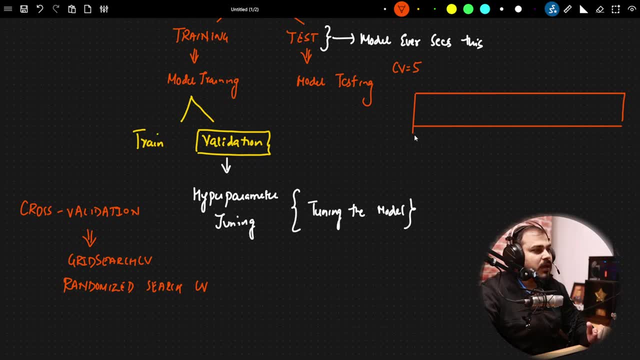 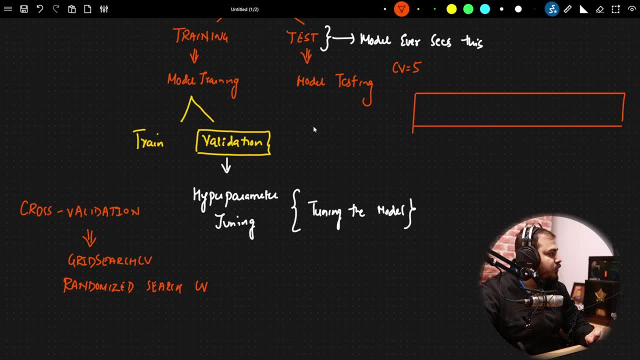 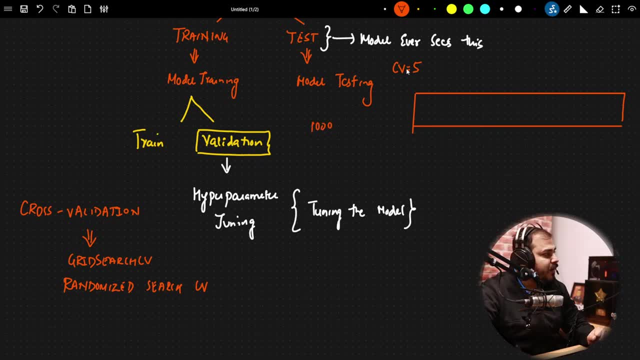 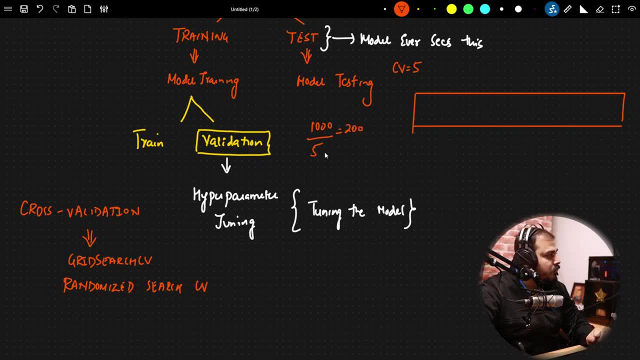 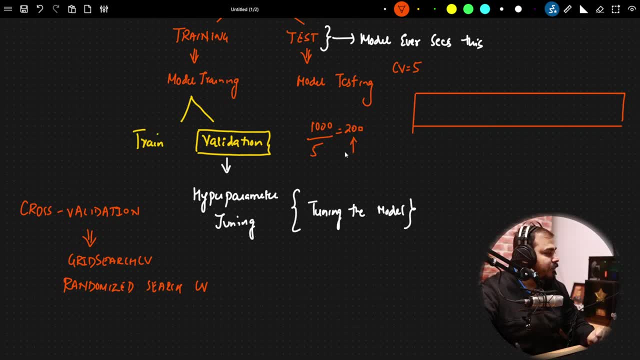 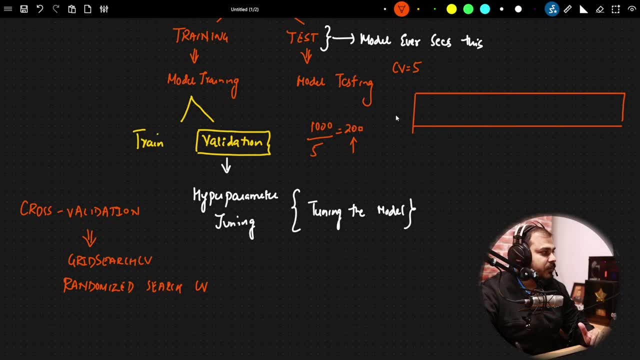 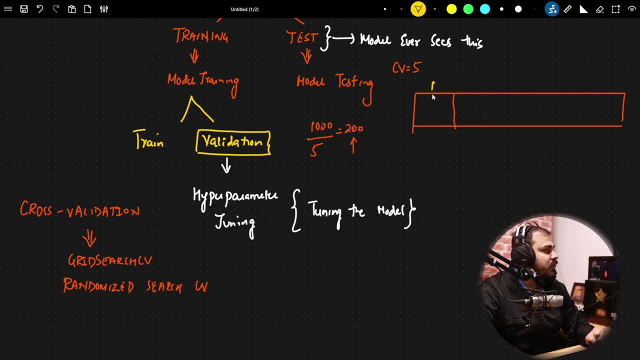 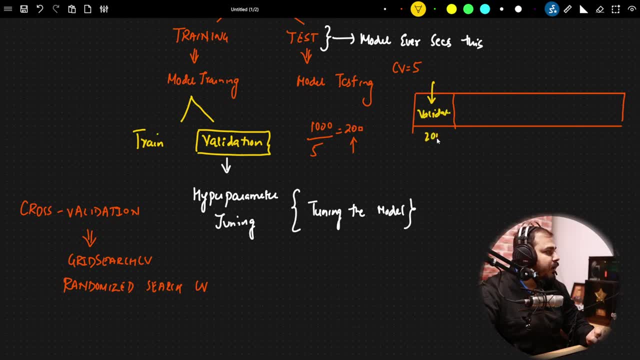 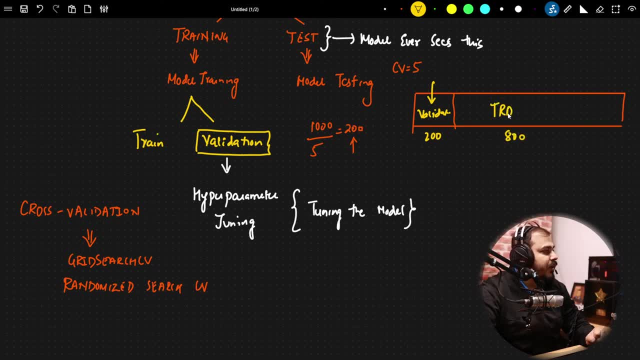 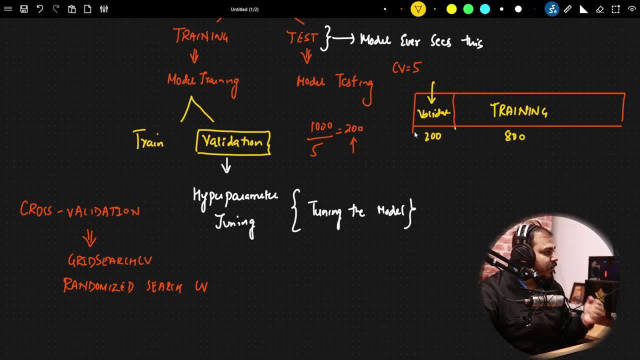 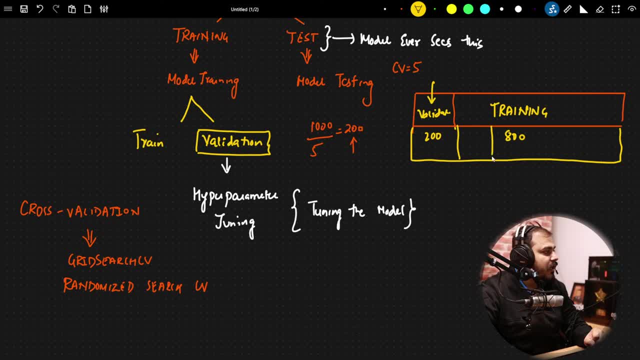 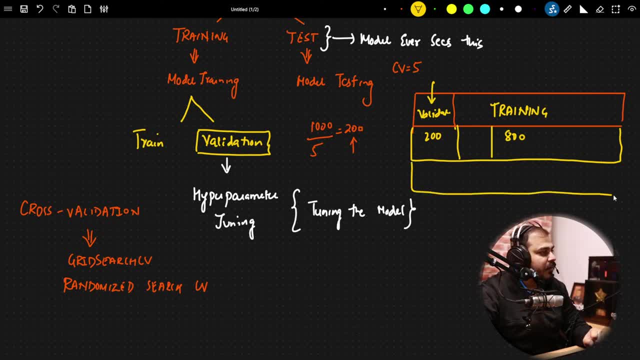 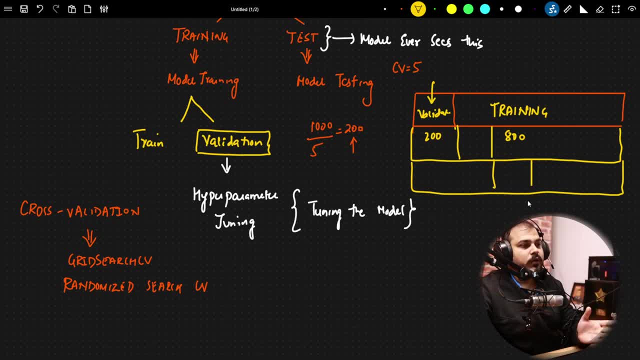 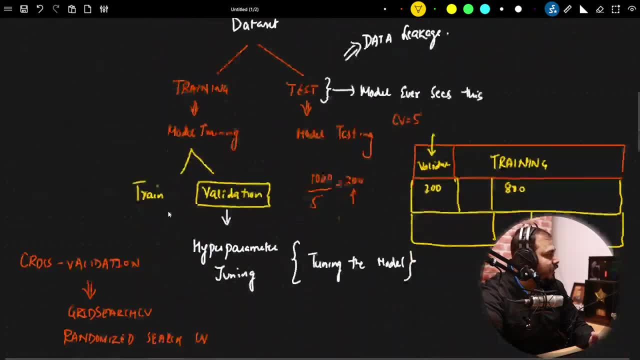 So today we are going to learn about the bottom to top. So today we are going to learn about the bottom to top. So this is one of the recent interview that was basically asked. Now coming to the second interview question. Second interview question was simple. 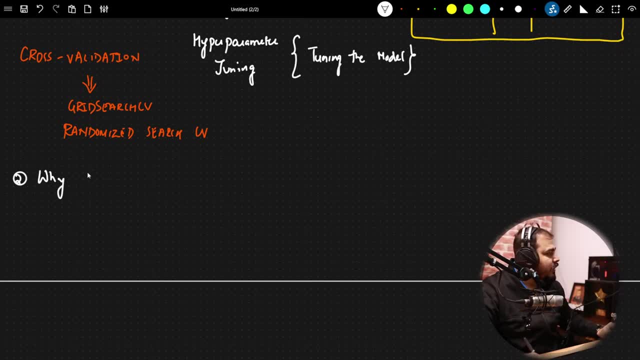 Why people use random forest mostly instead of decision tree. Okay, so this is the question. okay, Because you know that in random forest you have multiple decision trees. But why do we specifically do this? okay, Why do we use random forest instead of decision tree, or XGBoost instead of decision tree? 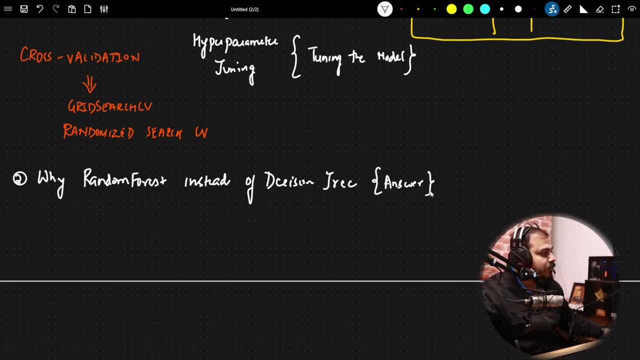 So this you can basically answer. I will just check out the comments. But yes, this is something related to bias and variance. okay, To provide overfitting, you know? So, when we say overfitting, what is the type of bias and variance we have with respect to overfitting? 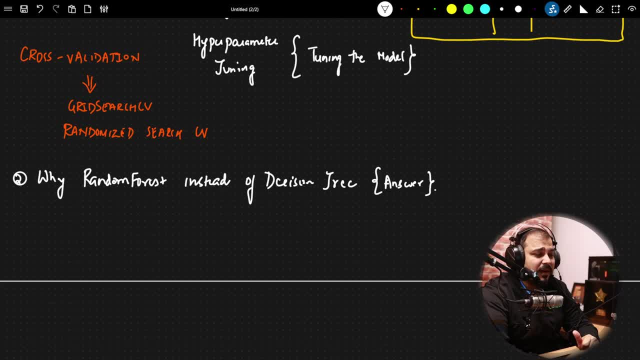 That basically, training accuracy is very good, test accuracy is very bad, right. So what is bias and variance? in that specific case, Can I say low bias and high variance. So decision tree usually has low bias and high variance, right? So in order to reduce this high variance to low variance and specifically to keep this low bias as low bias, 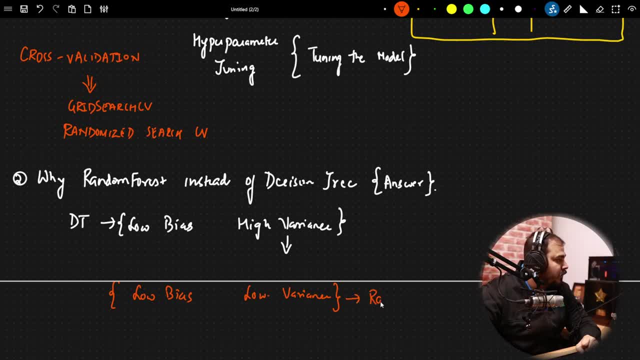 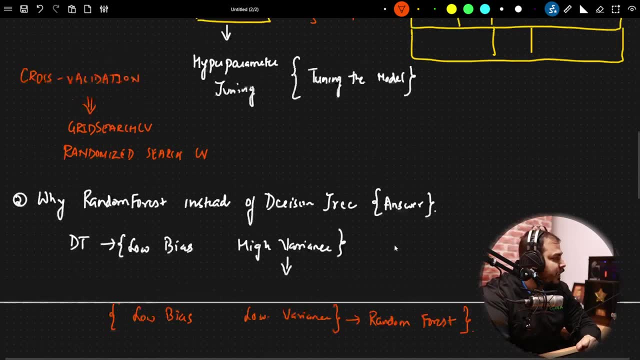 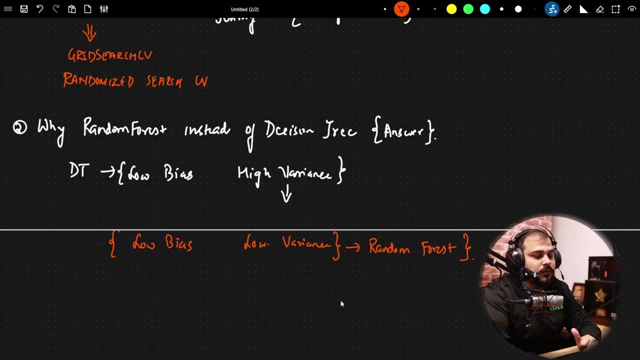 we specifically use random forest right, So this is what we specifically use right, So this can also be. this was also one of the interview questions that was asked to one of our subscriber, a person who was studying in iNeuron, and he answered it well, right. 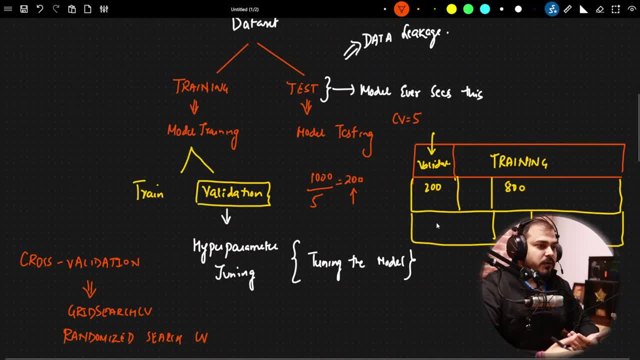 So good, Should I follow this strategy, prepare some interview questions? Yeah, from tomorrow we'll also be having quiz. Today I did not get time to prepare the quiz questions, but I hope everybody has got this right. And yes, random forest is a bagging. 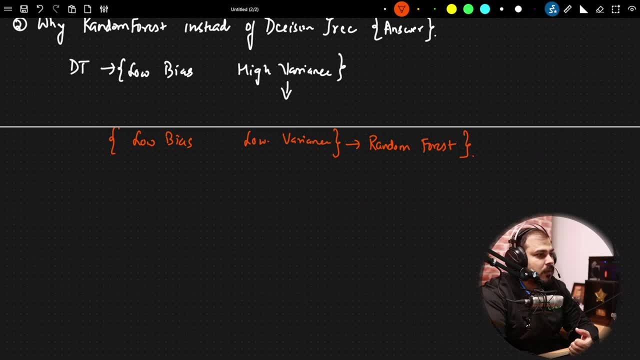 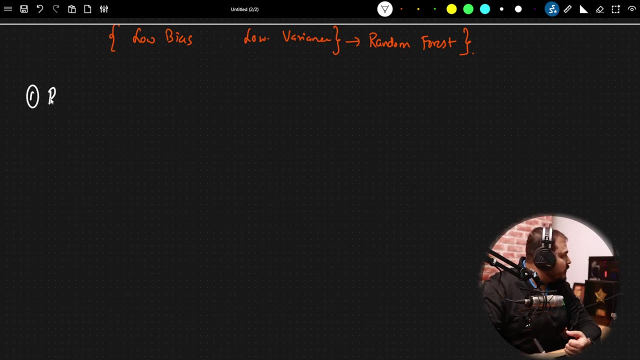 Right, right, Perfect, Okay. So shall I start the today's session now? Yeah, Okay, first, Now let's go ahead and discuss about something called a recurrent neural network. We'll go slow by slow, So we'll try to understand what exactly is a recurrent neural network. 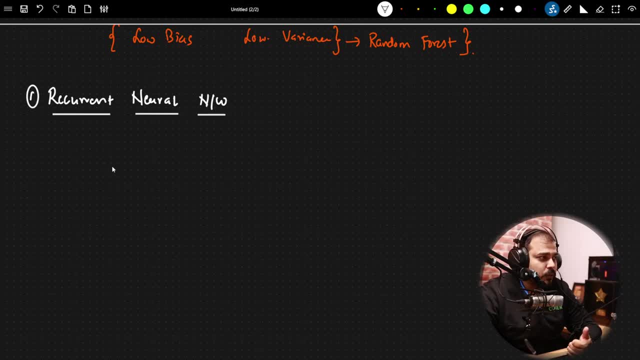 And you know what all things we can actually do, you know. so all those things will be there in this Now, in recurrent neural network. there are some important things, right? Okay, let's go ahead and discuss about the recurrent neural network. 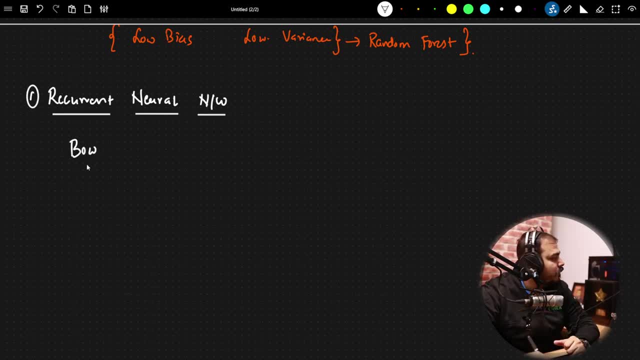 Now till now, the things that we have seen to convert text to vectors. okay, When we are using text to vectors, Or when we are converting This text to vectors, right, What is the most efficient strategy we have found out till now? 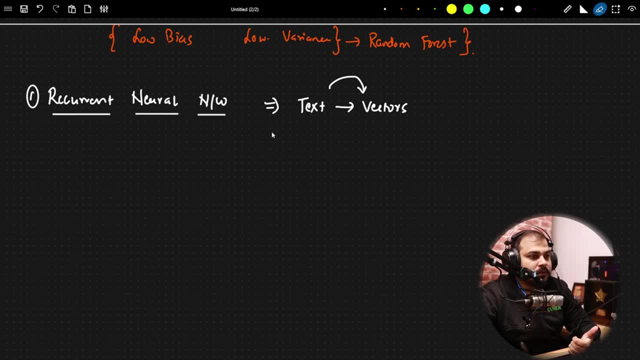 Tell me What is the most efficient way that we can basically find out, Or how we can actually do By converting text into vectors. If I really want to go with text to vectors, which is the most efficient way that we found out till now. 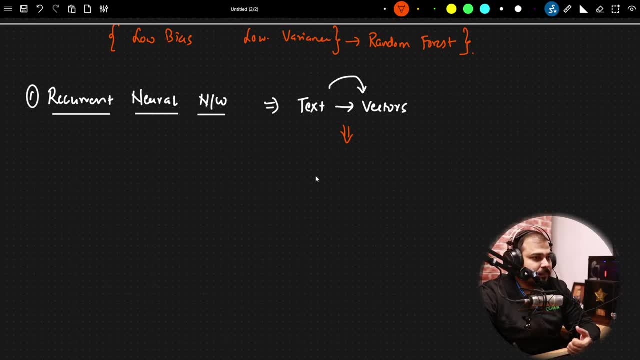 From all our previous session. Yes, obviously many people are saying it. right, It is word to word. And then what we do? We basically use average word to vec And this is nothing. but this is a embedding layer, right, Embedding layer. 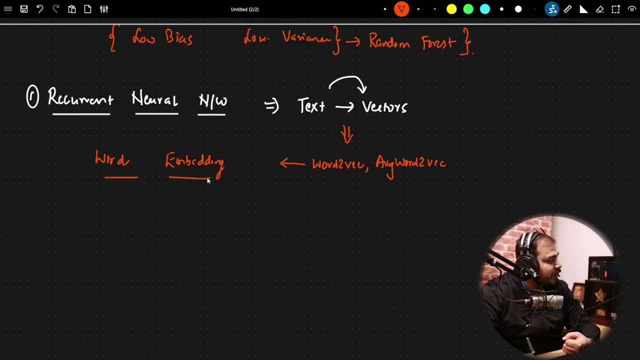 This is something called as word embedding, Okay, So this we have actually found out. Okay, But let's talk about some amazing applications. Suppose I have a specific chat bot. Now, in case of a chat bot, just consider an application with respect to chat. 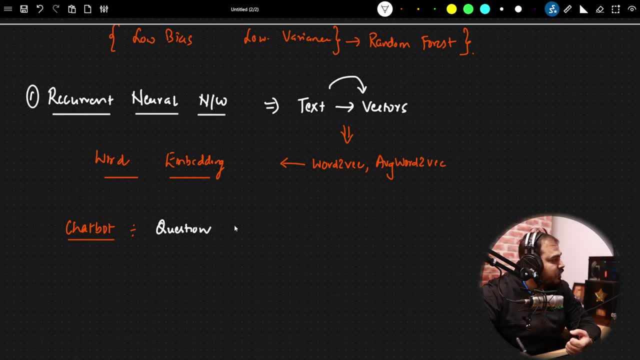 In chat bot you ask a question And specifically, you get an answer. Right, It is just like a Q&A- Specific question. whenever you are asking, you get a specific answer. Okay, So in this chat bot, each and everything are very important. 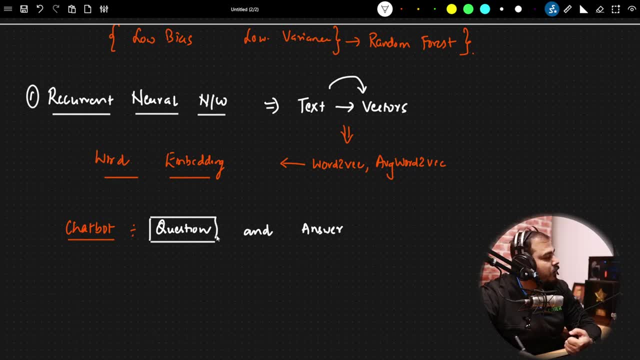 The question right. Suppose if I am asking a chat bot- hey, how are you? What is the weather outside? You know The chat bot should understand the proper context of all the question and probably answer it Right. This is a very important application. 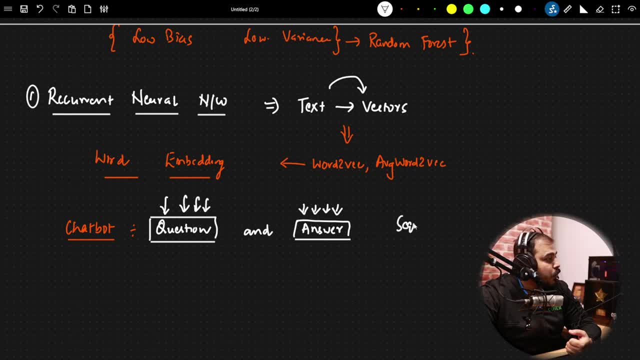 Let's say Over here what is the most important thing: The sequence of words. right, Are very important. You have to make sure that the sequence of word is very, very important, Right? Okay, Let's go to the next application. 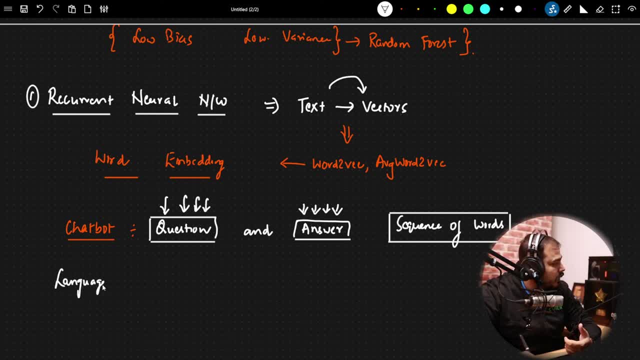 Have you seen language translation? I hope everybody knows Google Translate, Right? So in Google Translate you have a specific word from one language, Let's say from Hindi. You want to convert into English, Right? So here also, sequence of the word is super important. 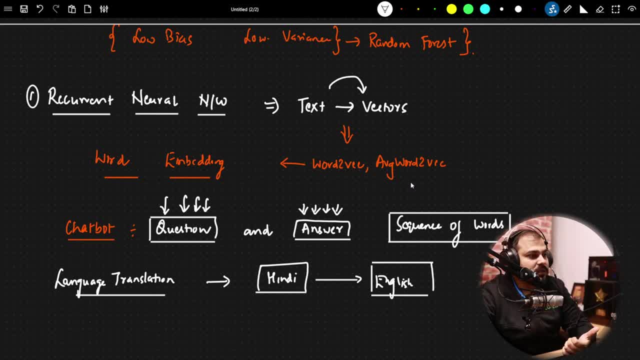 And you have to make sure that grammatically, all this, all this you know, conversion should happen properly so that it can be used efficiently throughout the world, Right? So language translation is also a very important thing And probably if you go and see in Google Translation there how accurately you probably get all. 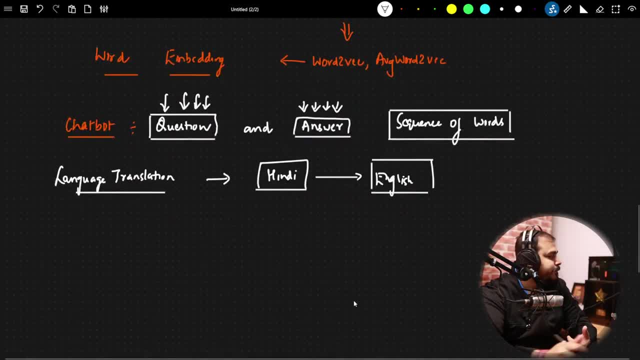 the language translated. Okay, Now if I take one more example: okay, over here, let's say: language translation is there, Chatbot is there. You also have sentiment analysis. Let's say you have something called a text generation. Now, right now, if you open your Gmail and probably start writing a sentence, right, 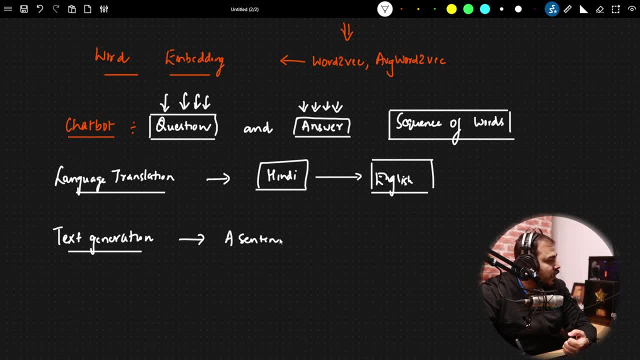 Does it give you suggestion of the upcoming sentence Suggestion? It gives you a suggestion of the upcoming sentence Suggestion. It gives you the suggestion for the entire sentence, grammatically Right. So this suggestion to completion of the sentence. Completion of sentence. 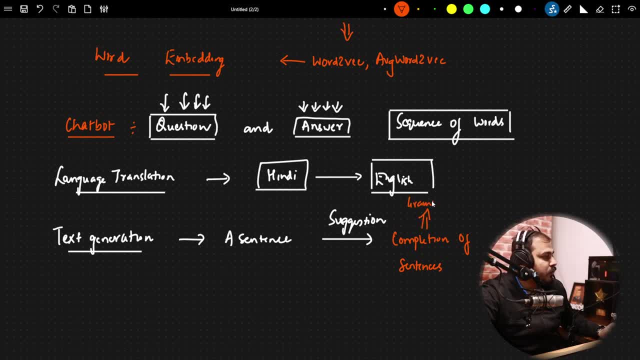 So grammatically it gives you very well, Right? So grammatically it makes sure that it provides you all the suggestion, Right? So I think you have also seen this. Probably, if you open Gmail and you start writing something, automatically all the suggestion. 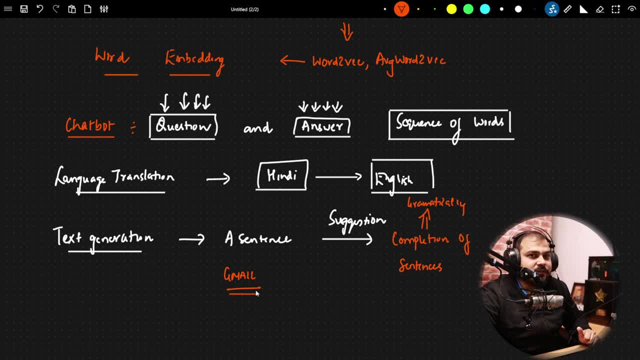 will come Similarly in LinkedIn. it also gives you auto suggestion. Okay, There is something called as auto suggestion. Okay, If you have an email ID, suppose let's say the email says that. or suppose if you have seen chatting in LinkedIn, right, 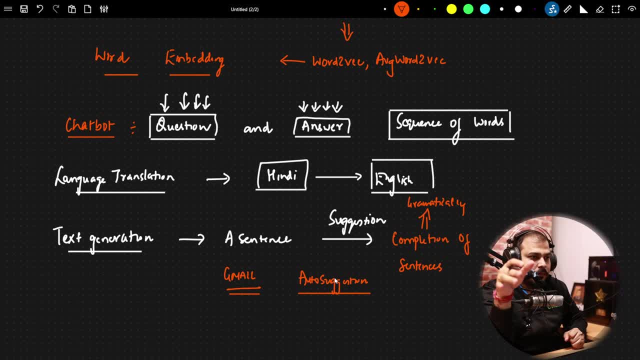 Whether you probably write, hey, are you free, You know? So suddenly you get a suggestion: Okay, Create a video meeting, Okay, Something like that. Automatically, multiple suggestions will be there, Right? So all these kind of models. the most important thing is sequences of words. 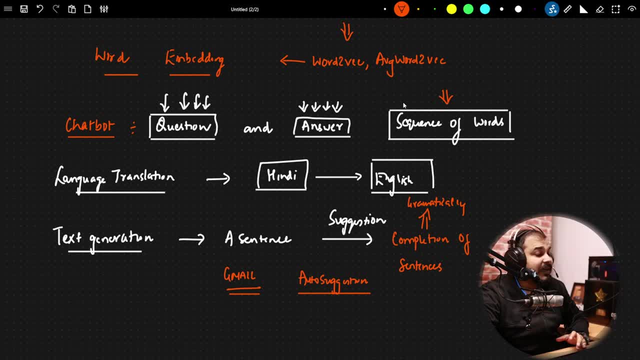 Grammatically. it needs to be right. You know Entity models. you also have entity label models, Right? These are all simple, very important Here. all these applications are super important in terms of creating a real world application which does most of the tasks that actually people require. 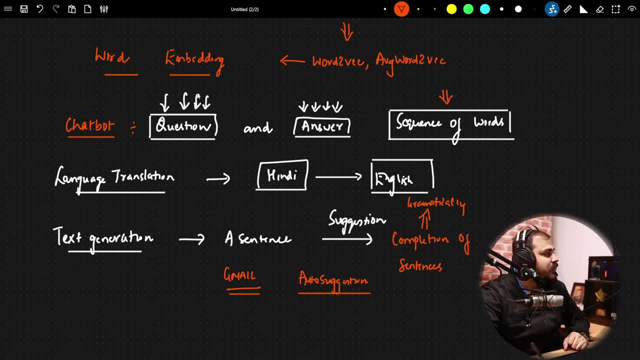 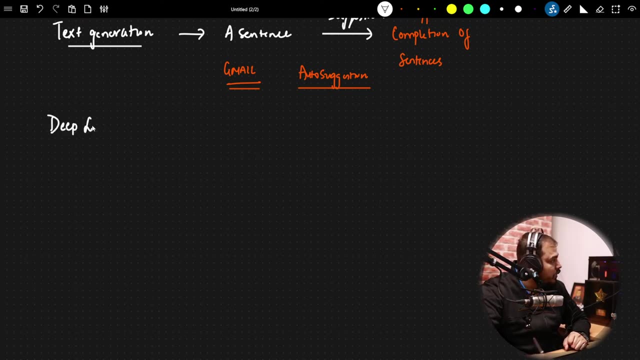 Very important task, Okay, So for doing all these things, we cannot be dependent on machine learning. We cannot be dependent on machine learning, So we have to be dependent on deep learning techniques. So deep learning techniques like what? So deep learning techniques? deep learning techniques like what? 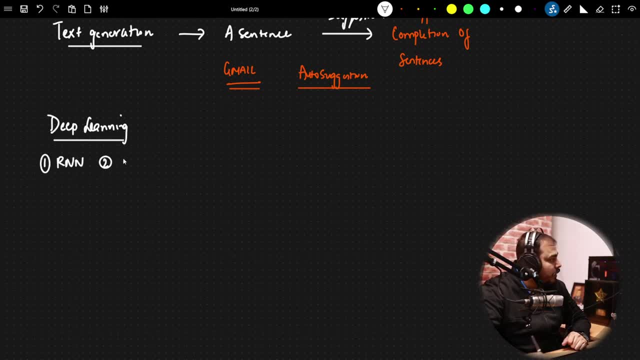 Like: I can take RNN. I can take LSTM RNN, you know, Because we will be training our vectors in this by using this neural networks. Right, Because machine learning will not be able to give us very good accuracy. Let's say LSTM RNN. you have transformers, you have BERT, right? 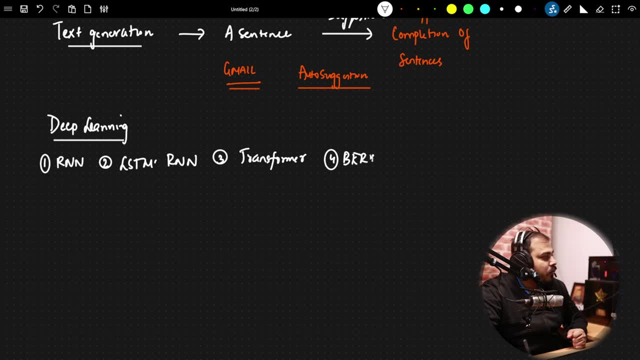 Efficient models And you know, at one point of time. you know Google search engine- let it be- or Gmail have used this kind of models And probably right now it may be using transformers or it may be using BERT. 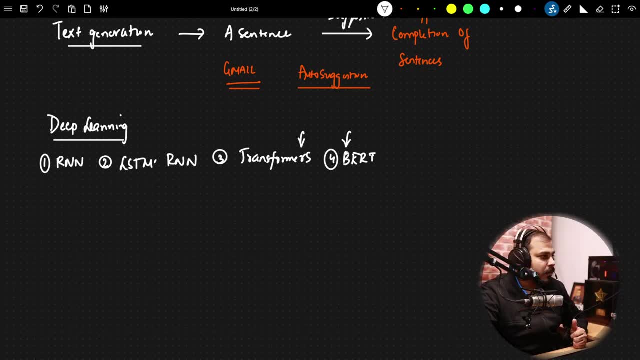 You know, Because this is the most beautiful part. You know So what we are going to do. We are going to learn slowly each and every architecture. We are going to learn it with practical application, And we are going to do it. 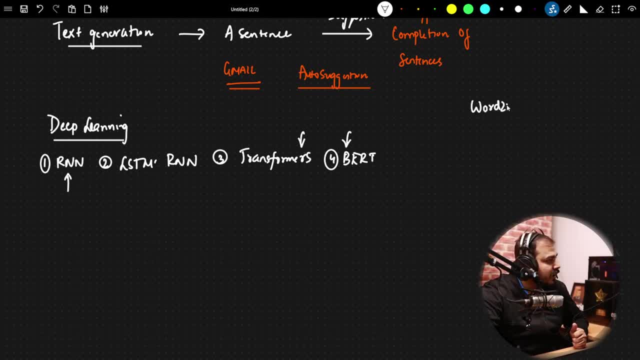 Okay, Now people may be thinking: Krish, what is Word2Vec then? Word2Vec is a technique in deep learning which we can train a model, Which we can train a model, Or we can use a pre-trained model which actually converts word into vectors. 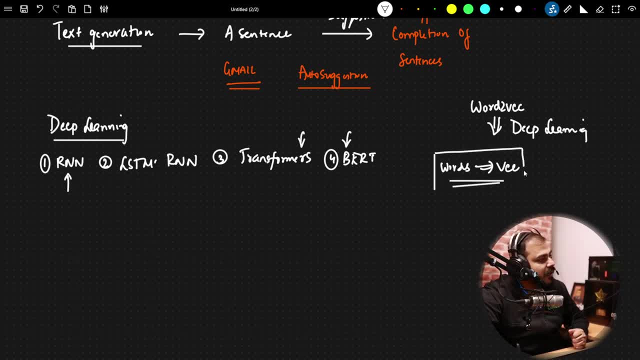 Okay, And why this is much more efficient? Because semantic meaning is actually captured Right: The vectors. that is basically created. semantic meaning is actually captured Right. So I hope till here you have some amazing knowledge. I hope you have understood till here. 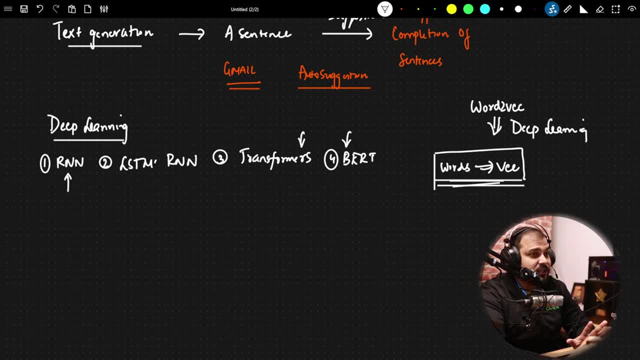 Yeah, Everyone. And again, whatever I am teaching you, this will be super important, even in interviews. So can I get a quick yes, if you are able to understand. And if you are able to understand, you know, please do hit like. 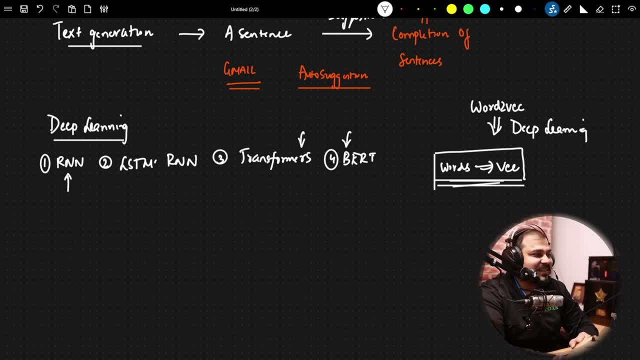 That would be amazing for me. Put some symbols in the chat That will actually give me some amount of motivation. Right Hugging face is also kind of library which you can internally. you can use transformers to train a specific model and many more things. 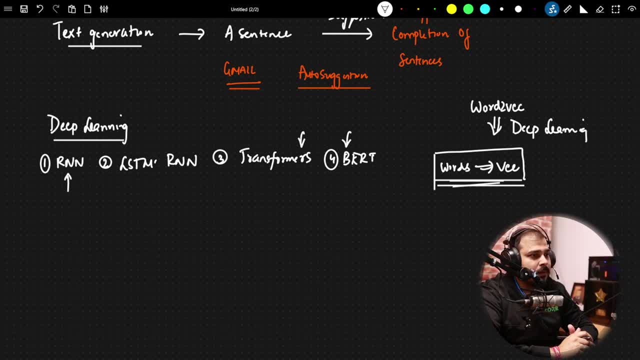 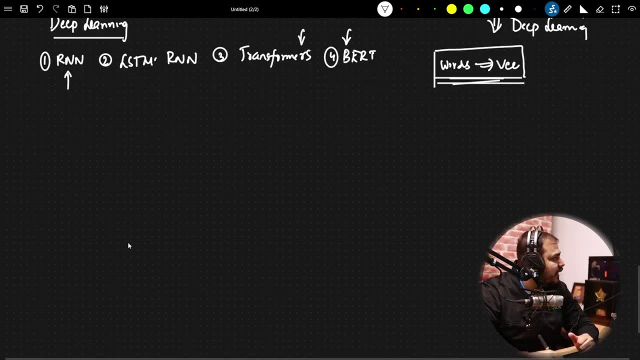 Okay. Okay, Now let's go ahead. At least make 100 likes, so that we continue Now. first thing That we are actually going to discuss about is something called as recurrent neural network. Now why recurrent neural network is amazing, Okay. 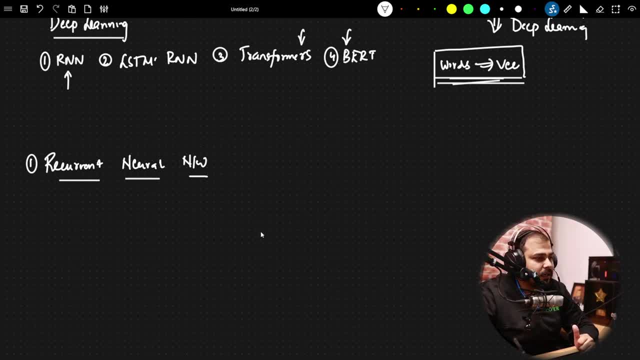 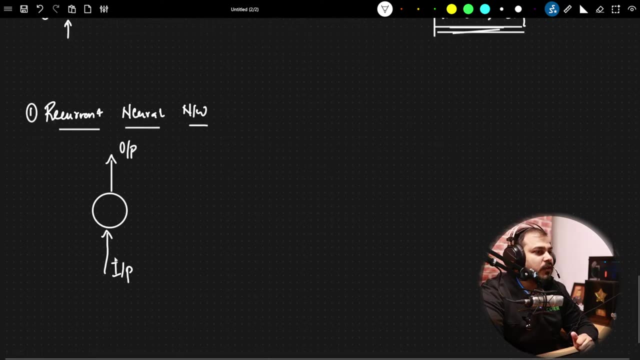 A basic diagrams of the recurrent neural network that we can probably see. Let's say: this is my neuron, Okay, This is specifically output. This is specifically input, I have my input, I have my output, Okay. And this neuron may be a single neuron or it can be multiple neurons. 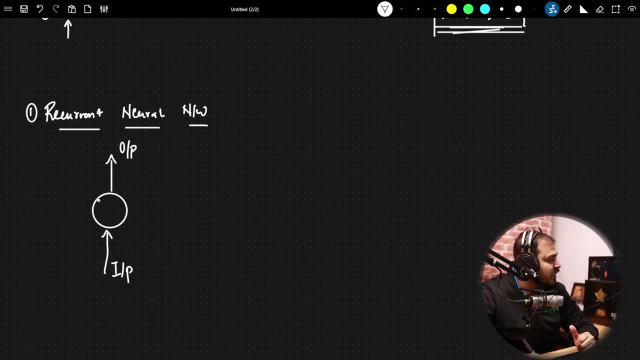 It can be even 100 neurons, Okay. So just consider this one layer, Okay, And whenever we get one kind of output, this output is also sent back to the neural network. Okay, This is the basic architecture of neural network. recurrent neural network. 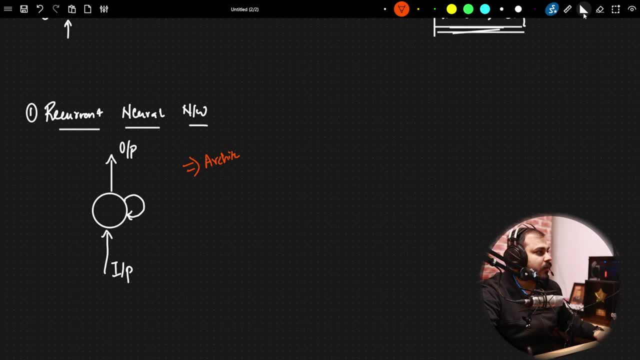 A basic architecture of recurrent neural network. Okay, So we will try to see to it. Okay, Now, if I really want to expand this, I can give this notation also, and I can give this notation also. See This notation also. I can basically give. 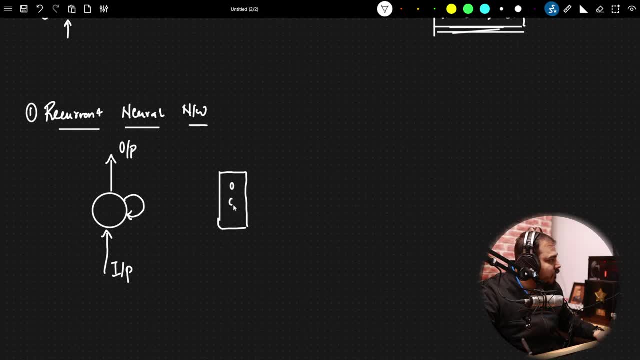 Suppose there is a layer. Okay, I have lot of neurons, Let's say 100 neurons or any number of neurons. This takes one specific input, This gives one specific output, And this output can again be sent back to the neural network. 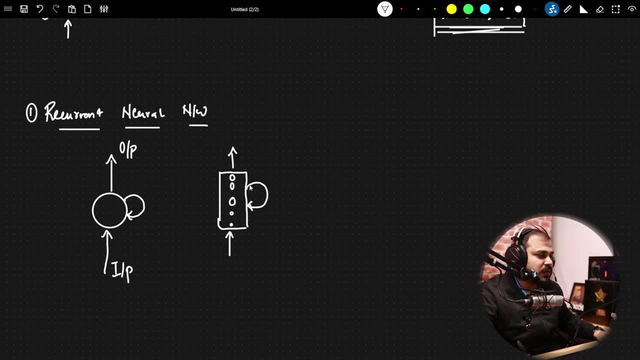 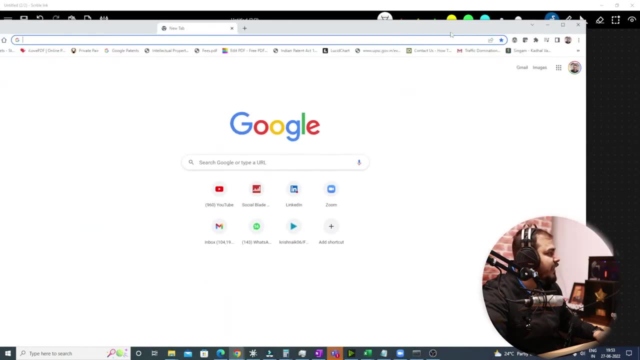 Okay. So this is another architecture that you can specifically use And there are multiple ways. Like, suppose, if I just show you, And probably if we also use some NLP applications like this, Like I will just say you, Okay, RNN. 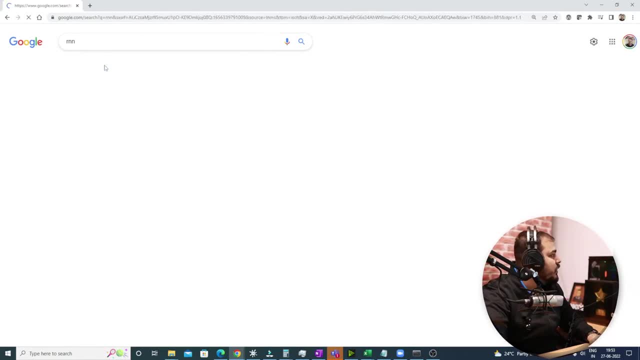 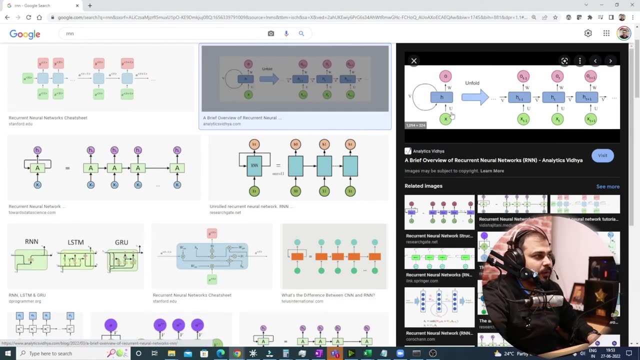 Okay, Let's say I am just going to search for RNN over here And let's go to the images. Okay, See, Everybody, can you see this? Let's take this specific example: We have an input, We get a specific output. 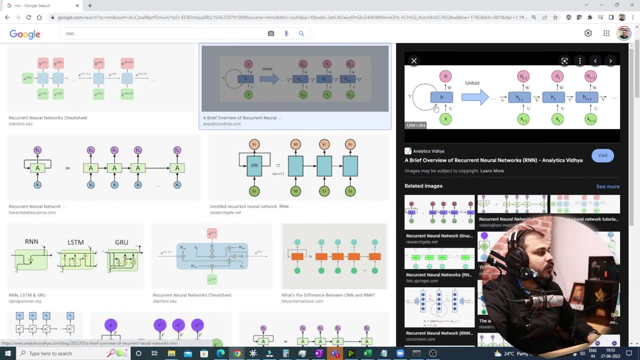 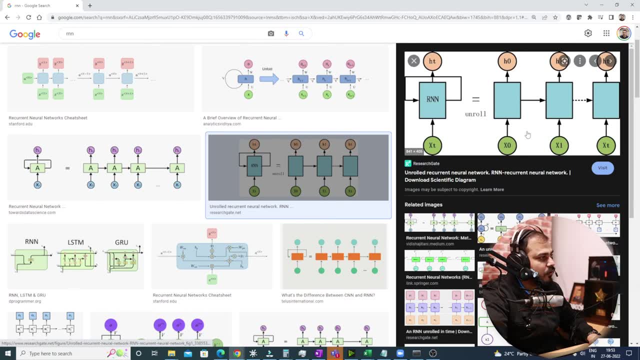 And with respect to this output, it is again given back to the neural network. Very simple, Everyone, clear. Can I get a quick yes? See Here also, Just focus on this. I will try to draw this later on. So I have a recurrent neural network. 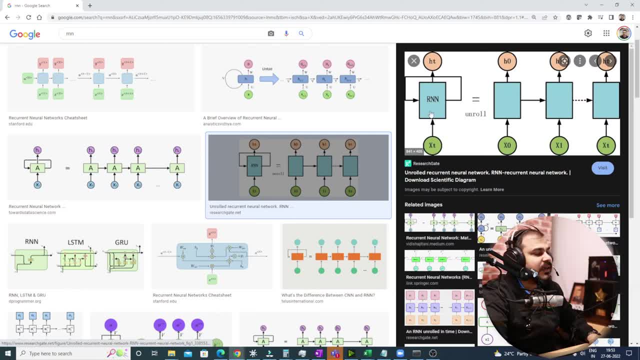 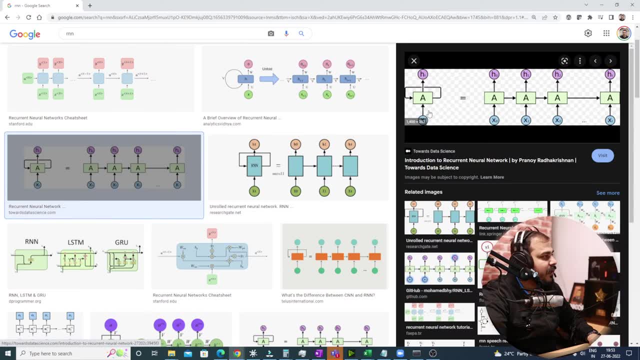 I give an input, I get an output, And this output is again sent back to the neural network. Okay, Everybody clear? Yes, Again. One more example: I have an input, I have an output, And again this output is also given back to the same network. 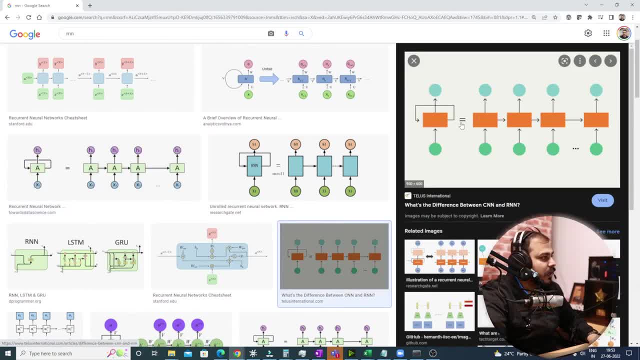 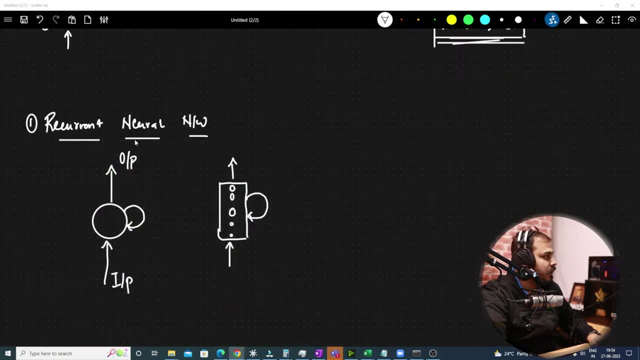 Okay, And anything that you probably see over here. Again I have an input, I have an output, And again it is given back to the same Everybody, clear, Yes, Perfect. So this is what it is. Okay, Now let's go ahead and let's try to expand this. 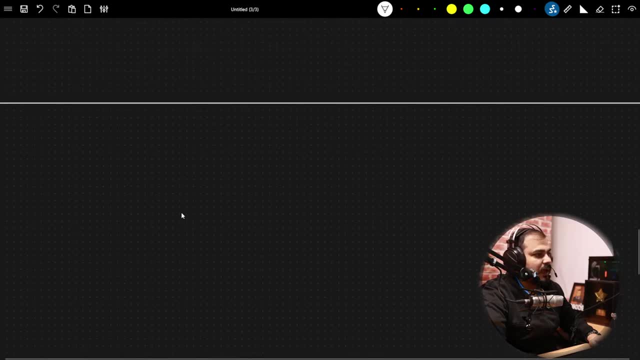 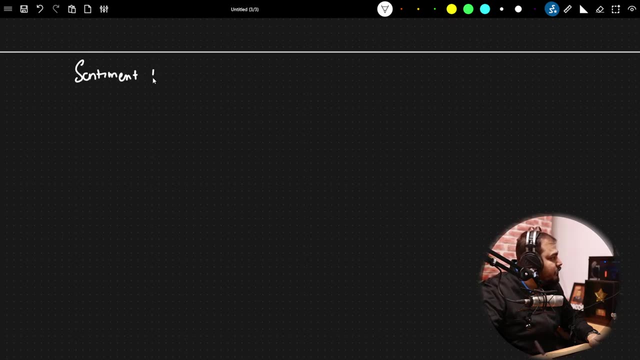 Okay, We will try to expand this network. Okay, And I will try to expand it by considering a very simple application which is called a sentiment analysis. Okay, Sentiment analysis. Okay, Or forget about this right now. Forget about this. 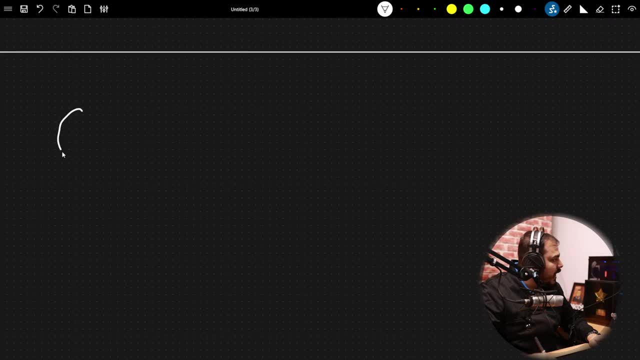 So we will try to see to it. Okay, So I have a network which takes one input, which gives one output, And then again this output is given back to it. Now, if I try to expand this, Okay, If I try to expand this, 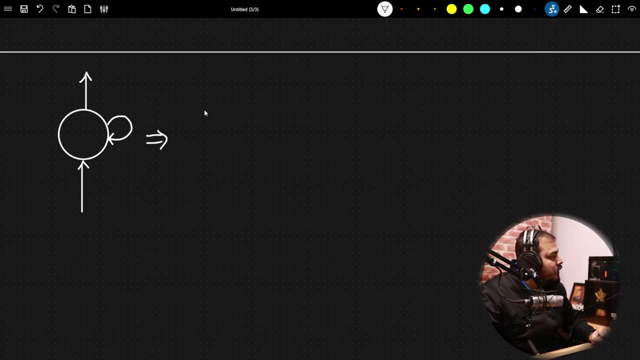 Okay, So let's expand this. Okay, So how this will get expanded. So I will be having a neuron like this: This will be my input. Sorry, This will be my output. This will be my input. Then what will happen? 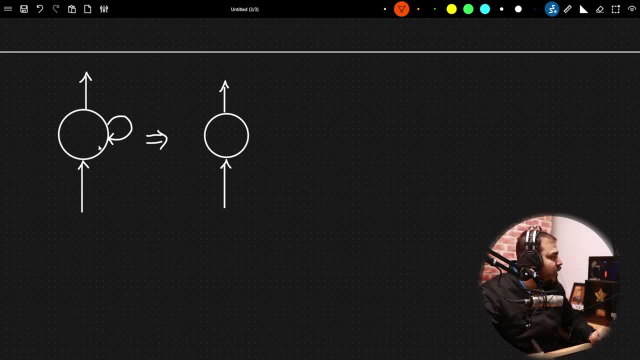 Since it is given back to its own network. So here will be one output. Let's give this back to the same neuron, like this, which will be having one input and one output again. Okay, Then again, this will be given back to the same and this will also be having one input. 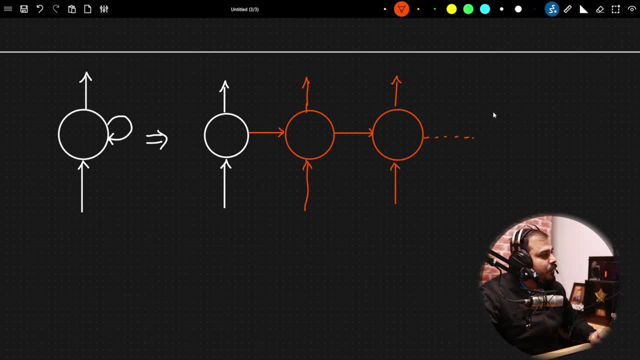 and one output And like this, it will be going to the next neuron, which will be having one input and one output. Then it will be going to the next neuron, which will be having one input and one input. Okay, Everybody. clear, Simple. 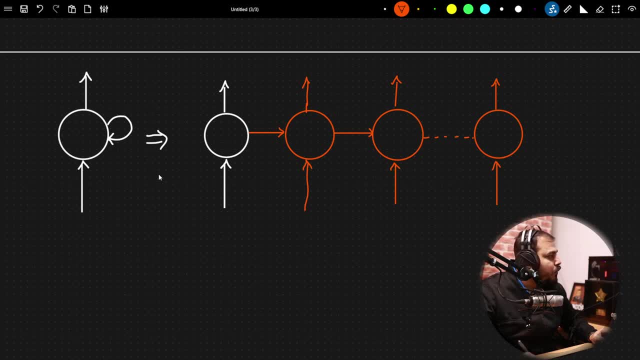 Okay, Now, as we go, What is this? What is this? You know The loop that you are doing: Every output is given to the next. Next, Every output is basically given to the same neural network. Right Now, can I say that this will work with respect to time stamp. 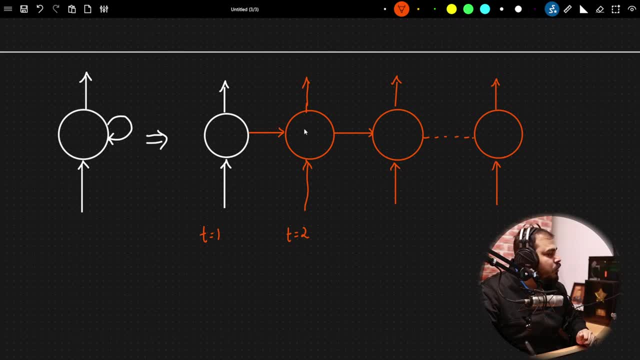 At t is equal to one. this output is going over here. over here. that at t is equal to 2: this is basically getting calculated. at t is equal to 3: this is getting calculated. at t is equal to n: this is getting calculated. yes or no? i hope everybody. 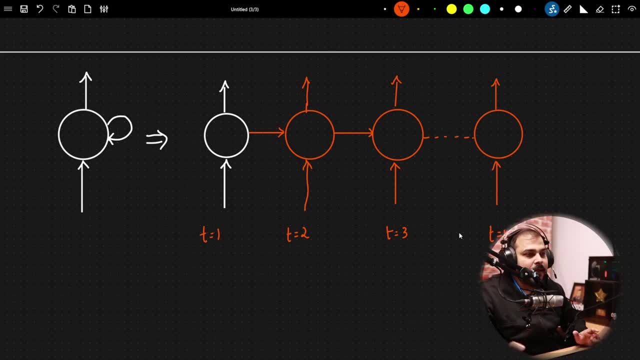 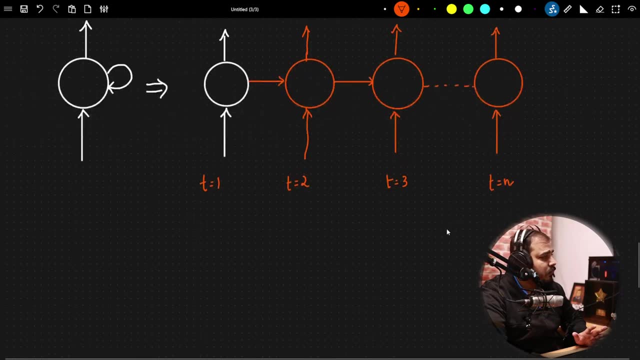 is clear with this simple neural network diagram: yeah, yeah, everyone, yes, everyone. so this is like: t is equal to n, right? so over here, what we are doing, we are just whatever output it is generating, we are giving it to the next time stamp of the same neural network. okay, same neural network, right, and? 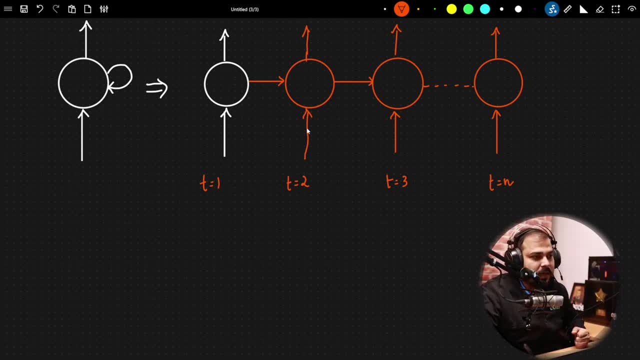 this can be one neuron and this can be 100 neurons. it is up to us. okay, everybody clear with this. can i get a quick yes, if you are able to understand till here, right, very simple right now. this is the entire process. okay, after this, what will happen if probably we have this many timestamp now, suppose? 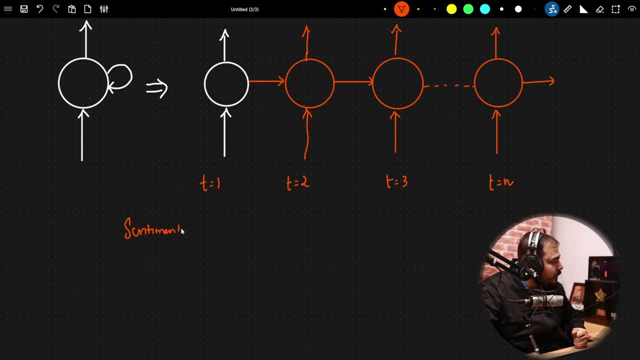 i say let's focus on solving one problem statement, which is called a sentiment analysis. what this sentiment analysis? either, let's say i have a sentence: okay, the food is good. right, the food is good. now, if i say food is good, let's say, with respect to this, my output. 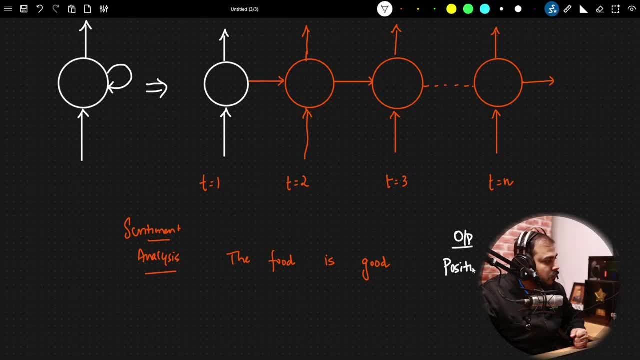 sentiment is positive, okay, okay. so my output sentiment is positive. so here you can see: yes, definitely it is positive. this is wow, amazing, okay now, okay. so, if you are able to do the simple neural network diagram, Now, how do I send this information? how do I send this information to our recurrent neural network? 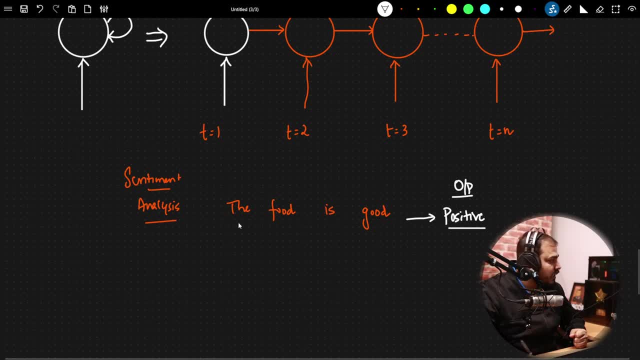 Very simple, we will try to see. So this word that you see, I will write it as x12,. let's say: Sorry, this is my first sentence. Let's say I am representing this by x11.. This is my x12 word, this is my x13 word and this is my x14 word. 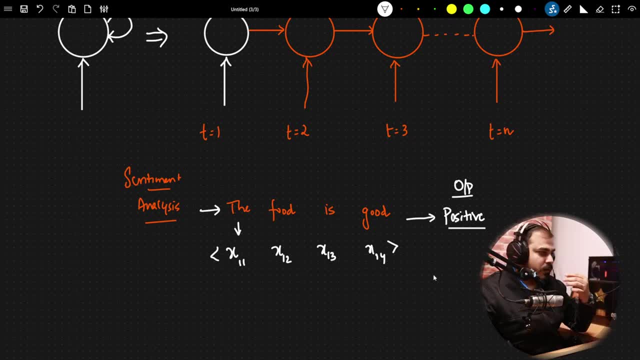 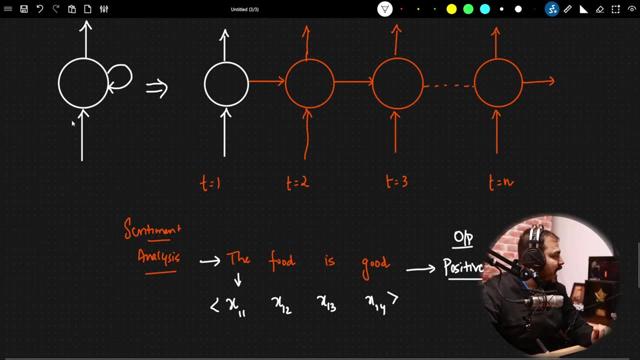 So here you can see, this sentence is basically having four words. Now, considering this neural network, at, t is equal to 1, which word I will actually provide, Because at a time I can only provide one input and I can get one output. 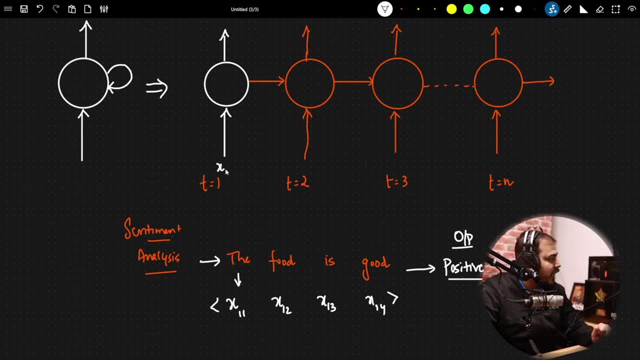 So in t is equal to 1, I will take up this first word and I will give it over here: x11.. Then something will happen over here. What will happen? Weights will get initialized. I hope everybody knows ANN. So in ANN, what will be there? 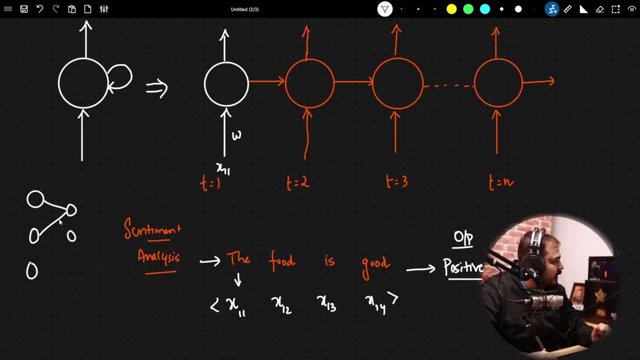 There will be an input layer and there is a hidden layer right. This will get connected to this. What is going to happen over here? Here weights are getting initialized right Here here all the weights are getting initialized. So similarly this x11, when we are providing, we will definitely convert first this x11 by using word2vec. 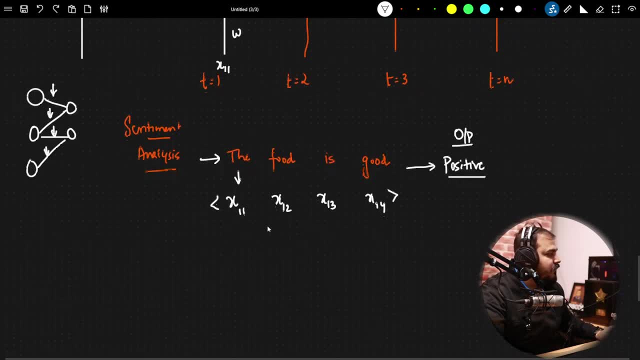 True or not? Okay, I hope everybody is able to understand. First of all, we will take this x11, we will convert this into, let's say, we are using word2vec. we will convert this into some vectors of dimension. 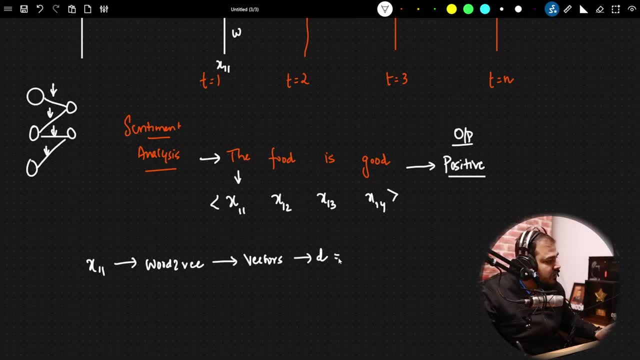 Let's say this dimension is d. Dimension basically means how many features- Let's say 300 features- are there? Okay, So we are going to get these dimensions and this dimension is going to get passed from here to this neural network, Right? 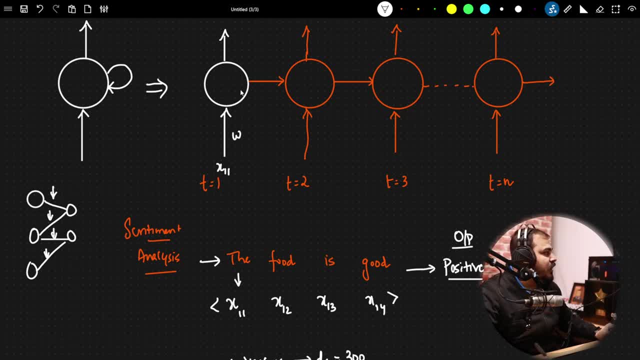 So here we are going to initialize some weights. Fine, So when this is done, some initialization will happen, I'll get some output. Then what will happen? This output will be sent to the next layer because at time t is equal to 2,. 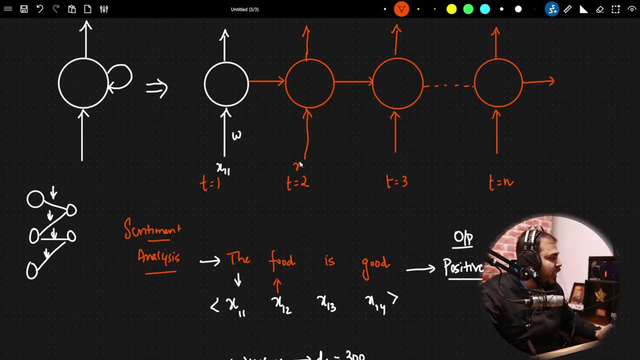 I am going to take this x12 word. So here I am going to get my x12 word, Everybody clear. So here I am going to get my x12 word. Then again, the same weights will come over here, right, Because weights will not get updated right now. 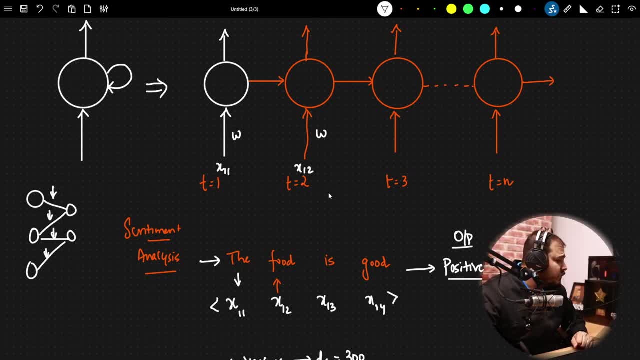 This is just a forward propagation. Similarly, at t is equal to 3, I will get x13.. So again, weights will come over here, x14.. Again, weights will come over here. Everybody clear now, Yes, Yes. 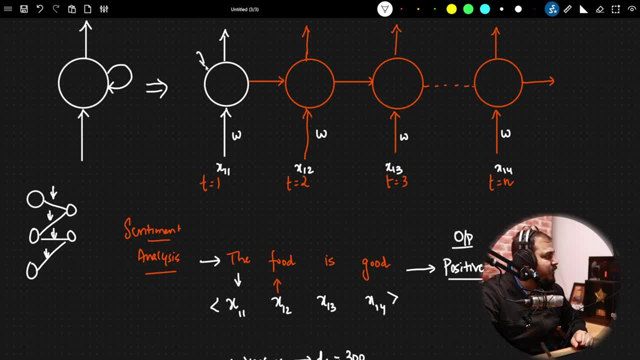 Yes, Yeah, internally, bias will get added, Bias will get added everywhere. Bias, bias, bias, bias, bias. Okay, Everybody clear How the weights is getting initialized. You know that, Okay, Weights, usually a lot of initialization techniques are there. 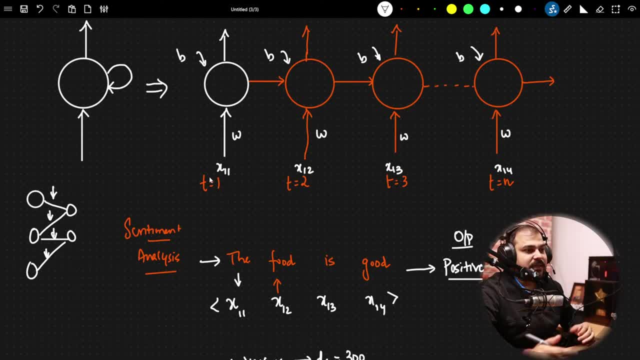 Okay, Perfect, Everyone till here and like this. Now, what will happen? Back propagation will happen. Forward propagation is here, Backward propagation is here. That I'll write in terms of equation. So this is the basic funda: how a recurrent neural network actually works. 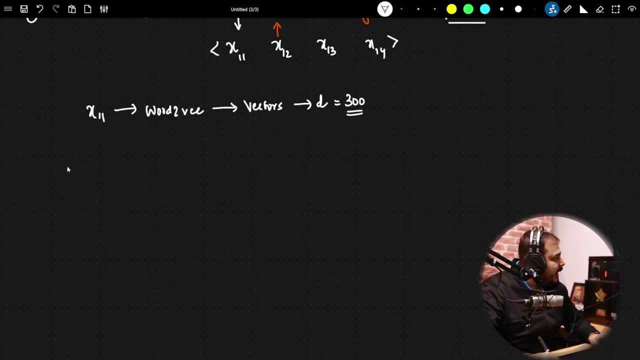 Okay, Now let's discuss about the types of RNN. Types of RNN, And I'm going to probably draw this in front of you. Okay, Suppose, first of all, there are multiple types. One is 1 to 1 RNN. 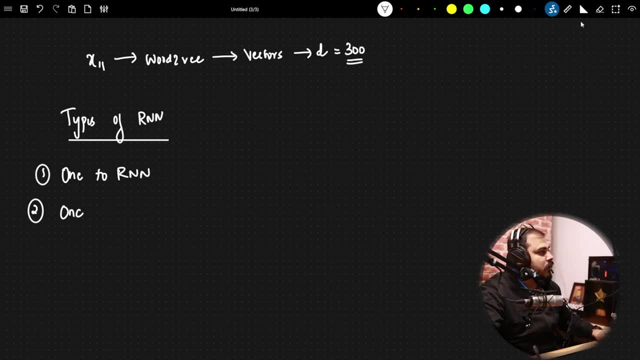 Okay. Second one is 1 to sorry. 1 to 1 RNN. 1 to 1 RNN. The second one is basically called as 1 to many RNN And we'll understand with respect to this use case. 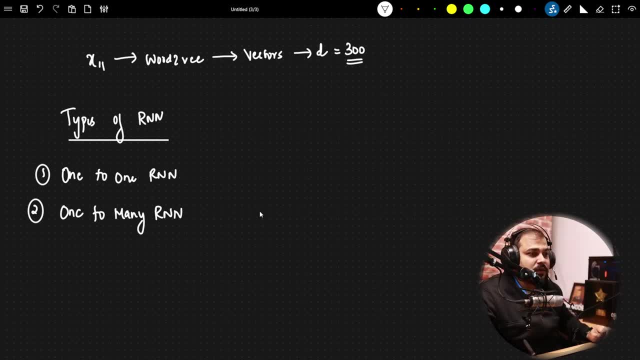 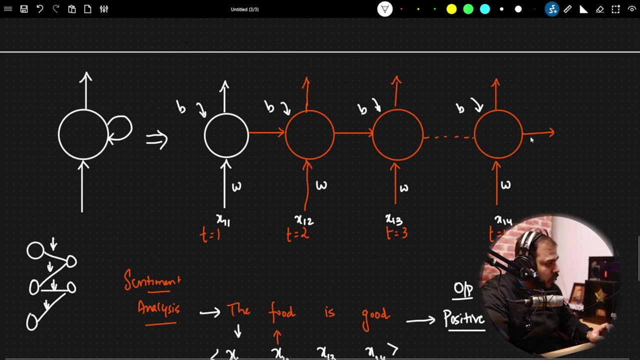 Okay, Is it the exact output passing to the timestamp, or some hidden state passed to the? I will again discuss about it. Just say that this output is again getting passed over here. Okay, I will talk about it. I'll come back again and I'll show you then. 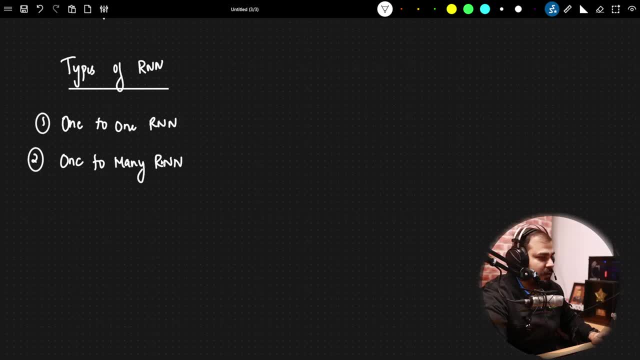 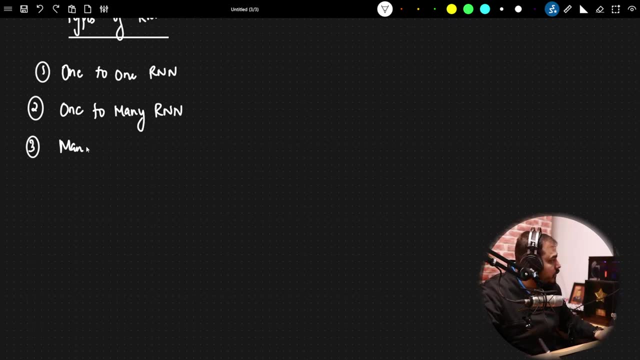 The entire equation, but before that, I really want to teach you what is types of RNN. Okay, Then the third one is basically called as many to 1 RNN. Many to 1 RNN. And finally, I have something called as many to many RNN. 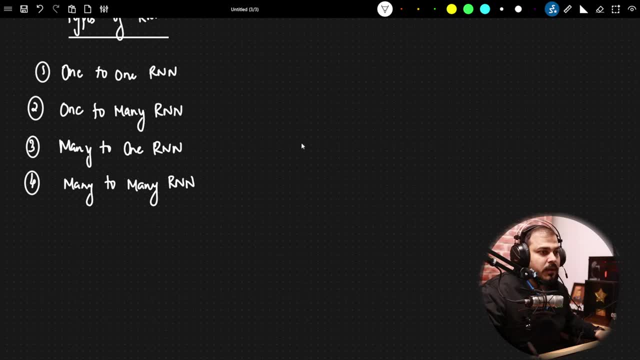 So these are the various types of RNN. Okay, The glove model will come. surfers, just give me some time, Okay. Okay, Let's see this. Suppose this is my neural network. right, I have one input, I have one output. 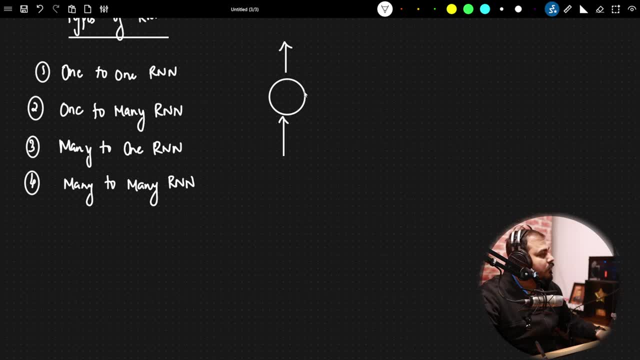 Okay, And let's say over here, the focus is that if I try to expand it, if I try to expand it- and obviously in RNN I have this, So I will start this. So here you have an input. Instead of retrieving the output here, we will just send the output to the next one. 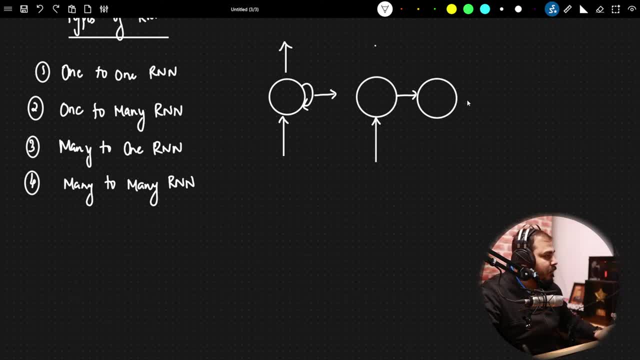 From here again, input will be taken or no input will be taken. Okay, Let's say again: the output is sent to the next one, Right, Again, the next output is sent to the next one, And finally, I retrieve the output over here. 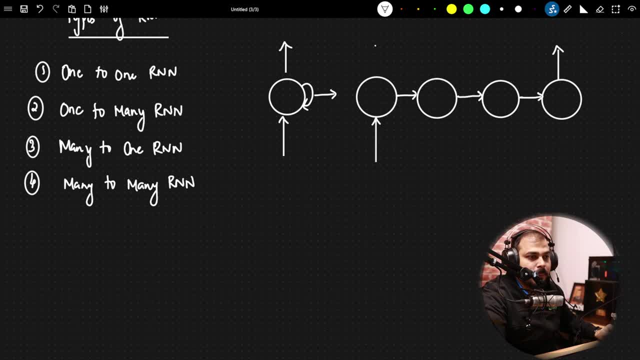 Okay, I retrieve the output over here. Everybody clear, Everybody clear. So in this particular case, do you see, I am giving only one input and I'm getting only one output. Yes or no, Yes or no, Yes, Yes, everyone. 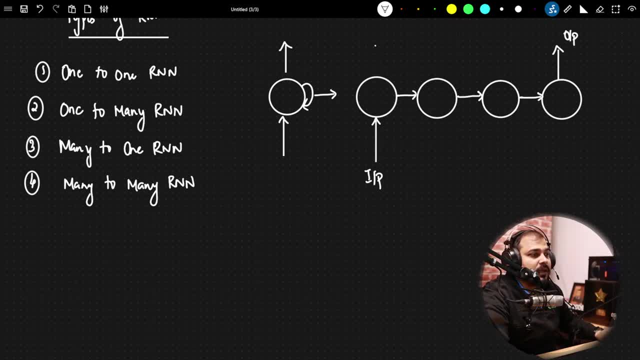 I hope everybody is. I hope everybody is able to understand here what I am actually talking about Here, what I am actually specifically doing. I'm giving one input and I'm getting one output, Yes or no? Yes, In the architecture, here also I'll be getting an output, but I'm not retrieving this. 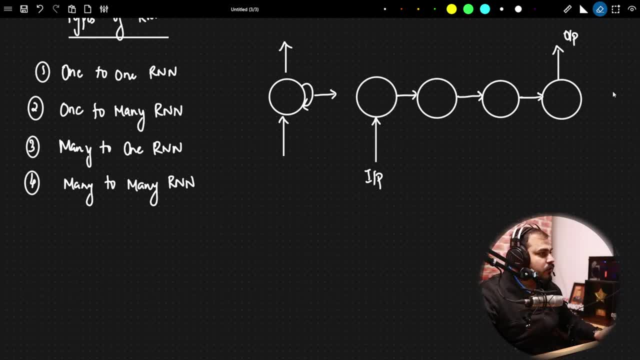 I'm just removing this output. I don't want it, Okay. So in this particular case, we basically say this as one to one recurrent neural network: Okay, One input and finally one output. Okay, Now let's go ahead and understand the second one. 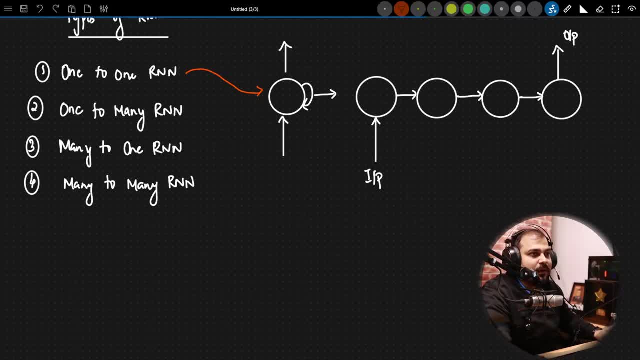 What is one to many? Now, in one to many, there will be obviously one input. And what is the example for this? This example can be anything right. You can also use image classification. using this, You can do image classification right. 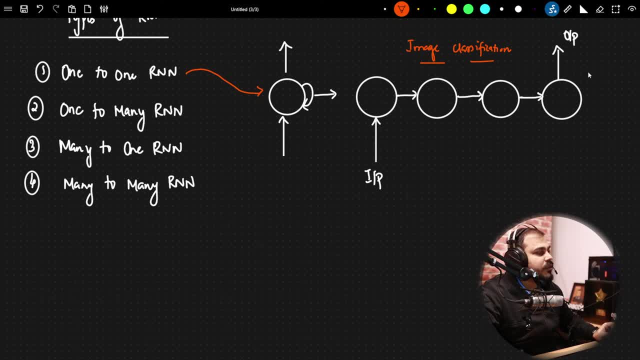 Using this one image you'll be giving over here and one output. What is the class type you may get over here? You're not CNN. With the help of RNN also, we can do image classification. Okay, I'll show you one application, but again right now not that important. but just understand that if you also probably try to see it, 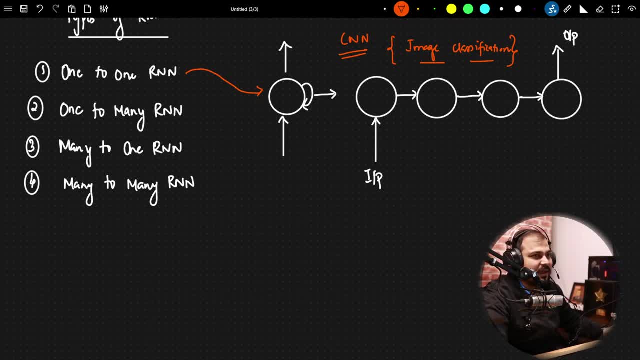 how this thing will happen. I'll just tell you, probably in some time. Okay, So one to one, uh, let's focus on this. one to one, uh over here. Uh, image classification can be a very good example, Okay. 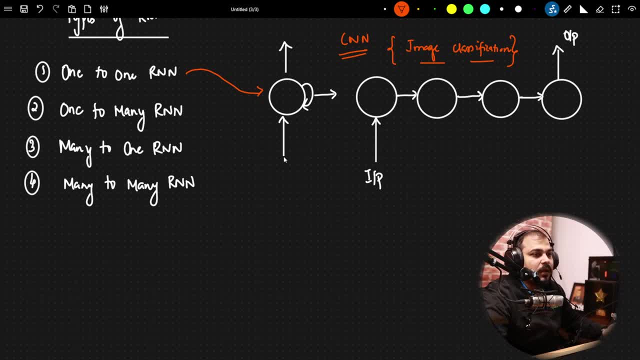 Now let's go to the second time. One to many. Okay, Now one to many. how does it look like? Okay, Everyone just see over here, focus over here. This is super, super important. Uh, these are all things you should know. 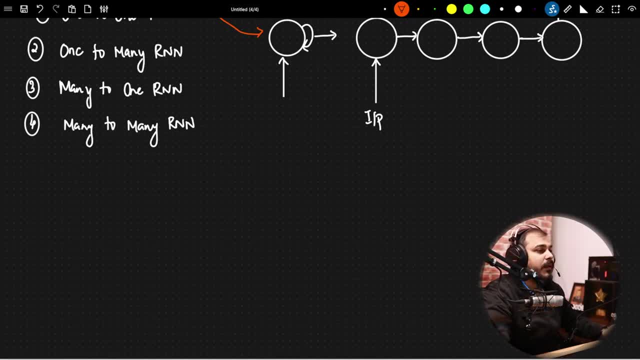 Then only you'll be able to understand well as we go ahead. Okay, Now, one to many, Now one to one, basically one to many. So second type what we are going to discuss. Okay, Just give me a second. 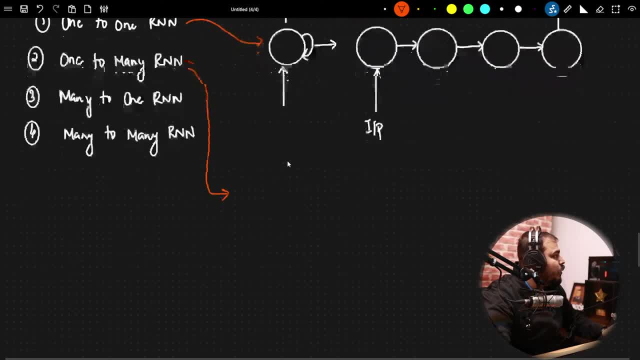 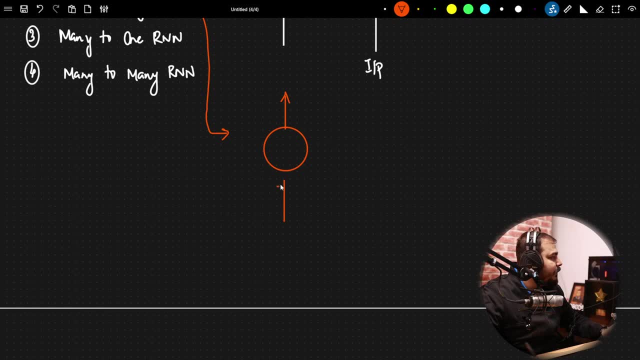 Okay, Just a second, guys, One to many. Okay. So here is my neuron. So in one to many again, what will happen? So this will be my representation. But if I expand this, the first thing is that I will be having one neuron like this: 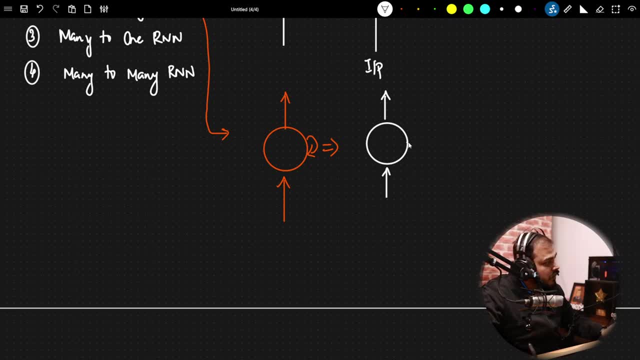 This will be one to many, Okay, And then this will go to the next one, So I can take out this specific output Also. I can take out this specific output Also. I can take out this specific output also, And like this, I can take out this specific output. 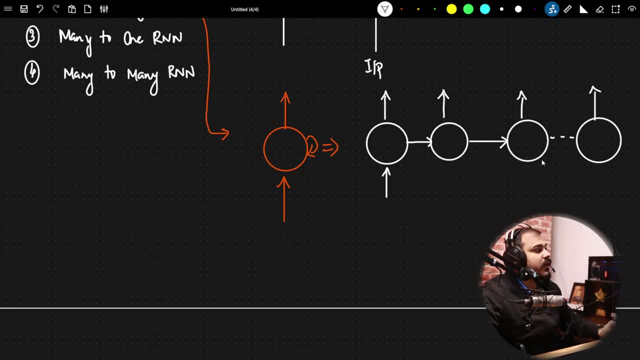 Also, everybody clear, Everybody clear with this. Yes, So here I have just one input and I have many outputs. I have many outputs. Everybody clear. I have a single input and I have many outputs. Okay, So each and every layer output can also be taken with respect to timestamp. 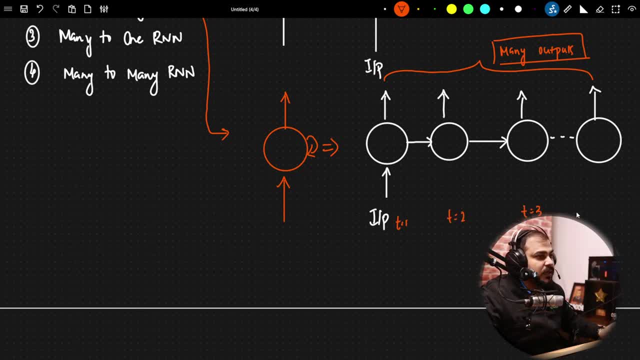 Like this will be: t is equal to one, T is equal to two, T is equal to three, T is equal to four. Everybody clear with the second type right: One to many, Yes, Yes. How many iteration does it take to get the desired output? 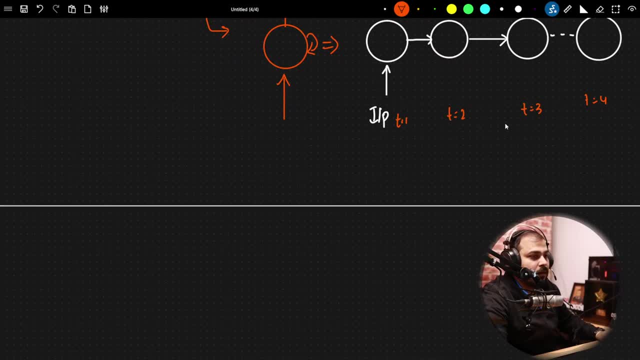 That depends on the loss function. We'll discuss about this. Okay, But I hope everybody has understood what is one to many right Now. can anybody tell me about some of the examples with respect to one to many, Anything that you have in your mind? 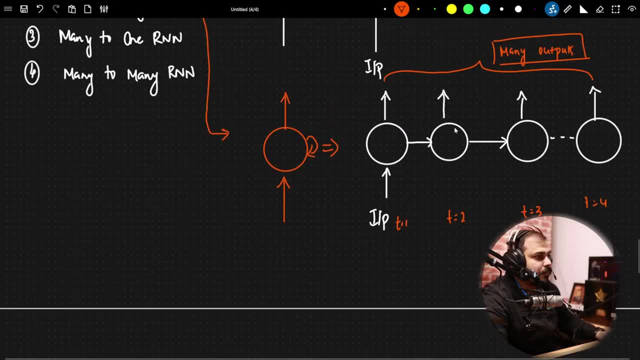 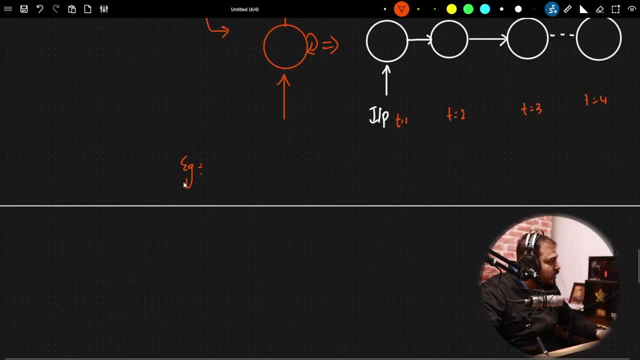 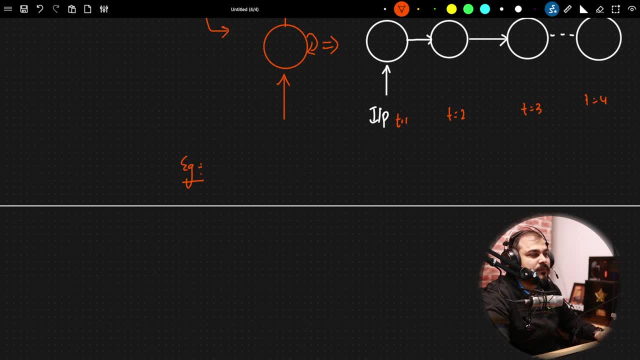 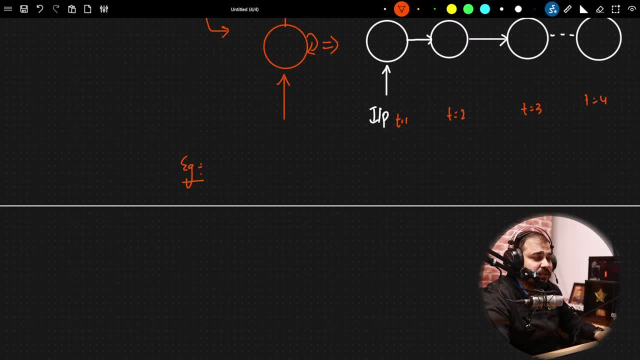 Any examples? Music generation, Okay. Music generation, Yes, Music generation can be a very good example. So here I have specifically called as music generation, generation in music generation what we do: we give one input and then later on the further music can. 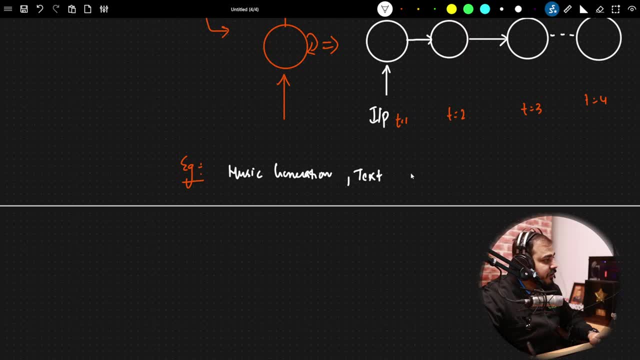 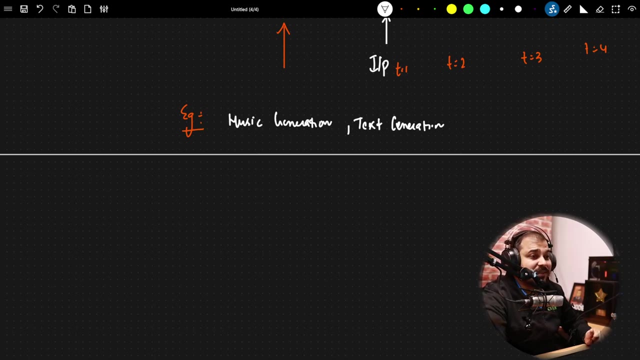 be actually calculated right. so i can also say text generation right. text generation is also one kind of example. i give one text over there and automatically all the text will basically get created right. any more example: one too many, anyone one too many? yeah. google search suggestions: okay. 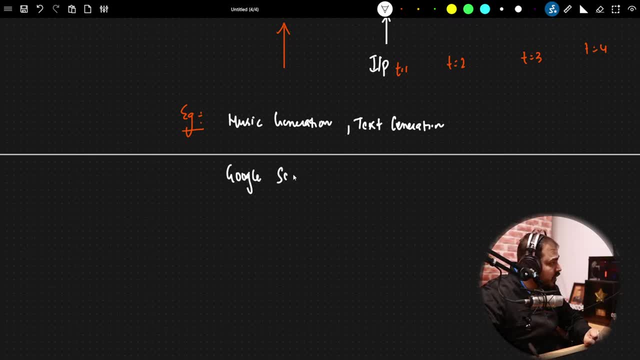 yeah, perfect. google search suggestion is also a very good example, because once you write an input, multiple suggestions can be given to you right, so this all can be amazing. you know examples? movie recommendation: movie recommendation is also a very good example, because based on that, you will be able. 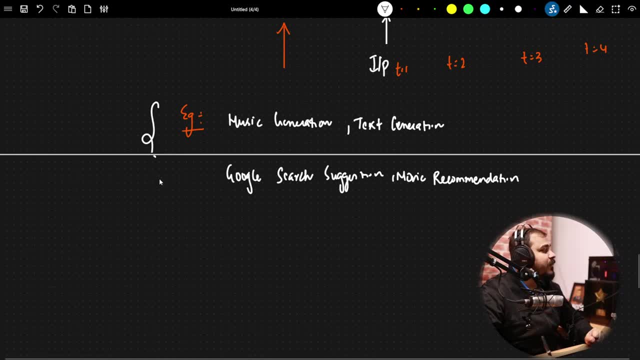 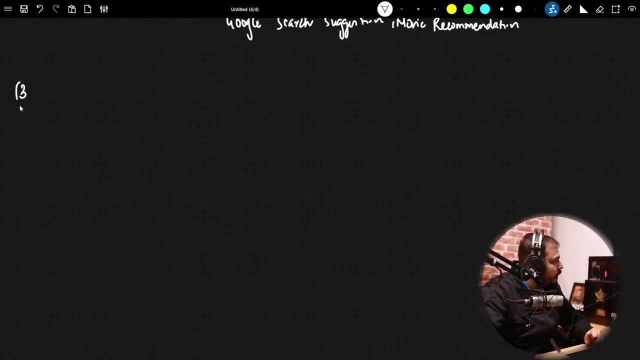 to get it right. so see, so many different, different use cases have been used with respect to this kind of architecture. okay, now let's go to the third one. third one is basically many to one. now can anybody tell me what is the example with respect to many to one, in many to one? what will happen? so i will. 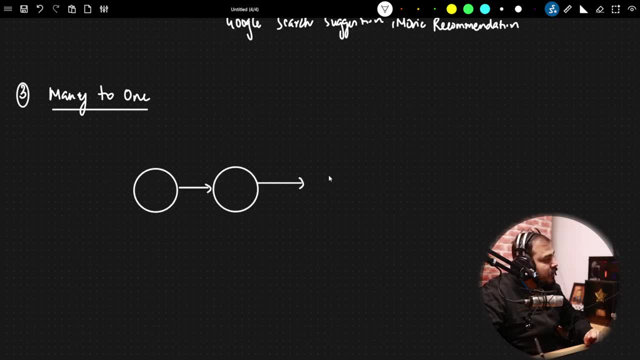 have like this, i will be having like this, i will be having like this, many to one, what may be the example, and this will be my one output, and here i will specifically be getting continuous inputs. okay, why? this can be any simple sentiment analysis. right, there we go. 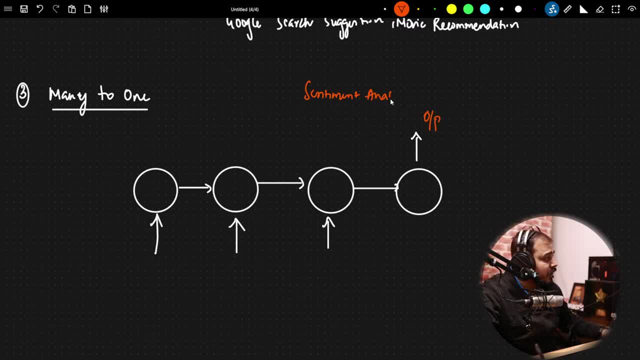 give multiple words and finally my output is yes or no. sentiment analysis: right, sentiment analysis: uh, can i say that okay? uh, from here i can also predict: probably the next day sale. predict next day sale. this can also be an example by taking the previous data, predict next sale to a next sale day. 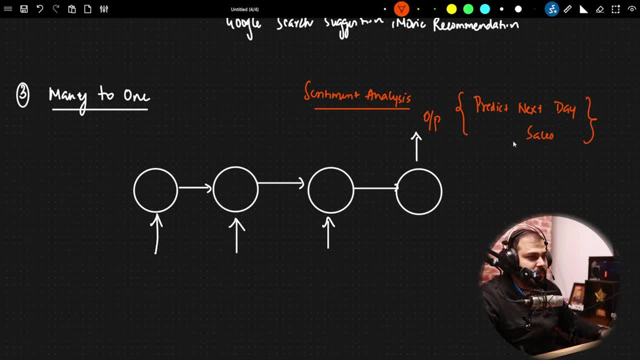 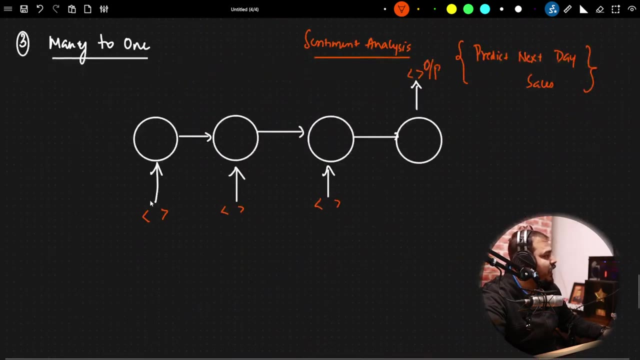 right next day sale. so this is also there as an example. uh, you can again see a lot of things with respect to that. here we are providing multiple inputs and here i'm getting one output. okay, so super important, super easy. so this is with respect to many to one, and now coming to the many to many. 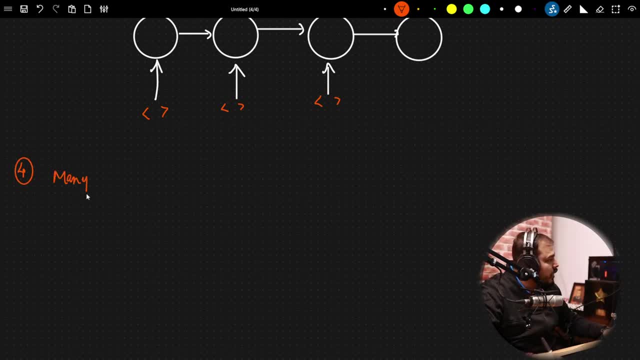 can anybody tell me many to many, which is the best example? many to many, many to many is a simple way where we specifically get one input, get one output and then i go over here and i probably get one output, and then i go over here and i probably get one output and then i go over here. 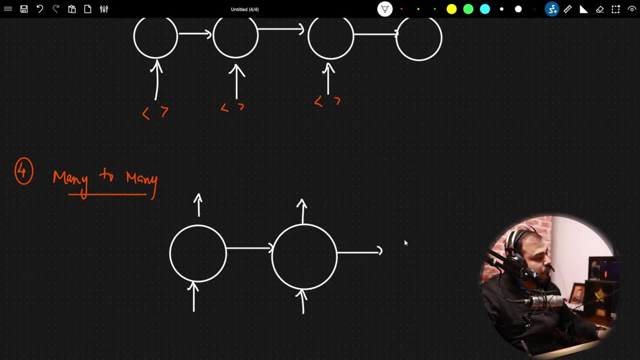 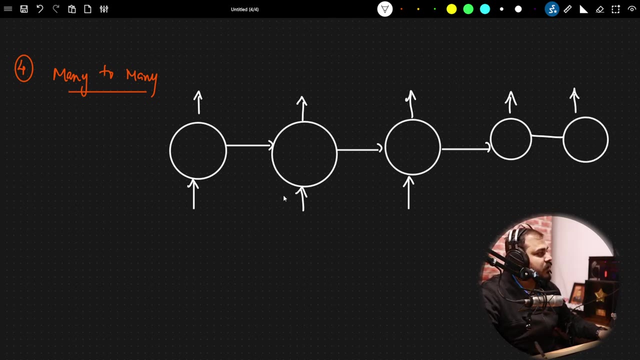 one input, one output right. like this, many to many will definitely be there right. so i can probably define: like this right. so in this particular case, the best answer will be: language translation right. language translation okay. or second example: question answering perfect question. answering perfect question. answering chat bots right. 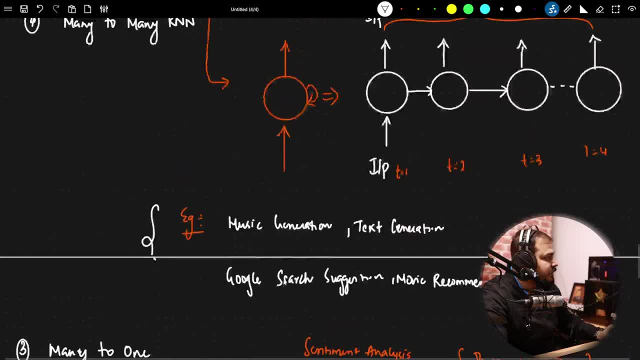 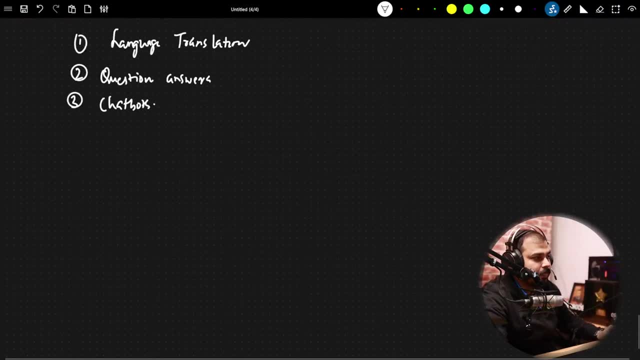 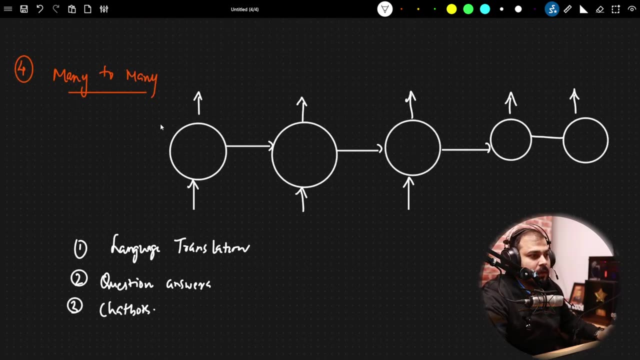 all these things will be the perfect examples for all these things: everybody clear. so how was the explanation till now? yeah, good, yes, clear. if you liked it, please make sure that you hit like, subscribe my channel. and don't forget to subscribe krishna kindy channel, because i am also coming up. 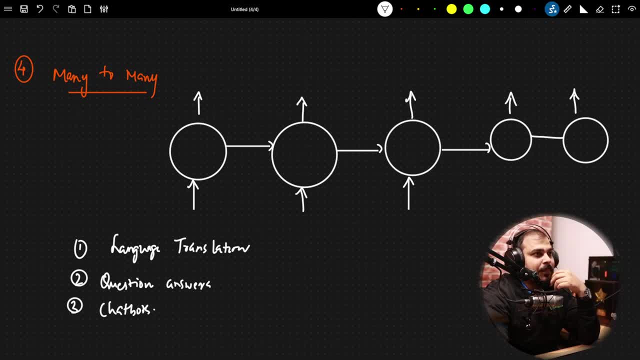 with lot of hindi videos related with data science. okay, and this can be an interview question to you. you know they may ask your use case. they may say, okay, what is this kind of things tell me? okay, what is this kind of things tell me? you know they may ask you anything, so always be ready to answer. 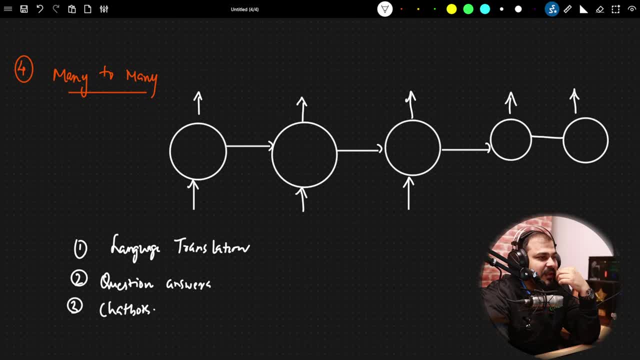 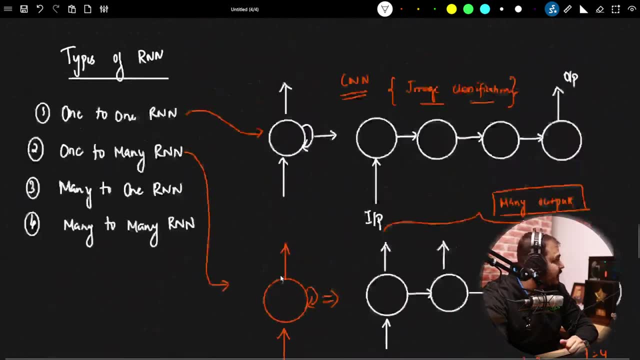 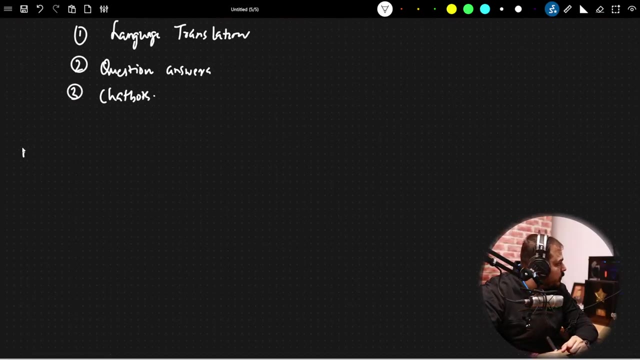 those kind of questions. they may ask you anything at any point of time. you know. they may say: okay, what is this example, what is that example, you know? okay, perfect, okay, now let's go with respect to the forward propagation. okay, so now my topic will be something called as forward propagation. 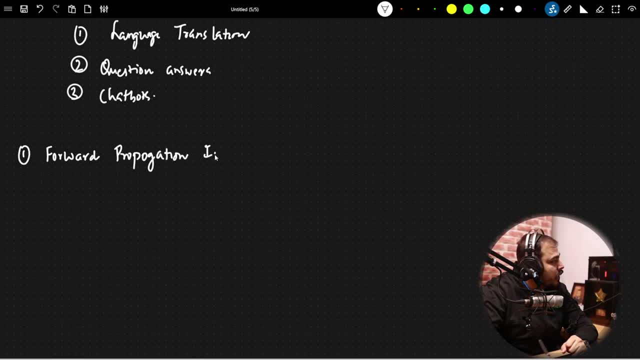 in rll, because whenever we learn about deep learning, right, there are two things: one is forward propagation, one is forward propagation and one is backward propagation- backward propagation, right, so this two, we are specifically going to discuss how things will basically happen. okay, and say at the end of the day, any complex problems that you see right now. 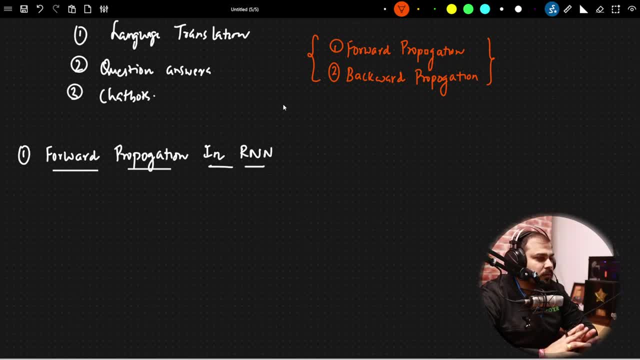 that are existing, like this one, for example. you have a problem, you have a problem with problem. you have a problem with csos and you have a problem with the thing that you're analyzing. that has been solved by google, you know. that has been solved by facebook, you know, specifically, 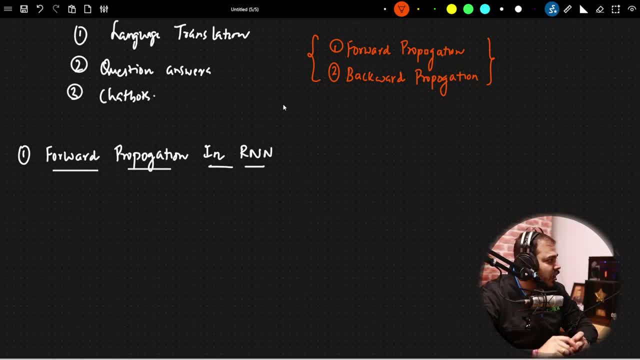 with respect to nlp or text data where sequence is involved. i'm not saying that rnn is only used for working with text data. rnn is used for working with time series data also. okay, so time series data also. it is super important and will be useful when you are specifically working with rnn. okay. 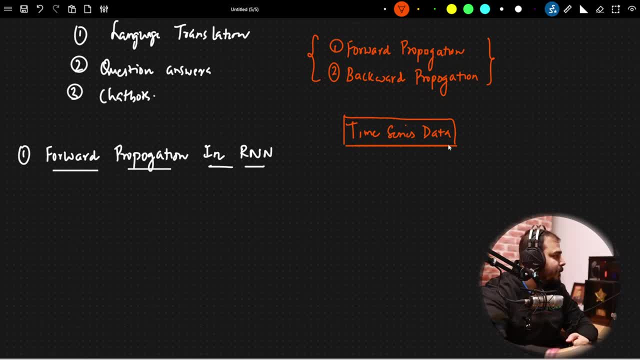 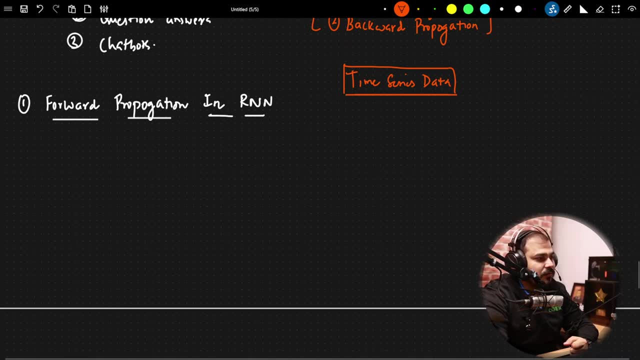 and you know this is it? so let's go ahead and discuss about the forward propagation. okay, and we'll try to understand what exactly is forward propagation and all. how does forward propagation actually happens in rnn quickly? first of all, we will draw a diagram and we'll try to understand. 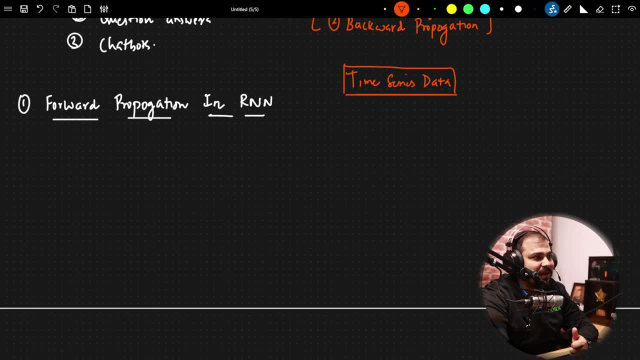 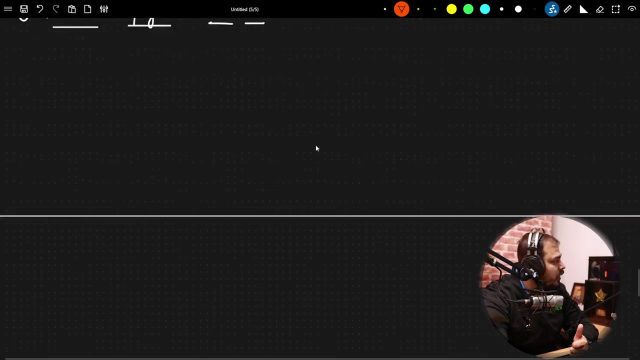 anyhow, if you don't understand something, i'll always be there to help you out. okay, so quickly, let me do one thing. okay, so let's go ahead and understand about the forward propagation and let's try to understand: how does forward propagation basically happen? okay, so for this i will just take a very simple 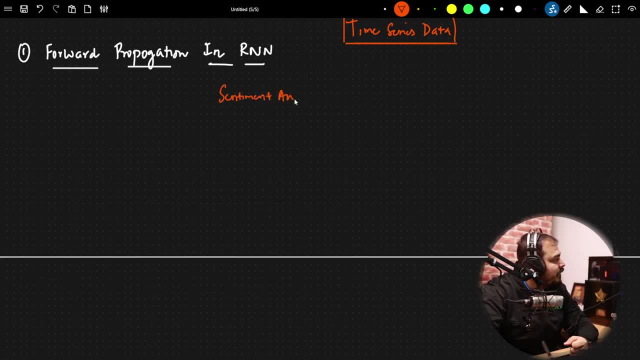 example, which is called a sentiment analysis. now, whenever i talk about sentiment analysis, you should know it is nothing but many to one rnn. okay, many to one rnn. you can define your own rnn however you like, but i am really much focused on many to one. okay, right now, many to one. you can also do with respect. 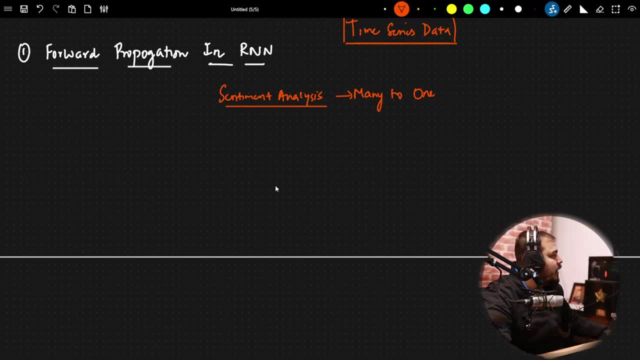 to many to many and whatever things you actually write. okay, now, with respect to many to one, let's consider: this is my neural network. okay, i have a specific input, i get an output and then i probably go to the next neural network, or this is my input output, but since i'm saying many to one, so i'm not. 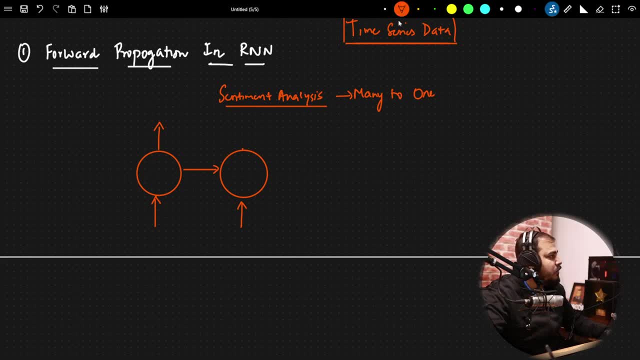 going to consider this. okay, but anyhow, the next, whatever output is generated, we are focusing on transferring it to the next neuron. okay, so here also one input, and like this, i will go and define one more, and this may be of any size you like. okay, so let's say one more, i'll define, so that. 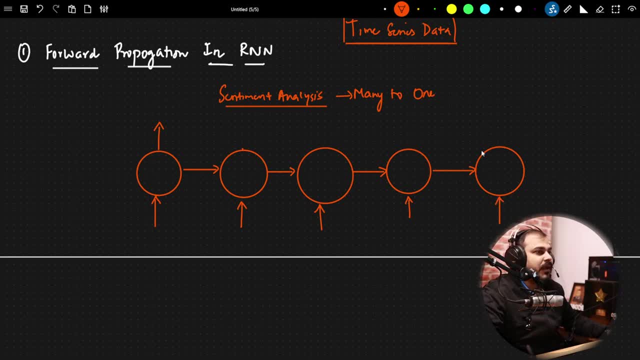 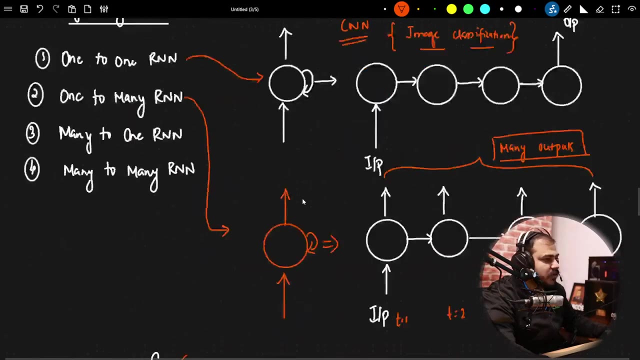 maximum size is basically getting covered, okay, and after this, uh, you know, i specifically get an output over here. okay, now let's say this is my text. as i said, uh, the text can be anything. i have taken an example with respect to the food is very good, the food is good. how many? four are there? five are there? the? 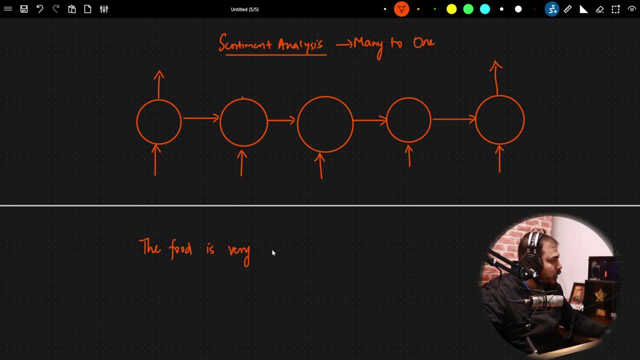 food is very good, right, and with respect to this, my output is positive, right, because this is a positive sentiment. so in this particular instance, this, i will write it as x11, x12, x13, x14, x15. now when i say i'm passing x11 over here, that basically i'm passing in the form 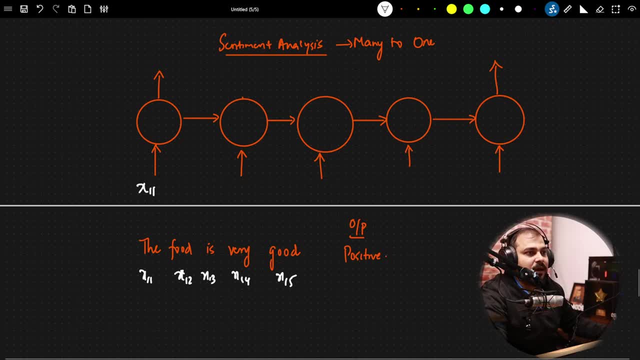 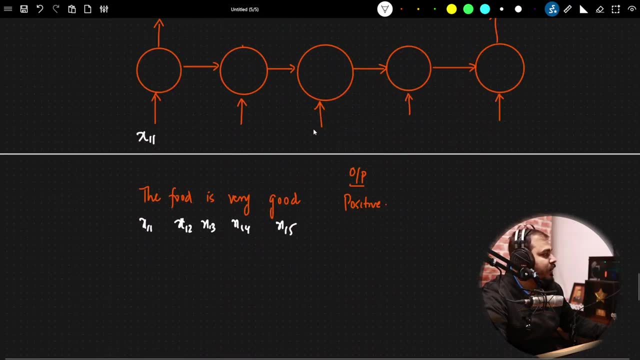 of vectors. okay, always remember this. you may be thinking how you know how this thing will actually happen now, right now, i'm just focusing on forward propagation. okay, so x11 is going over here, then what we do? we initialize weights over here. can i say, here we are, what kind of operation will? 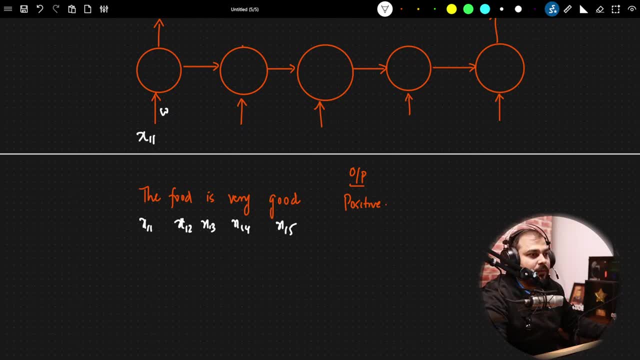 specifically apply. you know, between this x1 and w11, one, one specific operation we will probably apply right in forward propagation. we are just going to multiply the inputs and the weights right. so over here, suppose, if i'm getting this o1, this o1 and this output will be almost same right. so 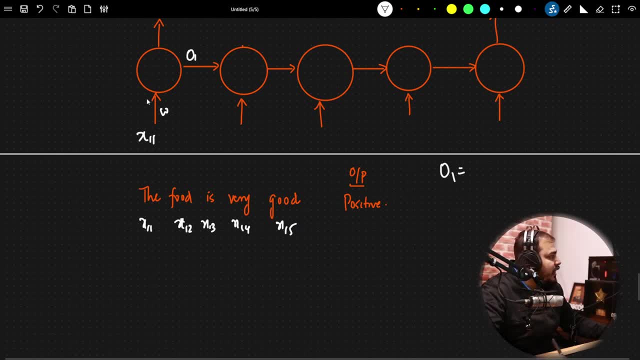 the first operation of o1 is nothing but this neural network. can i say this is a function, because one multiplication will happen, multiplication between x11 and w right. so can i write x11 multiplied by w right? so this thing and i'll be getting o1 right. very simple, very simple. i've not done anything, i've. 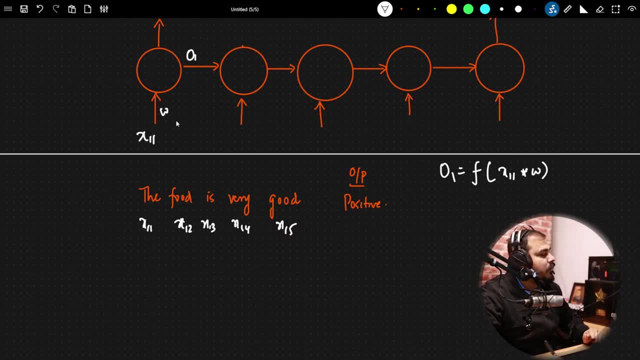 just done this matrix multiplication of x11 with w. x11 is in the form of vectors. okay, and this w, that many number of w based on the neuron- how many neurons are there? we are going to just multiply with it. then let's go over here. now, when i here, i'm just going to pass x12 and again w will be. 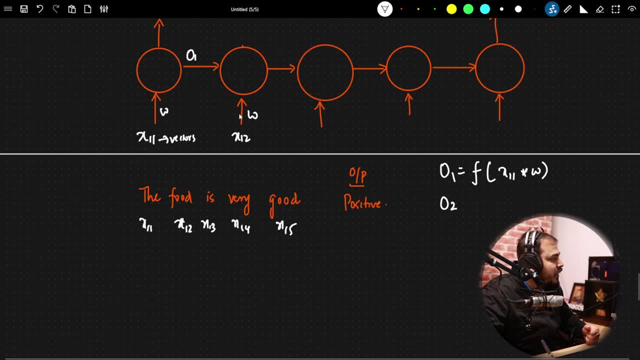 used over here. but since o1 is there, this o1, this x1 and w1, and this neuron is also dependent on o1, right, because this information is again getting passed over here. so here i'm going to initialize another weight, that is w dash. let's say this is another weight, right, and i have to make sure that. 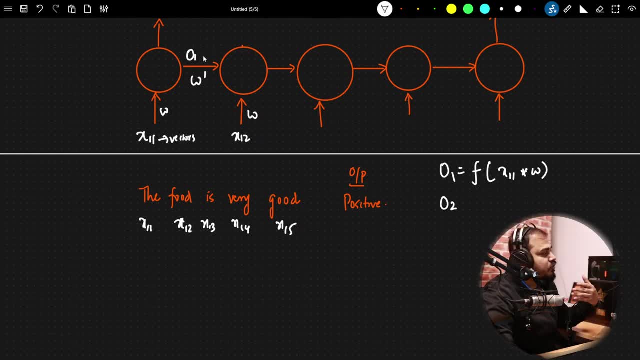 when i am multiplying. this i also needs to get added to this, because i'm also dependent or this neuron. this neural network is also dependent on the previous input. so here what i'm going to do: i'm going to create a function. first, multiplication will happen with. 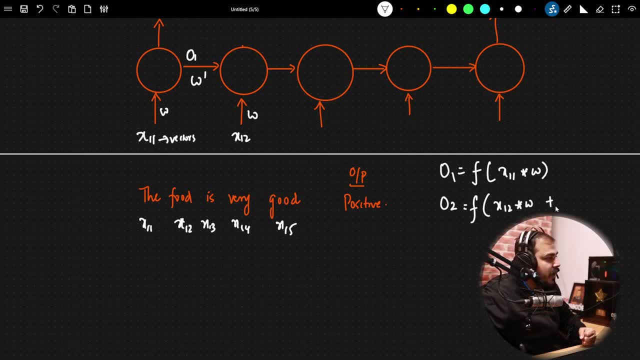 x12 multiplication multiplied by w, and then an addition will happen with o1 multiplied by w1. is it clear? everybody? yes, i hope everybody is able to understand. or this can be like a dot, dot operation. yes, dot operation, element file multiplication. okay, so i hope everybody is clear with respect to this. can? 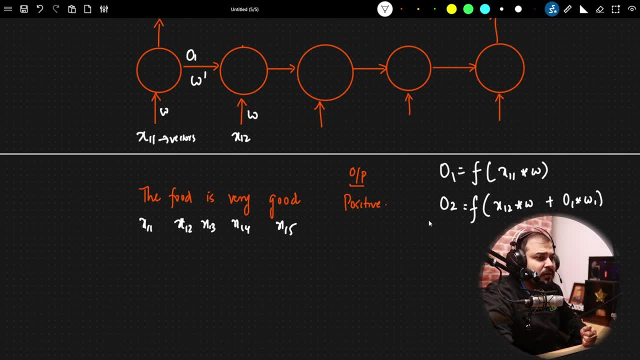 i get a quick yes, how it will identify the end of sentence in proper forward propagation. so when i will do practical application there will be something called as padding. so i'll show you that how to do it. don't worry about it right now i'll do of specific padding. you know some size specific padding and then we'll try to. 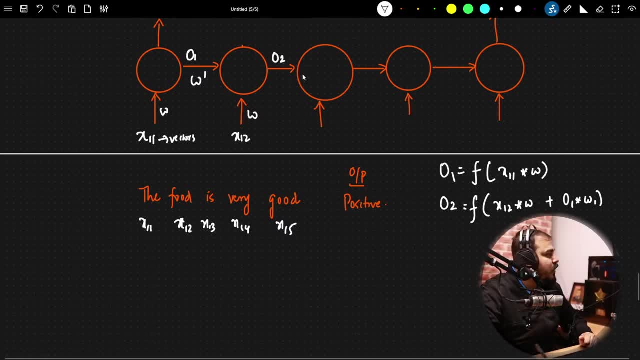 understand. then again, uh, over here i will get o2. now o2 will again get initialized with some weights, and here i'm going to pass x13. this will be width, then o3, then again weights, then x14, uh, w, then o4, and this is w, dash, w dash, and finally i will be having x15, and here i'm actually going to get it. 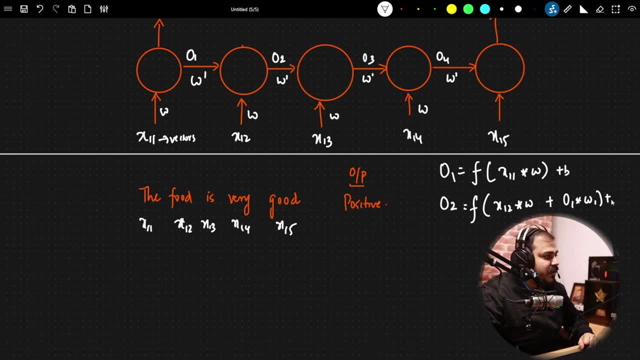 okay, don't worry, after this we specify the condenser, because we pantalla will be just like the temporary. ok, after this we specify the condenser. ok, add a bias everywhere. okay, bias, not that important right now, but let's focus on this forward propagation right now. but anyhow, you can add bias wherever you want. okay, so I'm just going to rub. 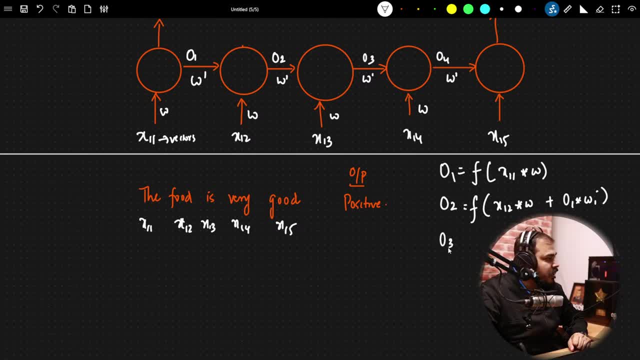 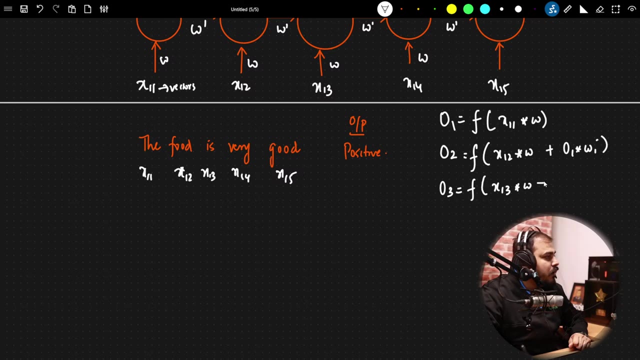 this. so let's focus on this operation, which is super. now, o3 will basically say what o3 is dependent on two things: this two and this two. so I will write a function of a function of uh. you can see x13 multiplied by w plus o2, o2 multiplied by w, dash right. so this will say specifically: be the. 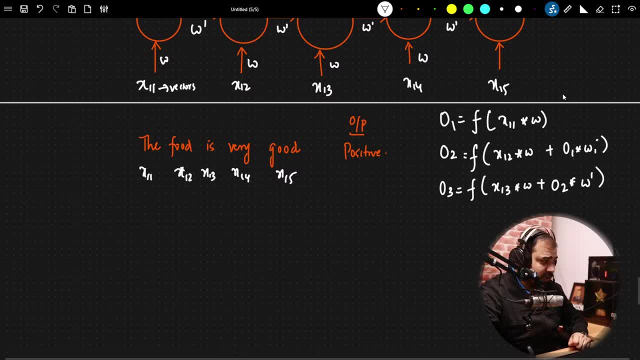 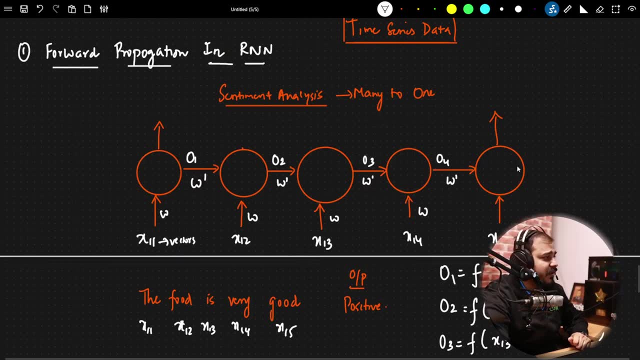 operation with respect to o3. now, like this: all the operation will continue and it will go till the end stage, right till this specific stage, okay, till the end. and you can continue writing this specific equation like this. so, finally, in the output right, we apply- since this is many- to one: 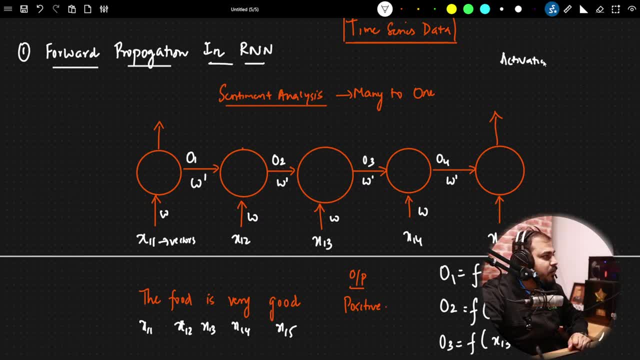 in many to one. which kind of activation function we can apply with respect to the output. many to one. which kind of activation? since, if this output is a multi-class classification problem, we specifically apply sigmoid right- this I have already explained in my deep learning live sessions- right when so not not multi-class? 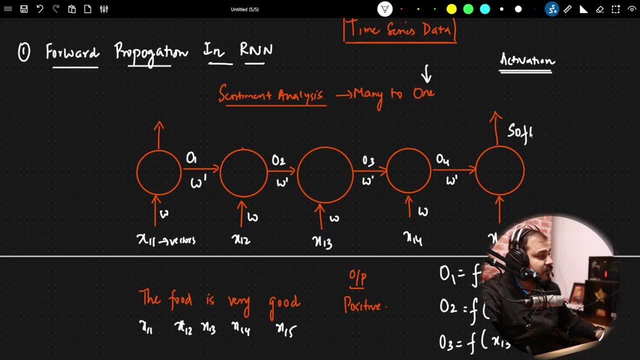 classification. if it is a multi-class classification, we basically apply soft max right. if it is a binary class classification, we apply sigmoid right. so for this, for multi-class, we apply this, for binary class classification, we apply sigmoid right. so either of this, we specifically apply this two. 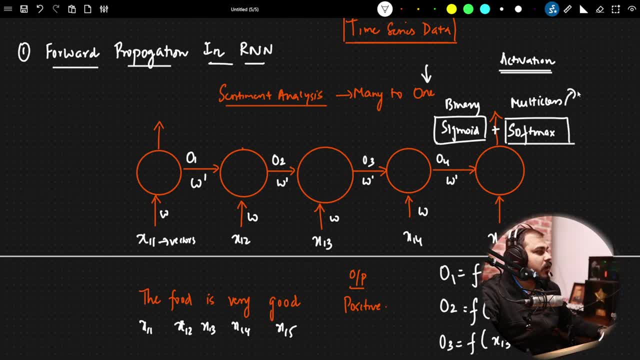 operation: either this or this, and finally I get what y hat right, I finally get y hat. after this, this output is nothing but y hat. okay, so this is, with respect to the forward propagation: everybody clear, yeah, yeah, everyone, yes, yeah, I hope everybody's clear. so I will see you in the next video. bye, bye. 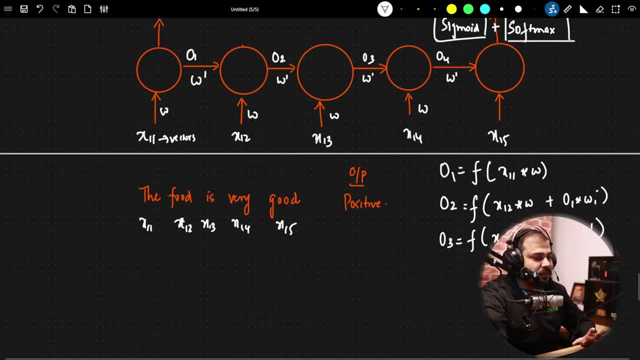 with this super important forward propagation. everybody has understood and we have focused on how forward propagation is going to happen right now in the backward propagation. what we focus on. once we get y hat, I'm good, but I will also be having my original y value, so I will try to. 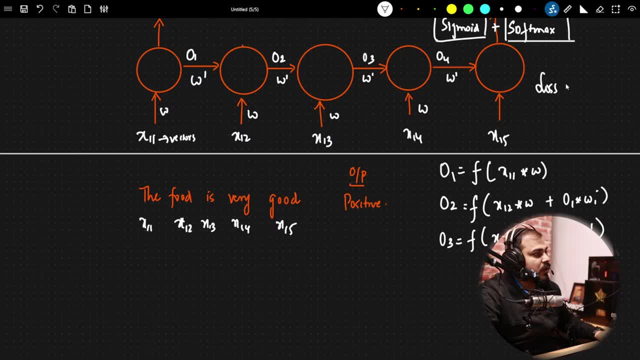 calculate a loss function. now, a loss function, let's say I'm going to use a simple loss function where I'm subtracting y and y hat, okay, and there are different type of loss function which I have again explained in different different laws. and I'm going to use a simple loss function where I'm subtracting y and y hat, okay, and there are. 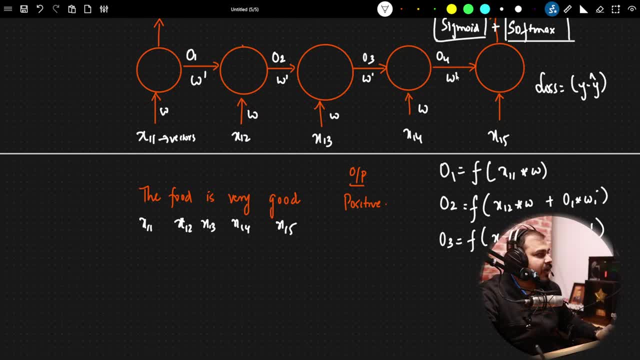 different type of loss function, where I'm subtracting y and y hat, okay, and there are physical loss function over here and, with respect to this, I'm going to update all these weights. right, I was just going to update all these specific weights, these weights, and this is going to happen with respect. 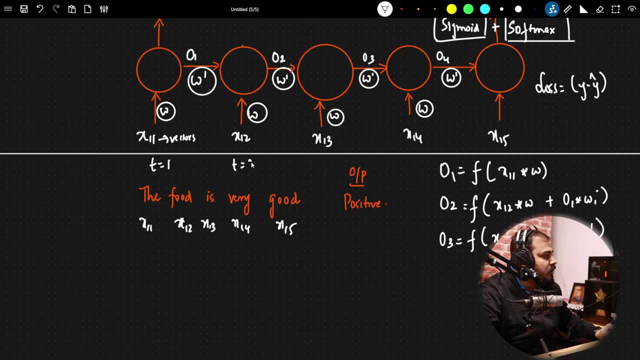 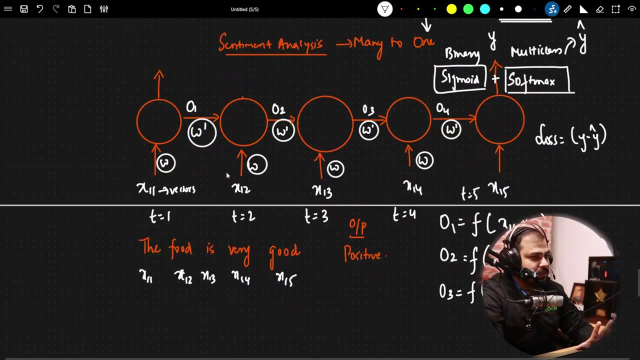 to all the time steps. so this was: t is equal to 1, t is equal to 2, t is equal to 3, t is equal to 4 and this is right. everybody clear can get a quick yes. how does the back propagation happen? i will try to show you that in the next class, but I really wanted to cover this. 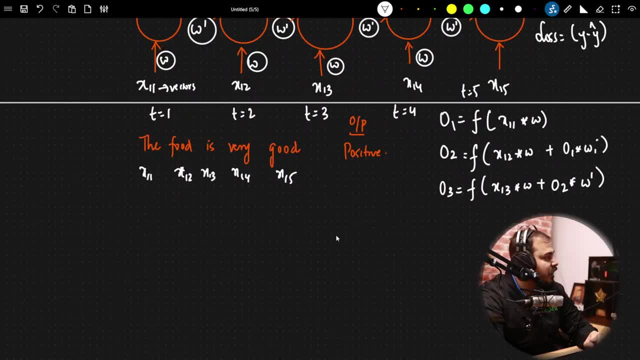 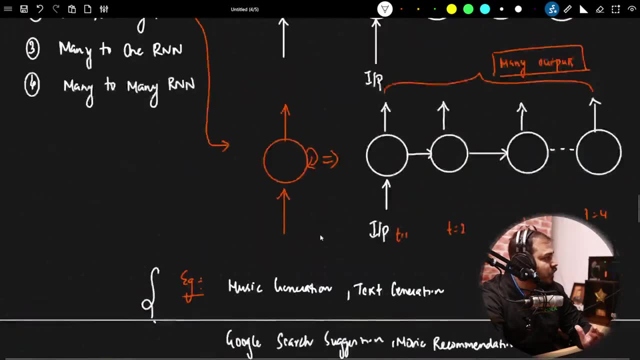 forward propagation and all do the same thing, this time, instead of exactly going to show what troublesbug is- and we have time, uh, because it is a one hour session. uh and uh till here. i hope everybody got an idea. can i get a quick yes, if you are got an idea till here. so, overall, what we are going to do in the 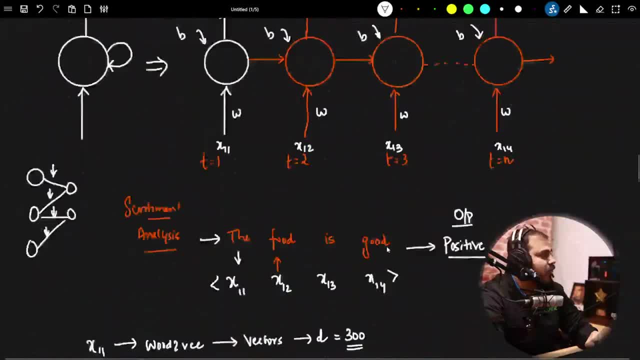 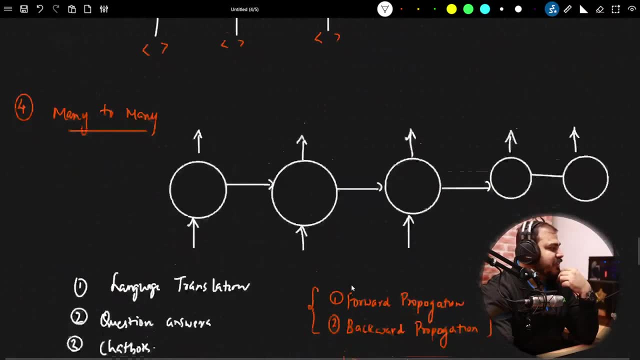 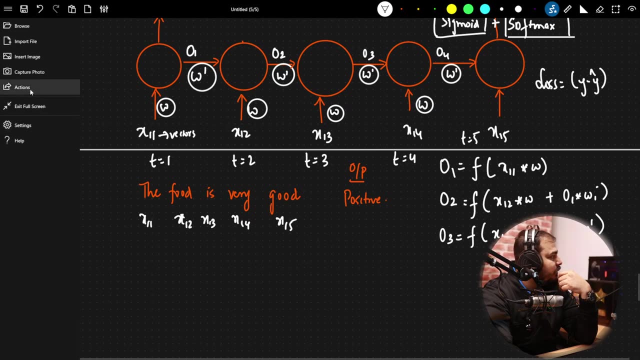 next class, also, after understanding backward propagation, we are going to solve a practical problem. i really want to cover each and everything you know, each and everything with respect to the rnn also, so that everybody understands from basic, from scratch. that will actually help you to gain your confidence right. so, overall, i hope you liked it. i'm just going to make sure that convert this. 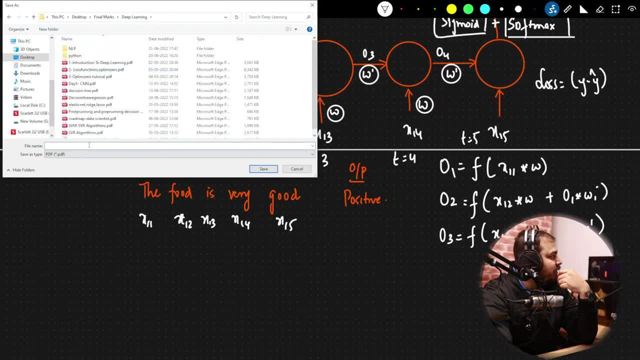 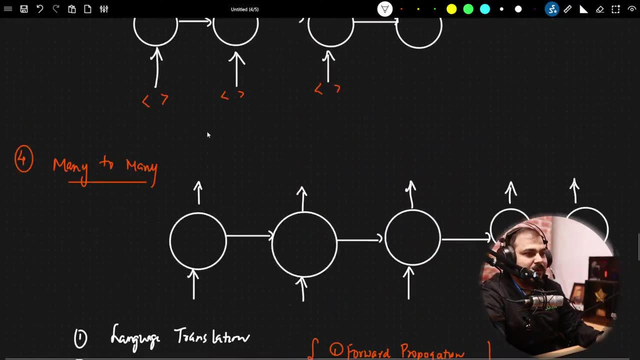 into pdf, okay, and this pdf will be shared with all of you. please make sure that you join the community link that is given in description of this particular video. so this is nlp day six, okay, and i have created. i hope everybody is liking my handwriting and you are able to understand. 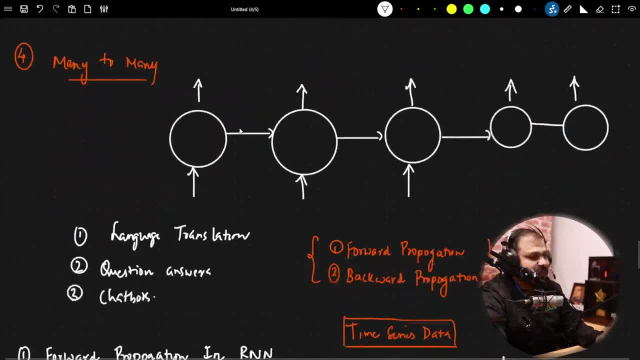 everything that i'm drawing and teaching. that is the amazing thing. when i teach, i always try to do it in a way that i can do it in a way that i can do it in a way that i can do it in a way light all these things and probably explain you right. so yeah, in the upcoming classes we'll be 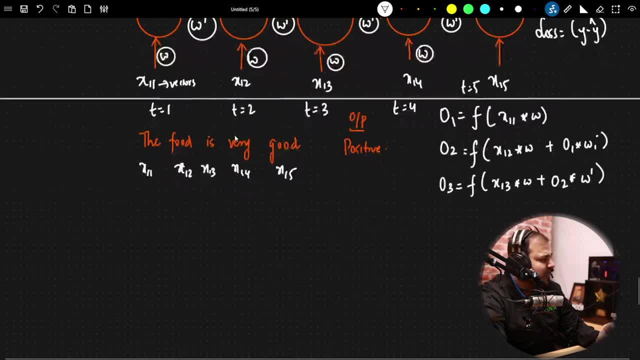 seeing a lot of practical sessions also. i really want to cover each and every bit so that you understand things right. so please make sure that you subscribe krishnak hindi channel. i hope how many of you have subscribed krishnak hindi channel? can you give me a quick yes if you have subscribed? 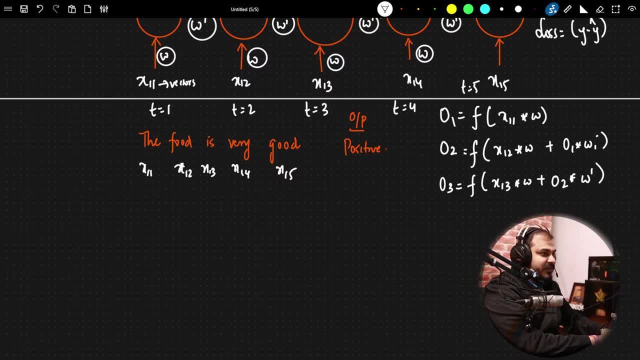 yes or no. if you have not, please do it, because i'm also coming with a lot of hindi videos, right? so i'm also coming up with a lot of hindi videos, right? so please make sure that you do that, because, again, i require your support to do anything in life, uh, so that i will be able to provide and. 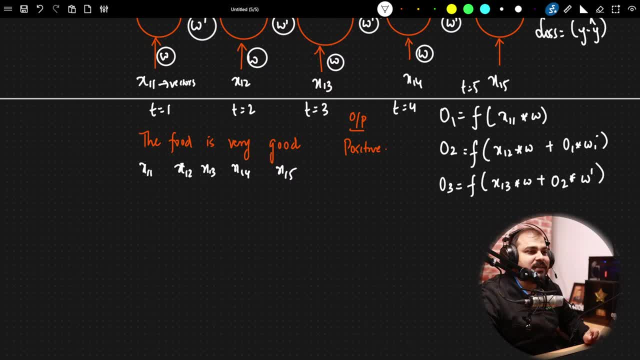 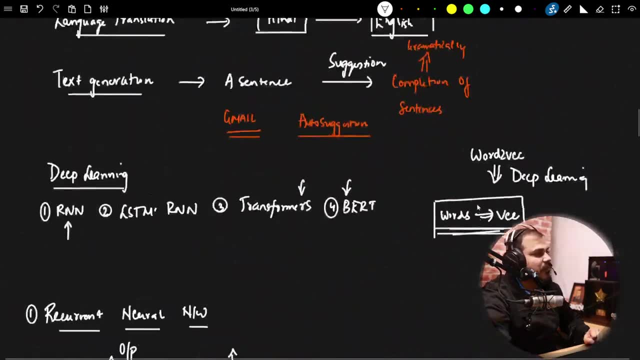 anything. if you really want to support my channel, join the membership guys. it will be quite important for me so that i'll be able to, you know, do all this kind of live sessions for everyone, provide you more information. this is a request. try to support by joining memberships. try to support. 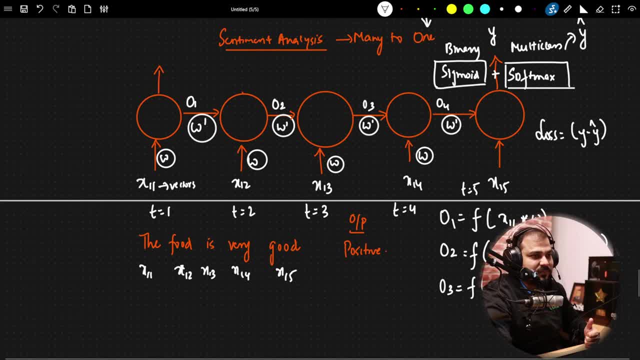 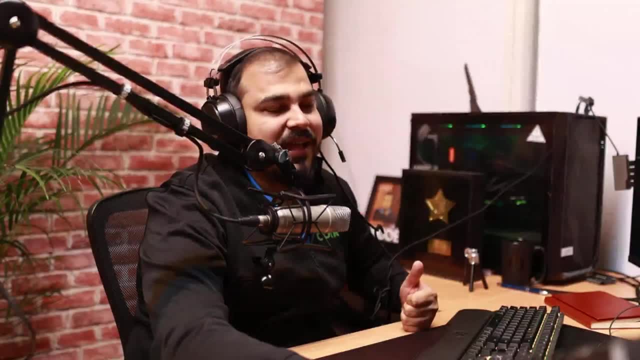 by giving some super thanks. anything that would be amazing, right, so i'll see you in the next video, right? so, um, yeah, this was it from my side. i hope you like this session. please keep on supporting, keep on, uh, sharing your knowledge. never give up you if you find even some difficult things. 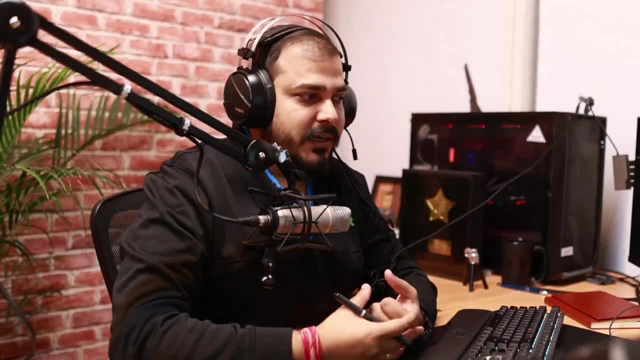 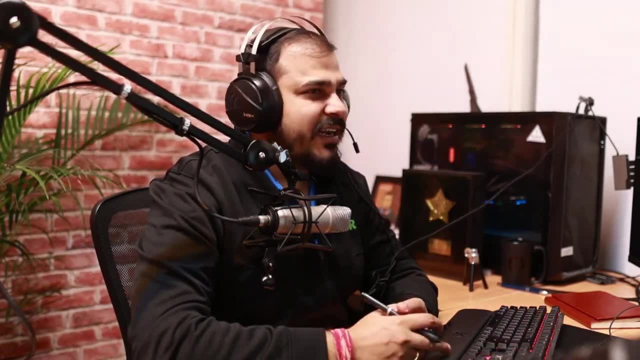 also make sure that you know: try to not quit and try to learn for it. uh, this is super important. from tomorrow, we'll also be having quizzes. uh, today i did not get time because saturday, sunday, you know- there was jobathon. more than you know, 80 percent, 80 people, you know. 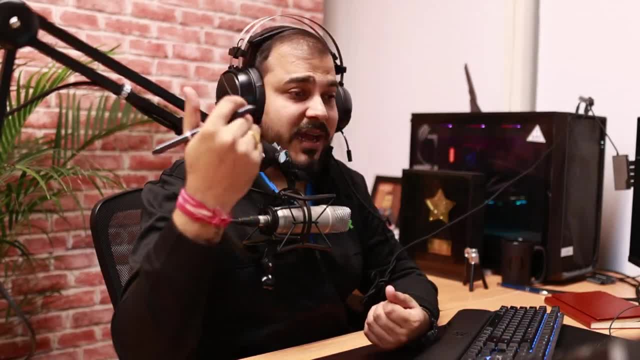 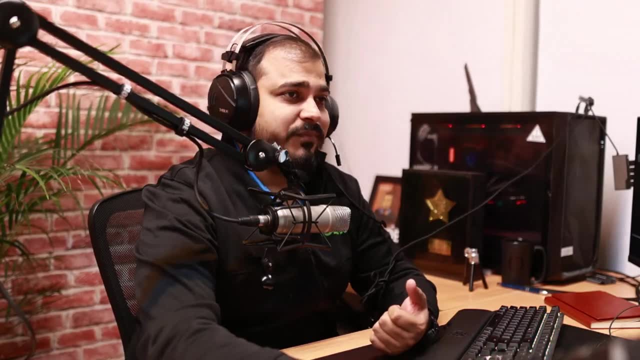 like around 10 to 15 got hired in iron neuron and there were some people who got hired in new sigma and there's still interview processes going on. in the future we- whatever courses that we come up with- will be super important. okay, one quick announcement that we have done, guys. this is super, super. 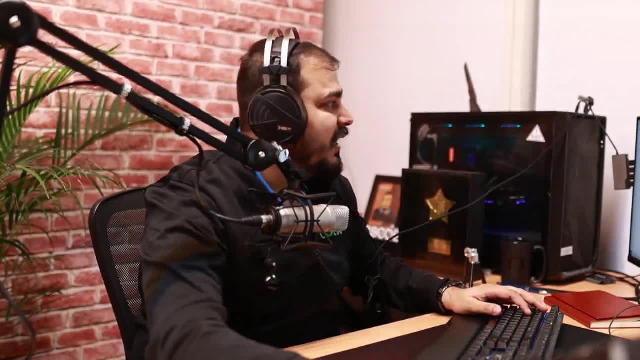 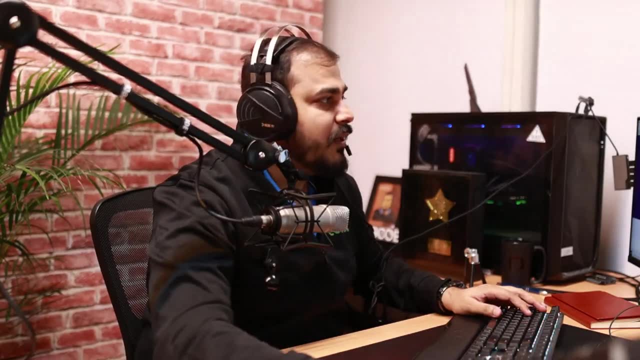 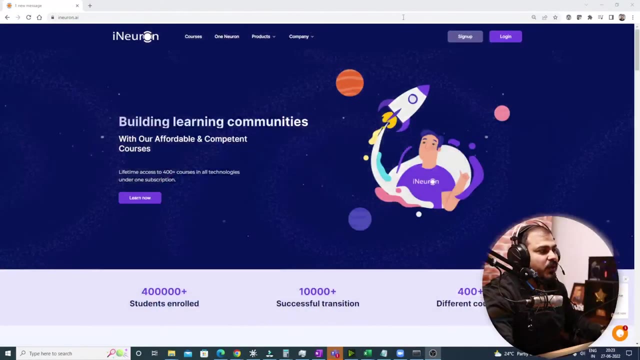 important for everyone. i really want to make this announcement quickly so that you don't miss this opportunity. now, any courses that comes up in iron neuron, you will be able to access it through tech neuron. okay, amazing. let me just announce it quickly. so here you can see that any courses now, any courses that 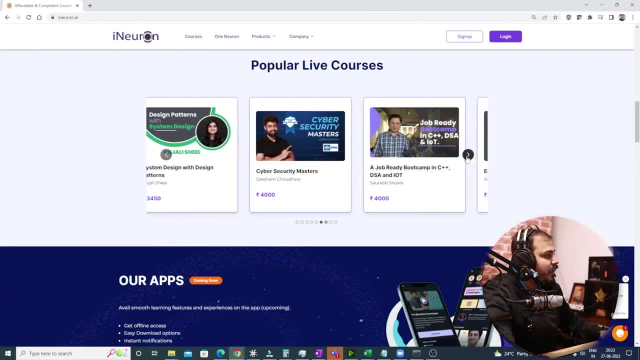 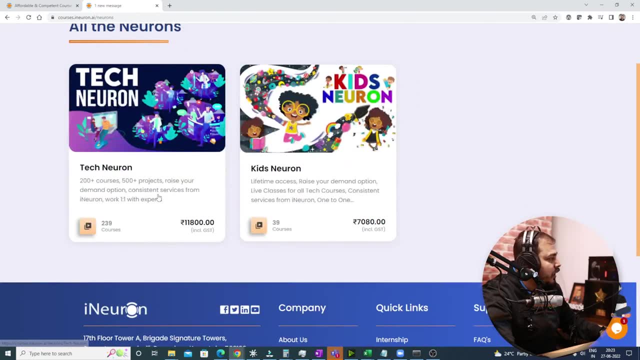 are going to come up. see, all these courses that are going to come up right, will be available in tech neuron. okay, it will be available in tech neuron. that is one neuron, uh, so here any live courses, so all the live courses, you'll be able to attend it. so suppose, if you log in over here, 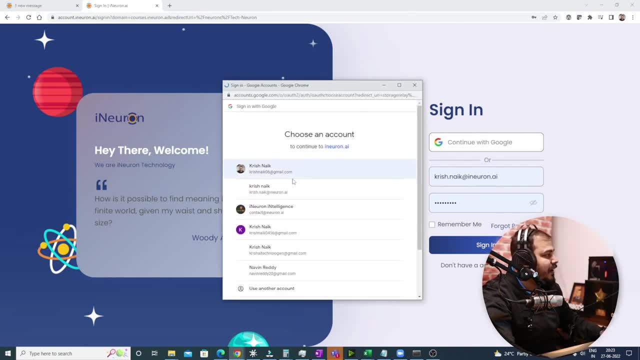 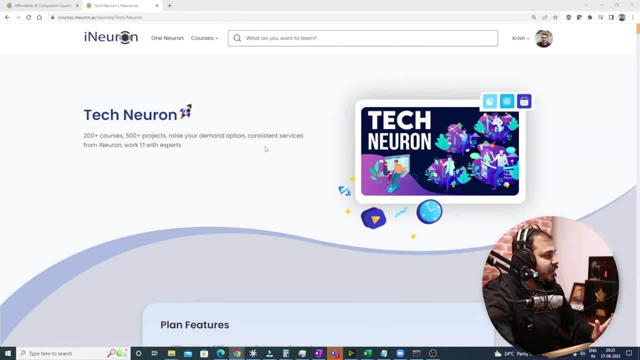 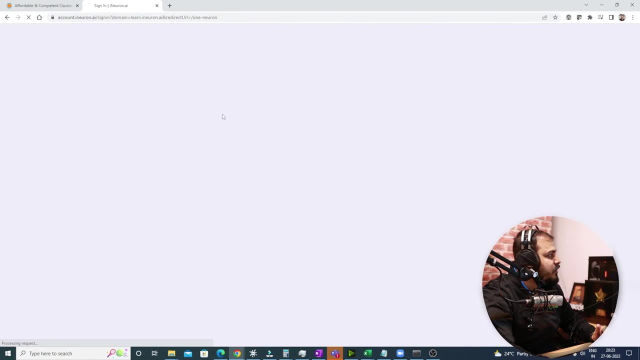 and if you take it, you will be probably able to attend all the live courses. the subscription plan is two years, okay, so you can go ahead and take it. see, just by paying somewhere around ten thousand rupees. this is including gst. if you go to one neuron here, you'll be able to see so many things. 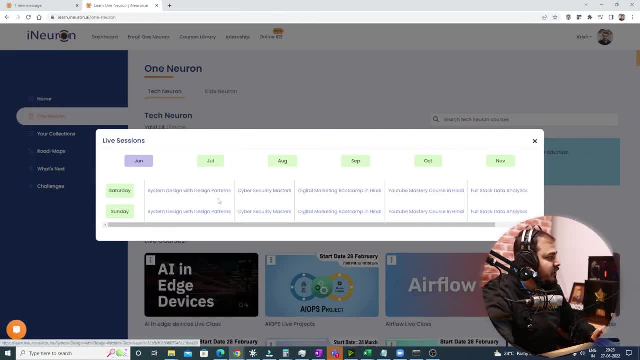 see this. so here, all these live sessions like system design that are going to happen in saturday and sunday. digital marketing, youtube mastery, full stack data analytics- in the future you will be having uh, enterprise java job ready boot camp in c plus plus dsa and iot. 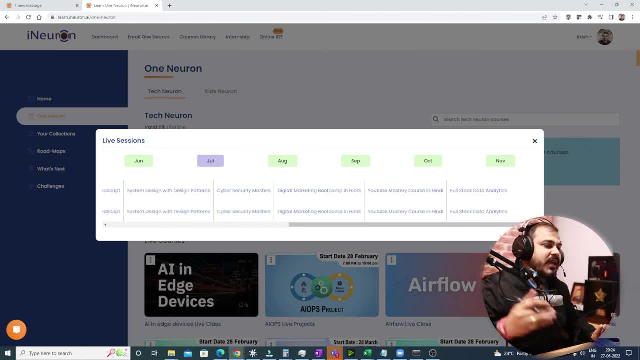 everything will be available to you, or every high, every available courses that are going to come up live in i neuron, that are also being available in tech neuron. so if you have already not used it, please go ahead. if you want additional code, use krish 10. you'll get 10 discount. okay, see, i know. 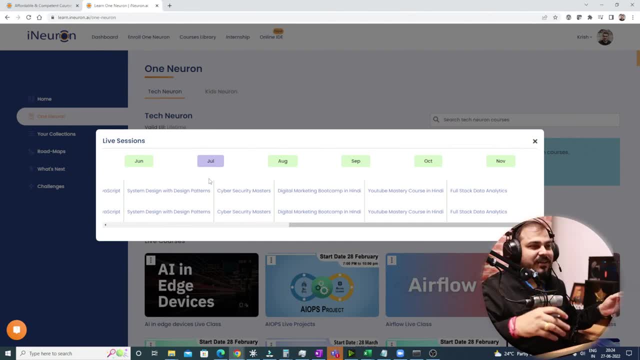 you may be saying krish about manga. this is very costly, guys, just understand, because we for the next two years, whatever courses that is going to come up, all will be available for uh in your dashboard and you'll be able to uh get the all the live. 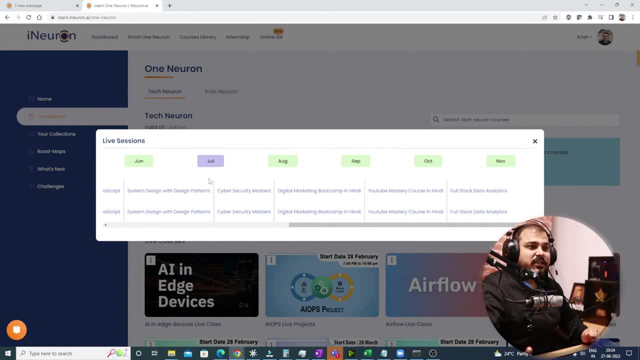 sessions from the next two years that are going to come, and every month we at least launch two to three courses also. so please make sure that you go ahead, take it up, you know, without wasting any time, and all the upcoming courses. anything right now: full stack data analytics- i am taking fhds.